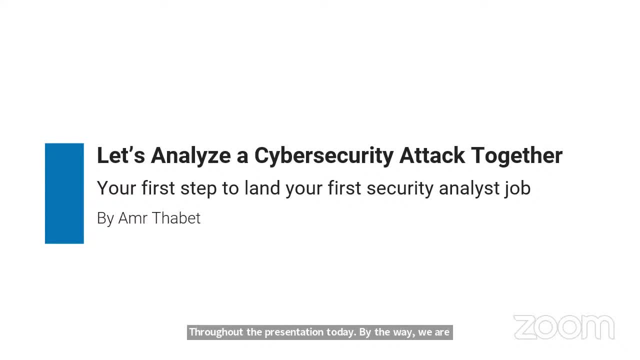 By the way, we are going also live on YouTube as well, So hopefully that's okay for you guys as well. We'll be on YouTube and LinkedIn. What are the must-know tools in cybersecurity to help get a job quickly? That is a very good question. 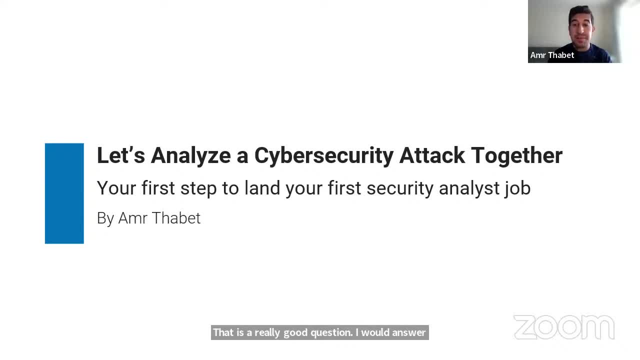 I would answer. that is, of course, Wireshark, which we're going to talk about today, but also Splunk or any SIEM tool. Most of SIEM tools are kind of the same- Elasticsearch or Splunk or- but if you're going to learn multiple ones, then learn Splunk, and maybe another one is Microsoft Sentinel. 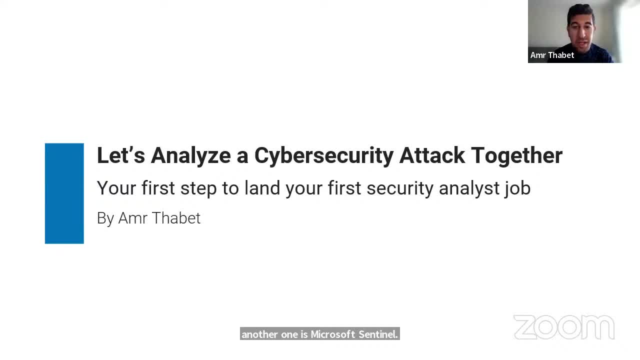 It's a really great tool as well. So, yeah, that, hopefully that answers your question, And we're going to go also deeper. We're going to talk a little bit more about that, Cool. Any other questions? We have now 35 people in the Zoom meeting. 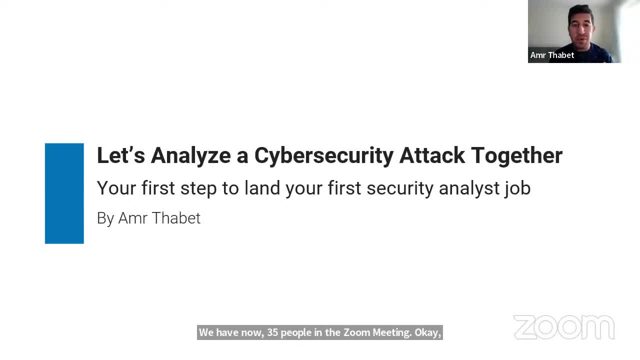 Okay, Let's get started, And there are people who can join us throughout the time. So first, my name is Amr Thabit. If you don't know me, I'm Amr Thabit. If you don't know me, I have been a malware analyst in Symantec before. 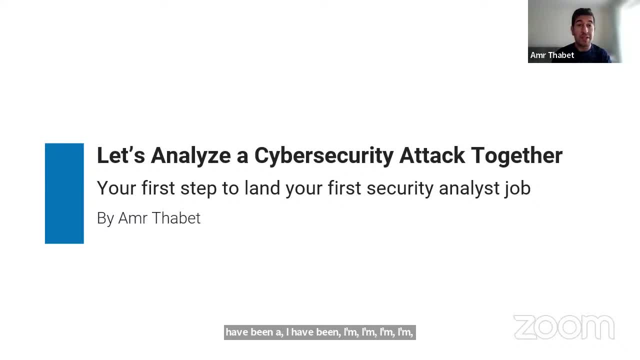 I have been a reverse engineer in Tenable and I'm the author of Mastering Malware Analysis and now I'm the founder of Maltrack. And in Maltrack we do provide different trainings and help people through building their career in cybersecurity and, as well, helping companies to do the daily SOC tasks and so on and instant response and so on. 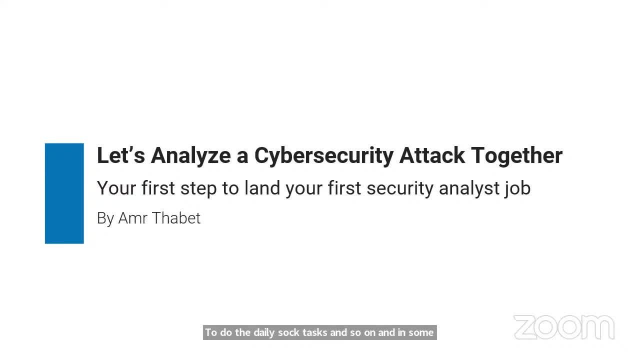 So let's get started And let's analyze a cybersecurity attack together. Give me a second, Just letting everybody in. So today we will focus on two things: how you can build a career in cybersecurity. That's one important part, And the second part is: I am quite sick. 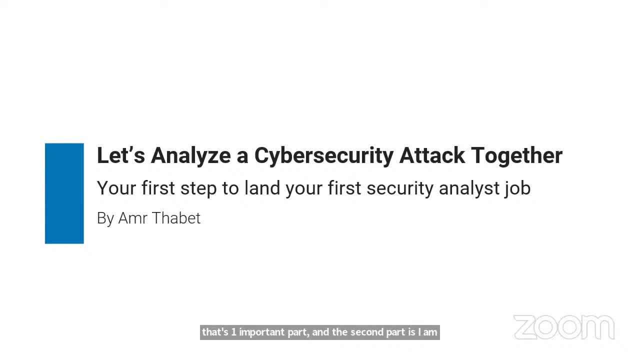 So I'm, you know, taking It easy. a little bit Sorry for all the breaks beforehand, But this is just a part, and certifications can help me to be a cybersecurity in the cybersecurity arc. We're going to talk about the certifications today, for sure, throughout the presentation. 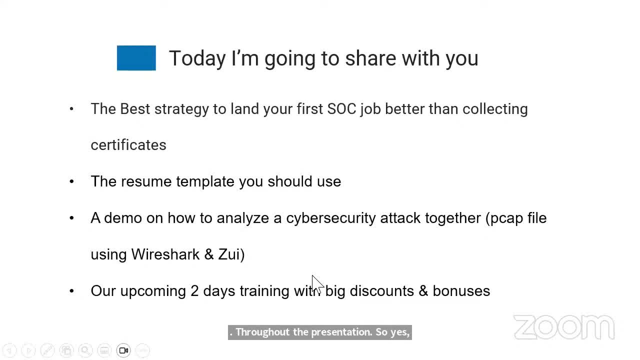 So, yes, we're going to focus on that as well. So today, what I'm going to share with you guys is the best strategy to learn your first SOC job And and like better than collecting certifications. That's why I'm going to talk about certifications today and the resume template that you should have to showcase your skills if you are not going to have certifications or work experience beforehand. 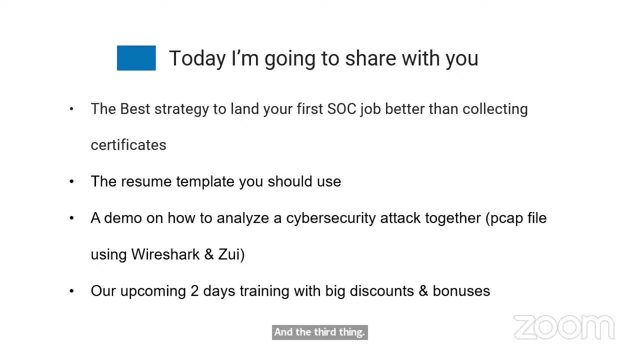 And the third thing is we're going to have a demo about how to analyze malware in Wireshark, or a backup file actually in Wireshark, And so we we're going to focus on analyzing the network attacks today And later on we have a training in 20th of April. 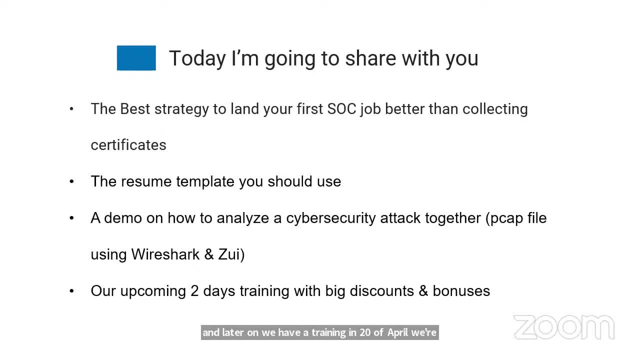 We're going to talk about it. That will be covering, you know, analyzing the attacks through also the other domains, like through Splunk or through different other other areas of the attack, like the host's behavior, and so So far, so good. Thumbs up if it's good. 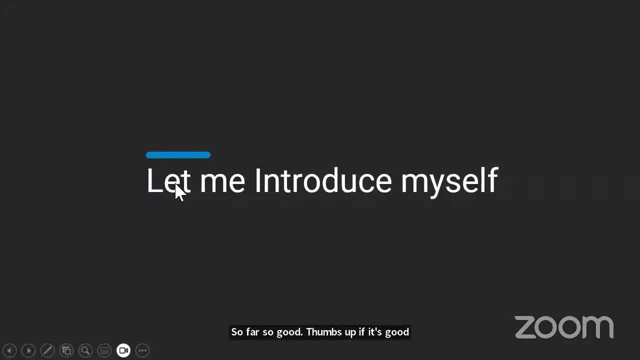 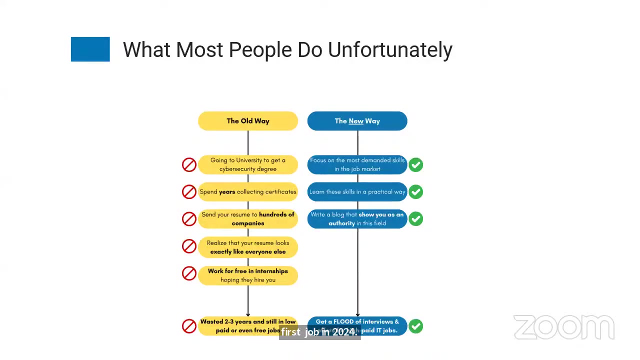 So I have introduced myself. So let's talk about the best strategies to learn a job, to learn your first SOC job in 2024.. If you are not already in SOC- which I see some of you guys already in SOC, but if you're not in, there's two ways you can go about it. 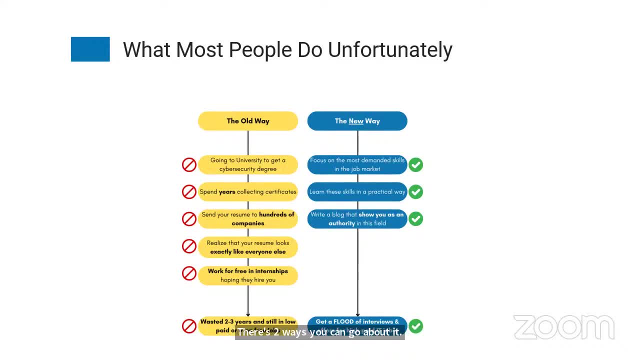 The first way is to get into, you know, to get into university. get into, let's say, Wireshark. No, you can't do Wireshark, But you can get a degree and probably get some certifications, Let's say CH or ACP. 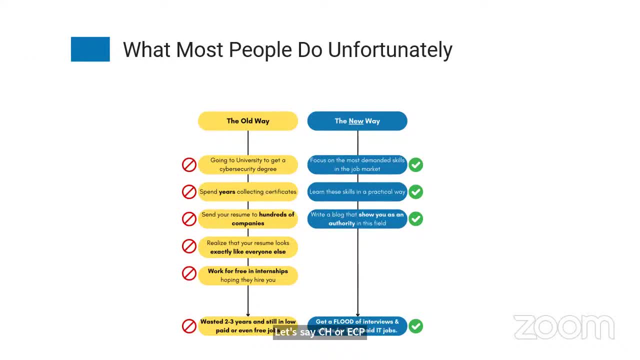 There's, you know there's so many other certifications: Security Plus from a, a plus CCNA, all of these certifications. So you start collecting one certification after another after another. deployment happens Once you finish. all of that is that you have a resume that is similar to almost everyone in the whole cyber security world. 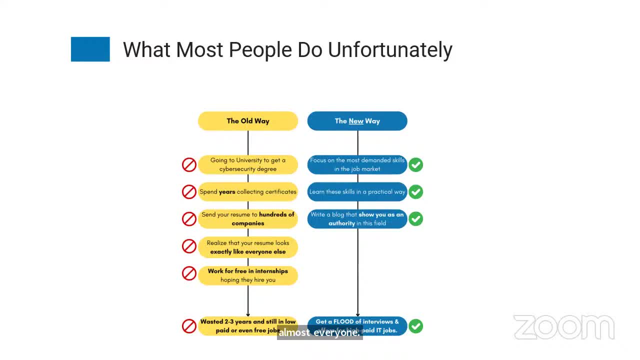 You know it depends security field, like the. you are applying for a job, you have a degree, maybe computer science or something related to cyber security, and you also have um, and you also have the same in terms of your um, in terms of your certifications. you have the ch and security plus and all of the. 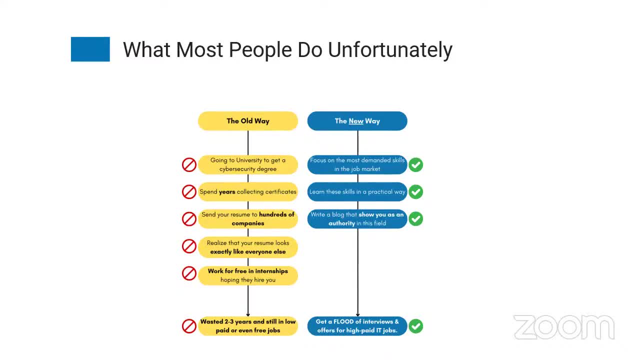 certifications that everybody also has. so you apply for a job and you see many of the candidates have the exact same resume. it's like a copy paste of your resume. so, um, what to do in this case? uh, i'm gonna, um, what's the name of the tool from that sentinel? yes, uh, so so what to do in this case? 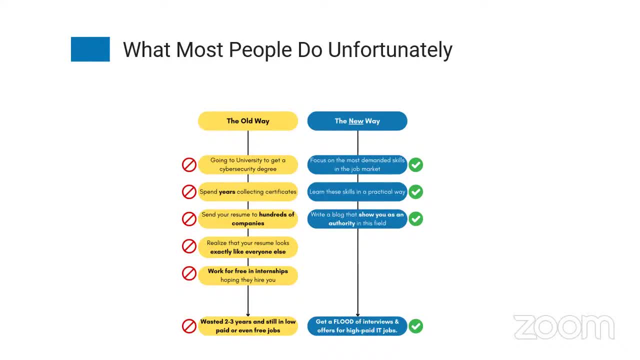 well, you will have to look for jobs and probably you will start with internships where you are not paid to hopefully compensate for the fact that you don't have the certifications. so you start to look for jobs and you start to look for jobs, and you start to look for jobs and you start to 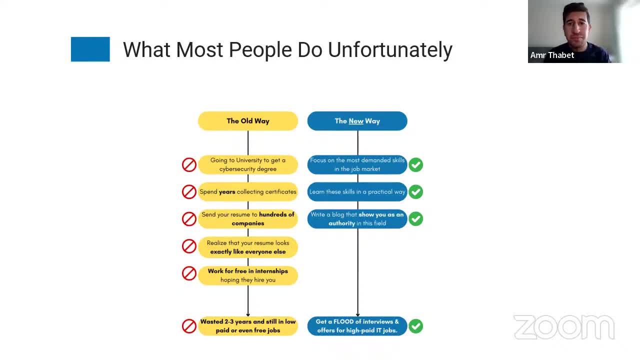 go with. okay, let me apply for the job first, for unpaid jobs. hopefully i can get the work experience and from there i can probably get you know liked by the company and maybe they're gonna hire me a bit later. if not, i am gonna have the work experience so i can use it to get a real job. 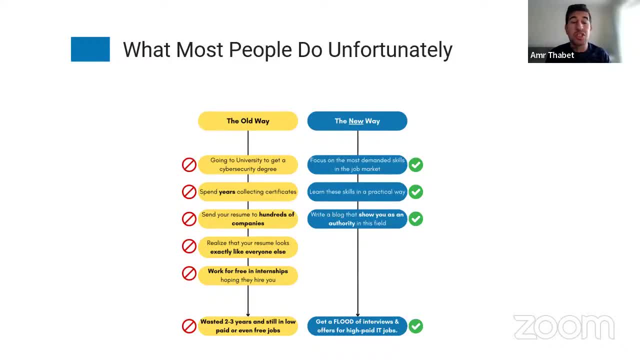 and then you continue in this process. you're going to the first internship maybe three six months, then the next one three six months, and with the promise: oh, you're going to be hired, they're going to be promoted after six months, and then you spend maybe one, two years in either. 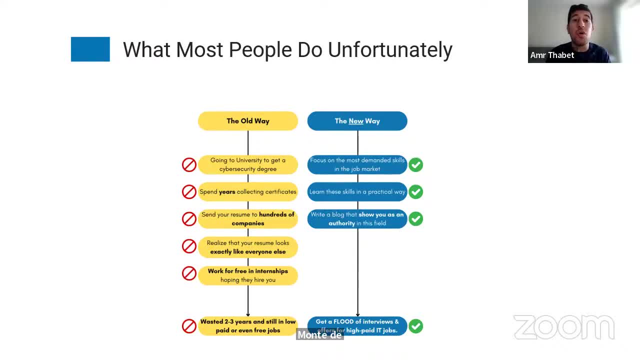 low paid job or or unpaid internships, hoping that they're gonna finally promote you into a real good job, right, and the problem is that this whole process takes long, long time between degree certifications, internships and, hopefully, a good job. until you reach that point, it's like 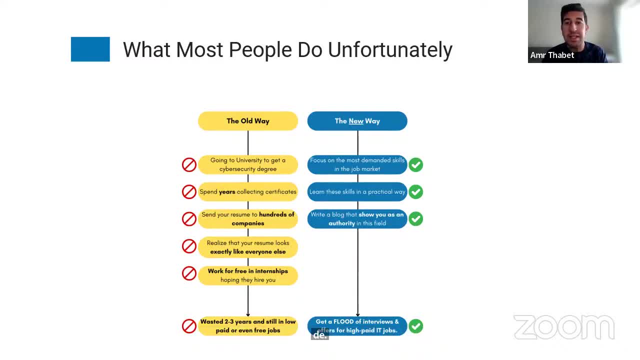 like last time. we were like somebody was saying: it's around, takes five years. that's the problem with this process. the process that i followed was a little bit different, so for me, i focused on learning the skills first. i didn't have, uh sorry, one break, um. 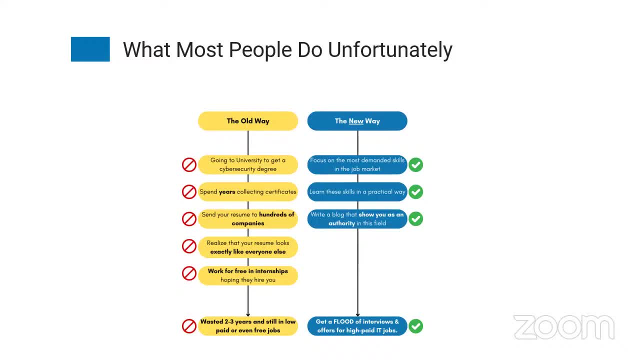 i focused on learning first how to do the day, day-to-day job, let's say, analyzing a malware, um, you know, looking through logs and doing all of the different things related to, like wireshark, analyzing attacks. i started learning the practical skill and my focus was at that time like: what are the most needed skills? what is the people talking? 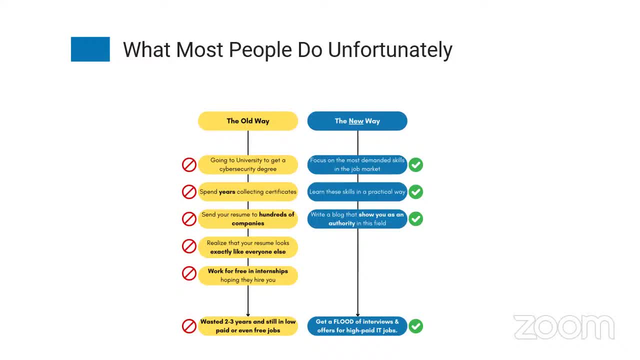 what are the people talking about right now? like if i would talk to um. you know an analyst, a cybersecurity analyst. what he is going to be talking about today, what's going to be the biggest um problem he's going to have right now? right, that is the first question i do have, and 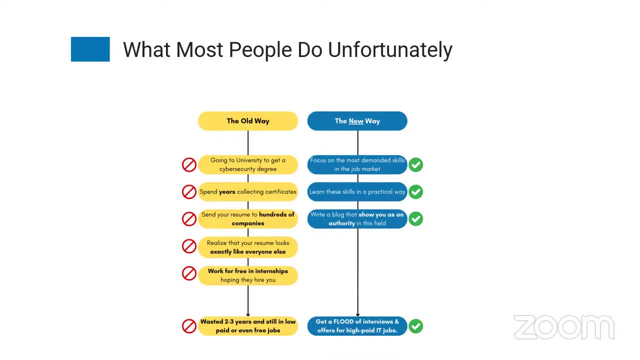 the second question is okay, if, if i can learn these skills and understand it practically, how i can show myself. i went into the, the degree route, into the certification route and then i ended up that i found they are very expensive. they are there's far too many certifications. i started. 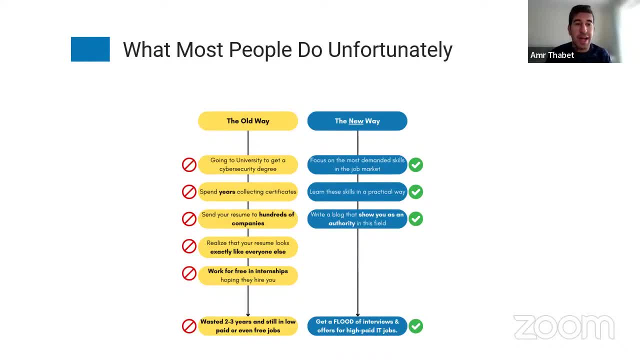 with the red hat. it didn't do very well with me. it's like: okay, i learned red hat, now i have to pay a lot to get the certification, and then i have another three, four certifications and i will be. i will cost me thousands of dollars and after all of that i don't know if i'm gonna get a job. 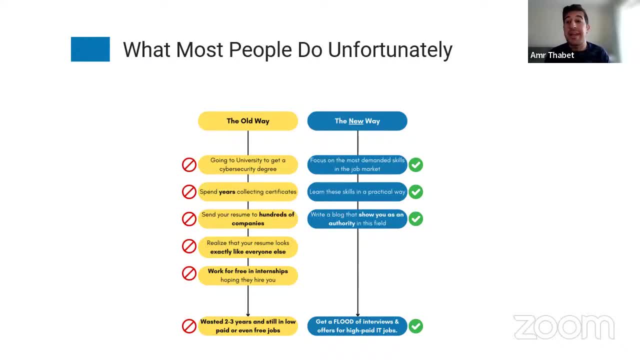 i'll be like everyone else. so i didn't go this route and i created a small blog and i started posting different analysis that i had and then in just a few months after that i was able to get in like, let's say, in six months time i was able to get five different job offers. 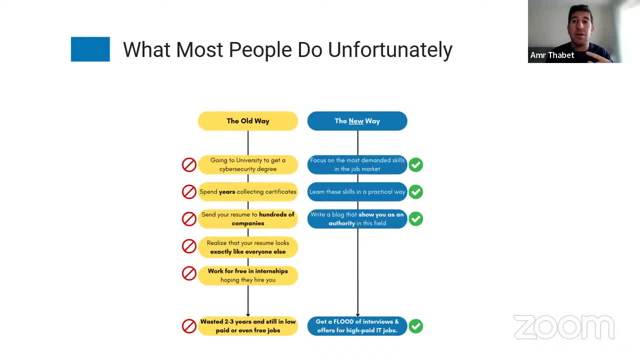 one from egypt, egypt, one from qatar. one uh online was a company called komodo. it's an antivirus company. i also worked in um in another uh also got another two offers, one from uk and one from one from italy. so i got five different job offers in like six months time, just based on. 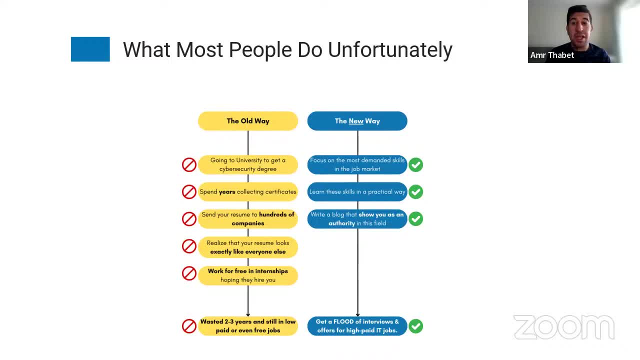 and based on just one or two reports that i have done so, i discovered that it's really not about the certifications at all. it's not. that's not what the companies are looking for. and now when i started working in the field and i'm meeting hiring managers and recruiters and so 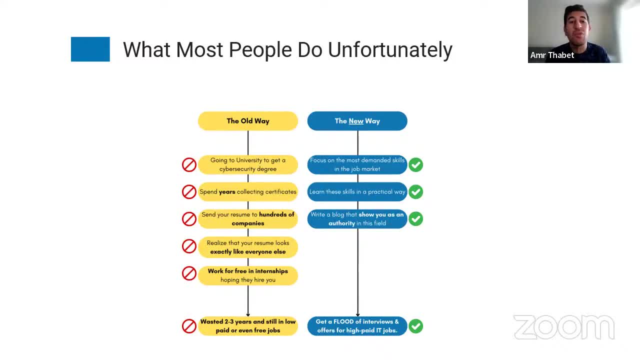 on. they are not looking for that. they are looking for someone who they can plug in the team and he can do the job. that's all they are looking for, right, and that is basically it. that's that's all what they want. so how you can prove you are that person right, how you can prove you: 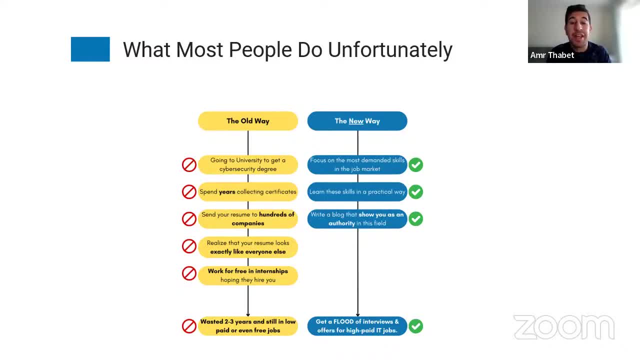 are the person who has the practical skills and certifications right now. nowadays doesn't prove anything anymore because a lot of people can basically pass the certification just by having paying somebody to take the certification for them. many people who many of the certifications are like are, kinda like you know, exams, like you know. 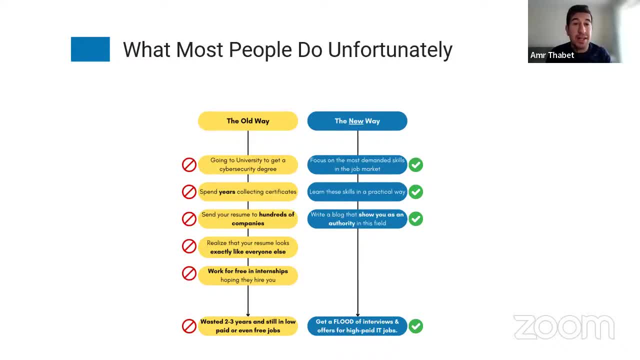 multiple choice and theory exams, so they are practically useless. some certifications that are practical, like OSP, but you see that most of the work, most of the work that you have, that you that you are learning through the training, is actually not related like it's not related to the real attacks that's happening nowadays, like, let's say, let's take OSP for. 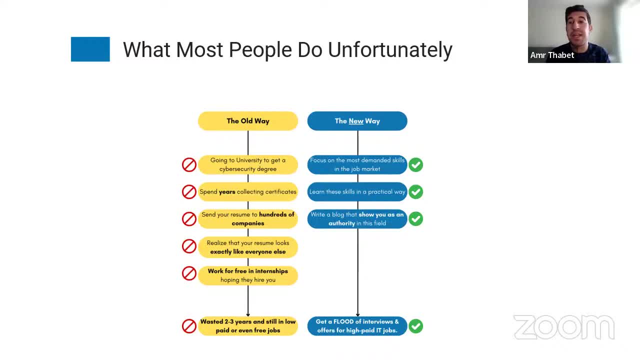 example, most of the things you learn through OSP, like you know scanning different ports and OS fingerprinting and finding these. you know exploits and use metasploit and use exploit DB. that is like 90% of the attacks. don't look like that- 90% of them, so most of the real 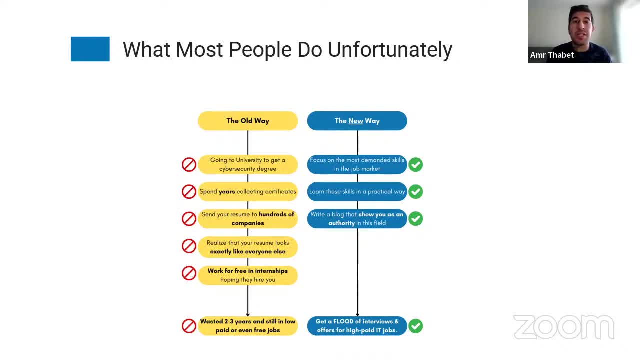 attacks that I see in the world are using phishing, are using malware, are, you know, are sending, are using active directory weaknesses and they are focusing on the real attacks on the weakest element in the organization, which is people. so they are not really focusing on, you know, on scanning ports and finding servers and trying to hack servers. it might. 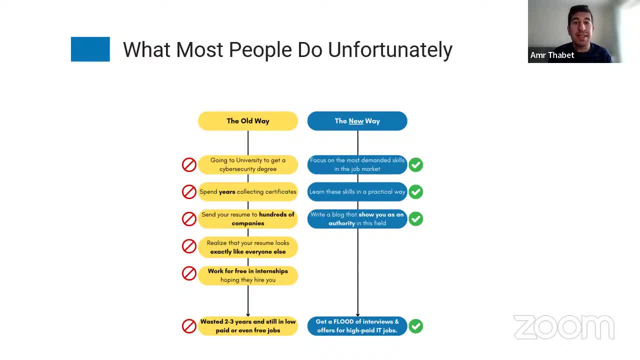 work in some attacks. some attacks might use these techniques, but the 90% of them won't use these techniques. so which is the better way? I should follow that process of you know of courses that are basically kind of phishing. so I think, I think it's a good question. 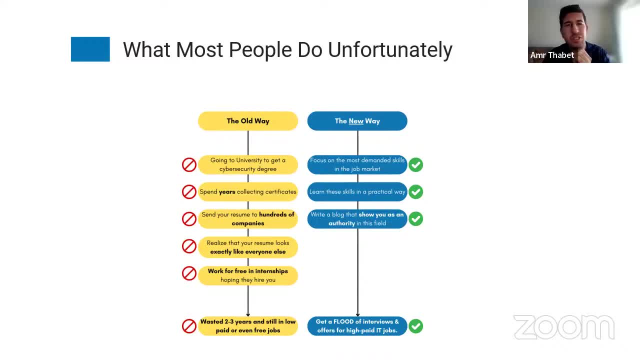 No, I think it's a good question: the old fashioned and take the certification and spend so much time and money trying to get the certification, and then I'm like everyone else and I still can do my day to day job and I don't have something in the proofs that I'm unique and take ages to do this part, or 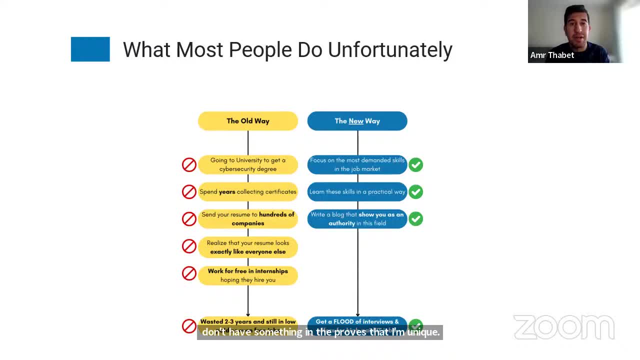 learn the practical skills that are actually needed in the market. just learn the skills that you, the things you're going to do in your day to day job, and focus on learning that. Then you know, apply these skills in a, in a in one analysis report or multiple. 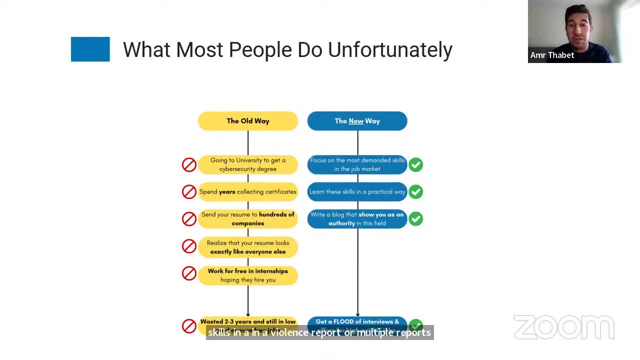 reports. multiple blogs share these blogs in your LinkedIn, in your LinkedIn profile, in your resume, and, and with that you can able to finally land your first job. Does that make sense for you guys? Thumbs up. if it makes sense, write me in the chat Like. 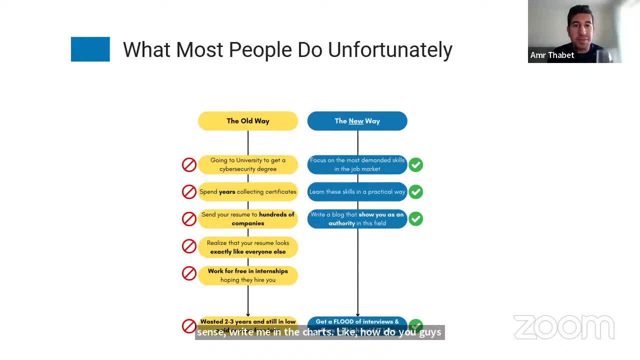 how do you guys think about what I'm talking about? Do you guys feel the same problems? Yes, Thumbs up. And, by the way, we are also live on uh, on YouTube and everywhere. So if you guys see you or you hear me, please write the chat as well. Uh, I see, um, I see. 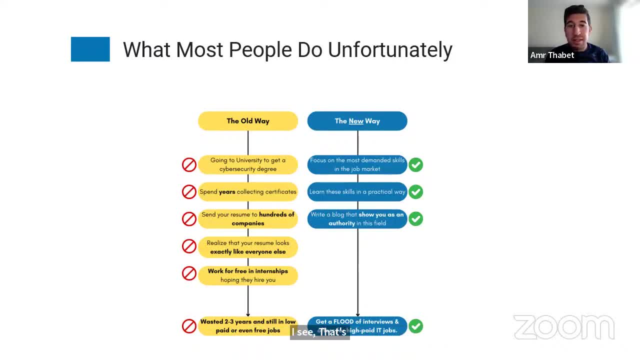 a lot of people who are interested in blog posts, but writing an interesting blog post is hard, isn't it? It doesn't need to be. it doesn't need to be very interesting either, which is a really good thing. You know, you don't need to have a very interesting blog. 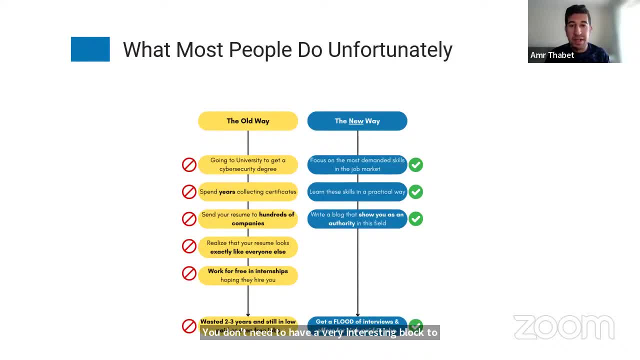 to really become, uh, to become successful in writing blogs Like my blog posts, like, if I show you in my first blog posts, they were really, really crap And I was using WordPress or blogger back then. No, not WordPress, blogger, which is, uh, an old app. 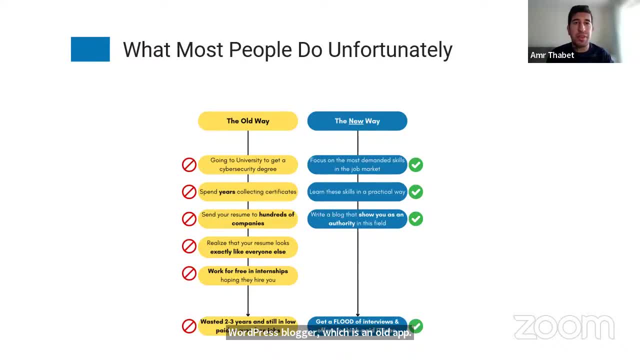 Um, and I had like a really terrible theme that was completely broken and I was writing different blogs. The English was barely readable, but at the same time I had good analysis. I have done some projects and that was all needed, but there is a difference here. There's. 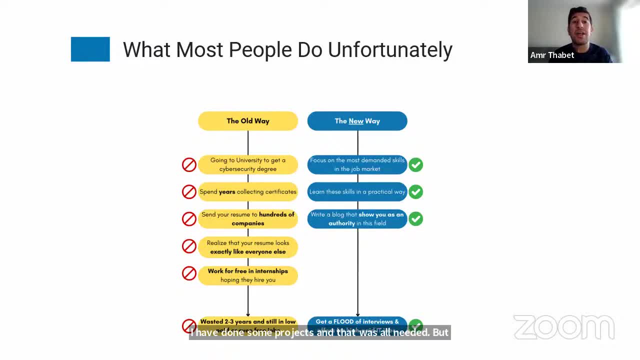 a difference between writing a blog generally or writing a blog that looks that you are a professional in what you're doing. That is the most important. So, um, so, that is basically what we try to do. That's what we try to do, to try to make something that actually, um, you know, to share something. 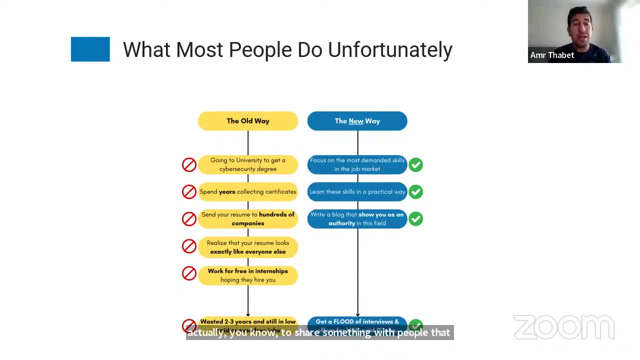 with people that is actually um, um sorry, I uh run out of thoughts, uh to to write something that looks professional, that looks like Um one second guys, Um, Um one second. So the whole idea is to write something that is uh, that is looking professional, that. 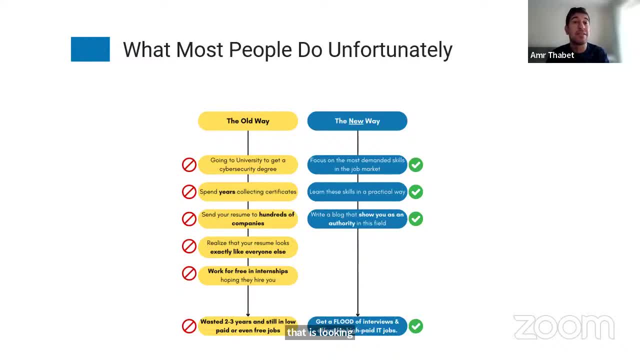 people can see that it's like, wow, this is a really great thing that I can do. It's like: is really this guy really understands what he's talking about? that is the most important, um, and that's what we try to do in different blocks. at the beginning, i didn't know how to write a really 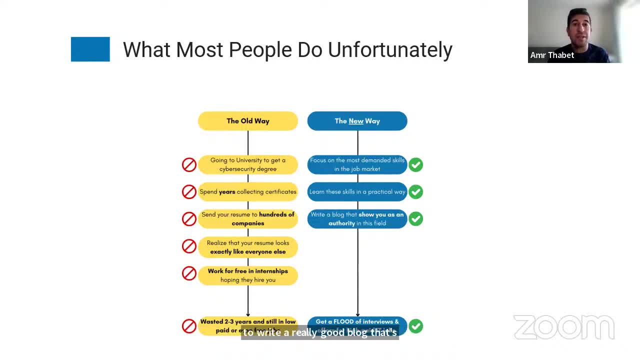 good block but despite that still got me results and still was able to analyze different attacks. but i was looking also on different other reports while i'm writing a report about one thing so i'm writing about. i was writing about stuxnet malware and i was looking at, like how semantic wrote an 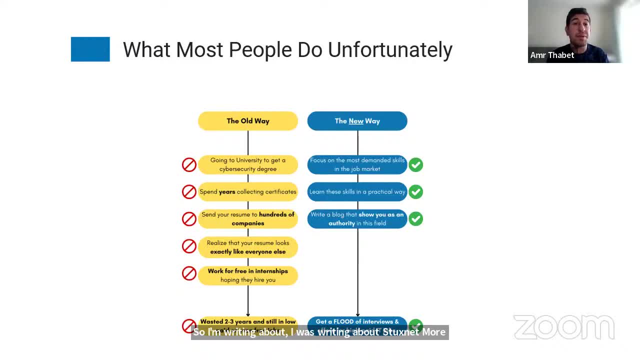 article about it, how esat wrote an article about it. at that time they were posting a lot of articles about it and from there i have learned the process and i followed kind of the process and now i can write way more professional articles and that's what we help our students with. but back then i 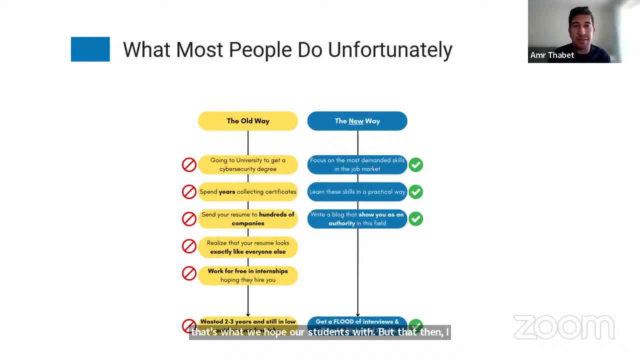 i wasn't really good at it, but i was imitating the others. if it makes sense, does that make sense to you guys? um, so i don't know what kind of projects i should do to be able to do that and to become a better network security engineer. we're going to talk about that, let's um, we're. 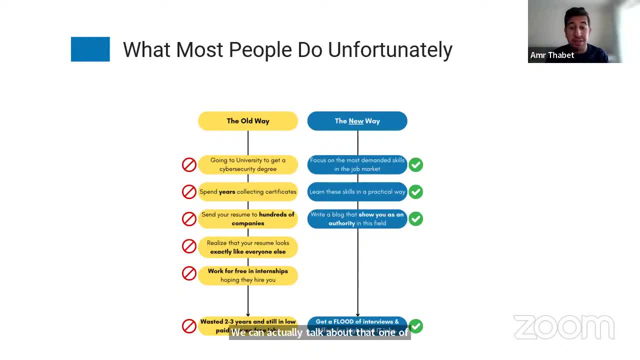 going to actually talk about that. one of the projects we're going to do is the analysis. what you're going to do today. um, so should i write a blog in medium rather than writing on my own site? there's no difference. um, the well, medium has more exposure. but that's not the main point. the main 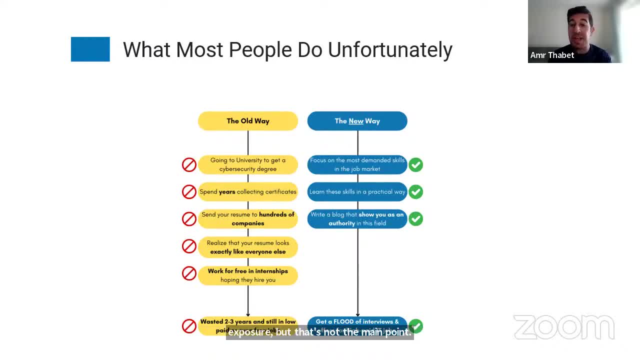 point is to be actually share that on your link, then on your resume, and we're going to look at your, uh, your resume really soon. so, uh, what the lady is saying, that's partially true. yes, the higher the interaction on a platform like linkedin with a good, helpful videos ends up with good visibility. so, yes, uh, that ends up with a really 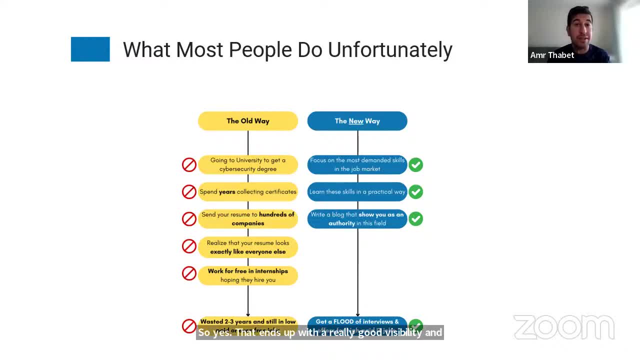 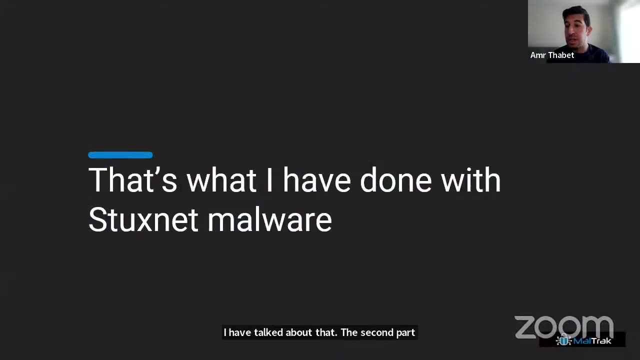 good visibility and, as well, if it's your own work, not just sharing random stuff, is is even better to show that you know what you are talking about. but the second part from there is your um, i have talked about that uh. the second part is your uh, is your resume. we're going to. 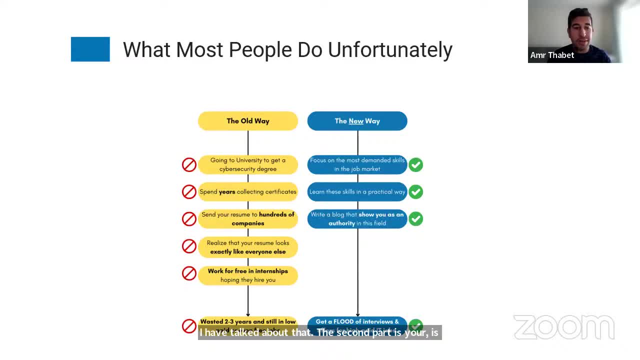 talk about the resume in a in a minute. i will get into that in the slides a bit later. but a big part is also your resume and we're going to, we're going to share with you how you can show that in your resume really, really well. but before we go into that, we're going to focus on what's exactly the 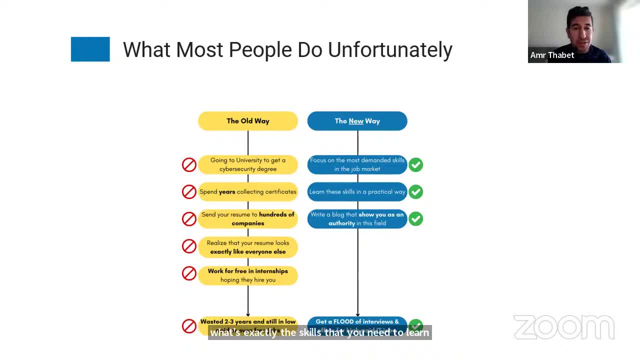 skills that you need to learn? um, does that make sense for you guys? any question you have thumbs up. make sense, write questions in the chat um thumbs up. are you guys hearing? are you guys still here or? um? um, sure, yes, perfect. um, cool, cool, cool, cool, okay, let's. uh. so before we go into like how your resume will look like if you follow, 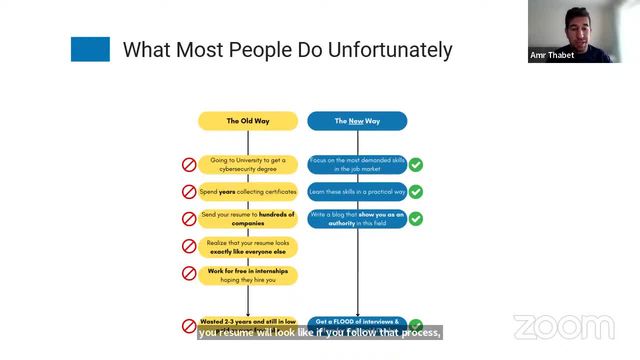 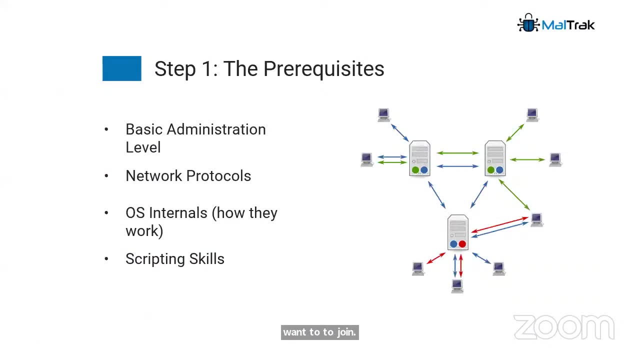 that process. let's focus on what's exactly the skills we need to learn. what's exactly the the skills we need to focus on if we want to uh, to join. so the first thing is the prerequisite, right? uh, the prerequisites is basically um is basically learning the basic administration level. so learn, let's say, linux, how to use linux. 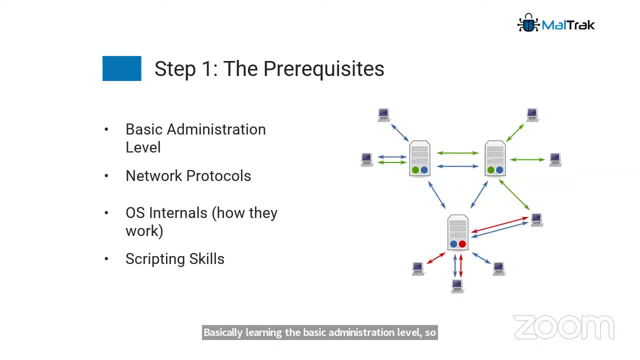 as a user, even not just like, not like. you don't need to be like taking certifications, red hat certifications or something. you just need to know how to use it as a user right, how to install tools, how to install different apps, how to use python, how to use the common prompt, how to delete some. 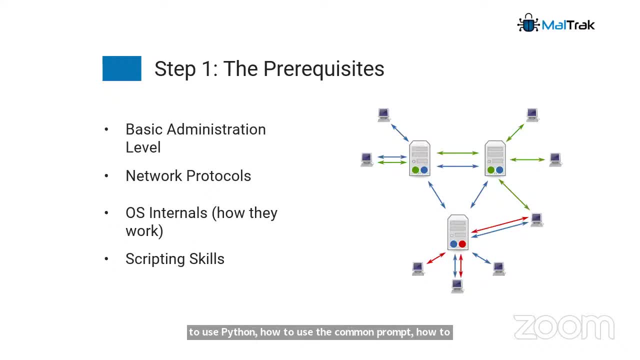 something, how to deal with drivers problems, all of these different things. and the second is network protocols. so how the internet works, that's very important. how the internet works, the bcap files understanding the hdb protocol, dns, tcp, udb, um, ftb, smtb, all of these important. 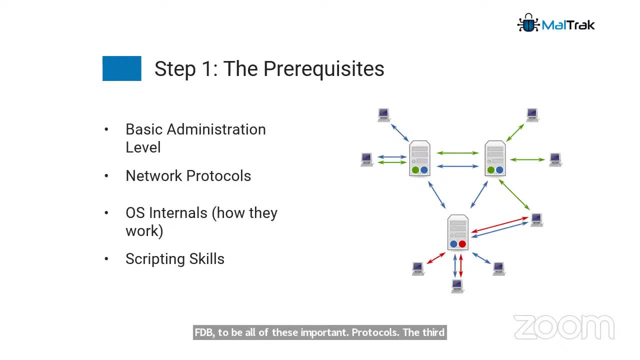 protocols. the third is- which is a bit optional, but you can learn it along the way- is operating system internals. and the operating system internals is really understanding, like, how the system works, uh, how the system works, and, um, like, what are processes, what, what are threads, what are these things? what's the process, thread, um, and how, the, how the system loads, uh, what's. 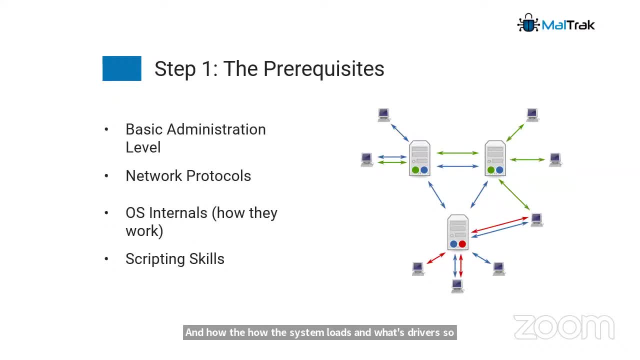 drivers. so what's? apis, windows, apis, all of these different things? you don't have to learn them straight away, but it's going to really really help you along the way when you are learning more, because if you are going to respond to instance, you need to understand, like, how the system works and how he can abuse it. uh, if you need to understand. 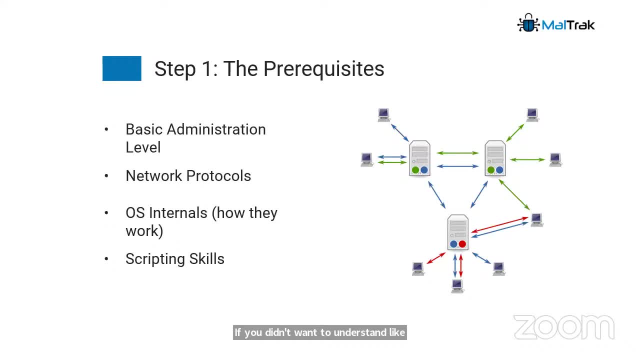 like identity attacks. so it's like: okay, he's collected privilege. what does that mean why he wants to escalate privilege in the first place? what should i do about that? so all of these questions. you need to understand operating systems a bit deeper to be able to- uh, to analyze that. 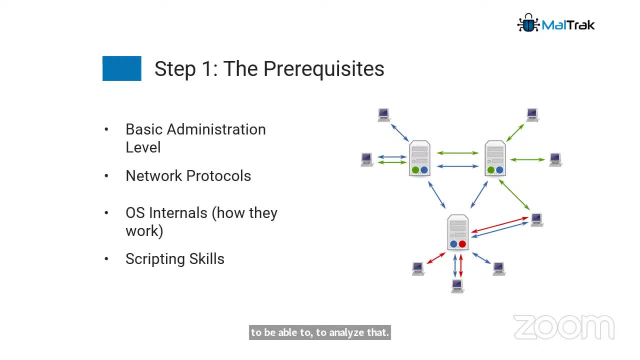 i'm reading also you guys, your chats in youtube and on uh. if you're guys on linkedin, let me know. there's anybody linkedin, let me know. um, the fourth one as uh prerequisites is the scripting skills. it's not a must and it's not programming skills. there's a difference between, like full fledge programming course. 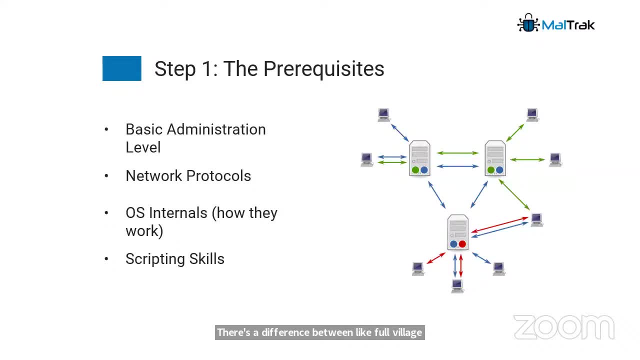 or just writing a small script that is five, ten lines of code or something like that, just to collect some information. it really helps, especially partial, to automate some response parts. again, it's not a must at the beginning to land your first shock job, sock job, but it really is really helping along the line. let me come back to the questions. so 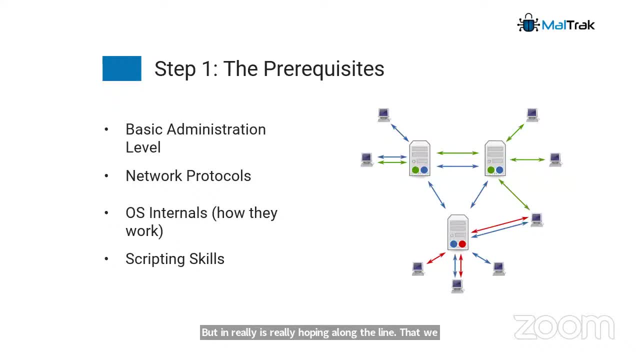 i'm working in security others. in my daily job i use curadar, otrs and other tools. i have been told it's the maximum takes 18 months to learn everything to master my current job. 18 months is good amount of time, but there is two sides of the whole story. 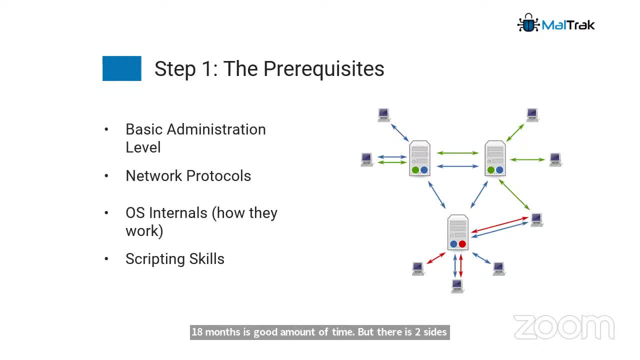 however, i won't know how i can improve my skills. um, so there's two sides. it can take, uh, 18 months, but you also learn some tools that's used specifically in your organizations, like curadar or other stuff. right, there's another company. if you're gonna work another company, they're gonna use something else. 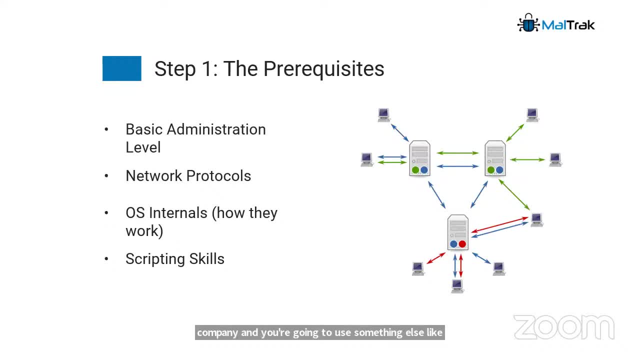 like, let's say, they're gonna use um, they're gonna use splunk or they're gonna use sentinel. so there's a part where learning the actual skill and then there's a part where you are learning the tool, and the tool is not the most important. you need to learn one tool, that's you know. 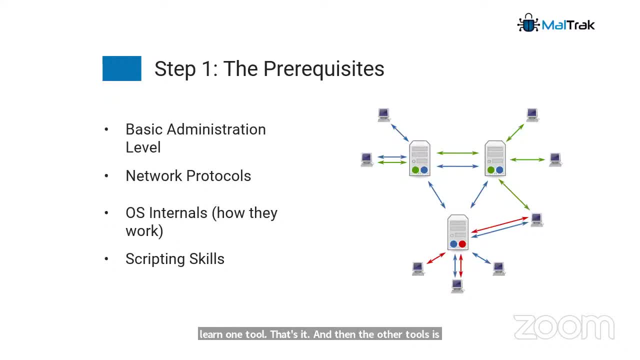 and then the other tools is okay. so, um, how to? i need to learn everything to master my current work. so if you are a security analyst who basically uh, report like see attacks, you just okay, i saw an attack here. let me format the machine and isolate the the attack and that's it. 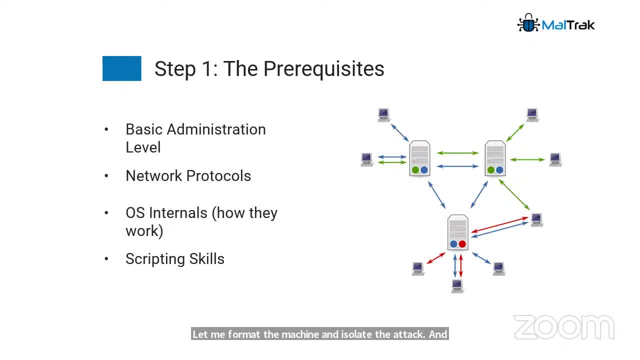 um, i will repeat about the scripting skills. um, if you just like removing, remove the attack and that's it, you need to learn how to investigate the attack further and investigating the attack. so what we're going to do today in the demo, but this is a really really. 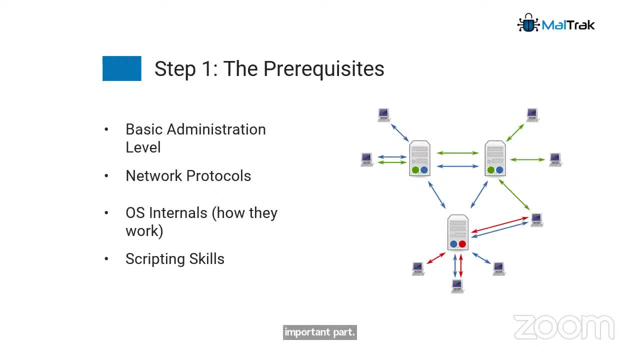 important part in able to investigate the attack, further understand how the attack came here. what are, uh, what, what's exactly the weakness that got him into this uh, into this company, into able to penetrate the, uh, the network, how he, um, how he's created privilege, uh, what's the first infected? 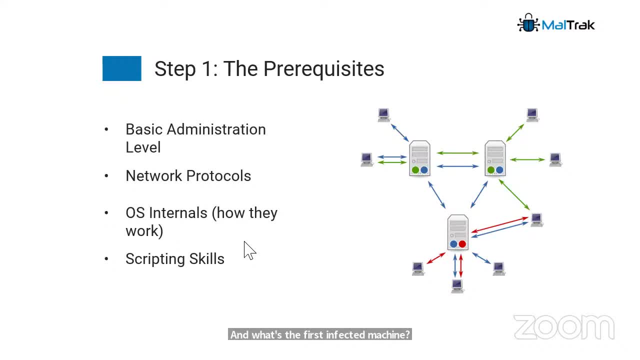 um, how we can protect against this attack in the future. all of the different things. investigate the whole attack is the next question. um, i see rasam saying: uh, can i get a malware announced job in egypt? um, i believe there's issue cert. uh, that is related to malware analysis they have. 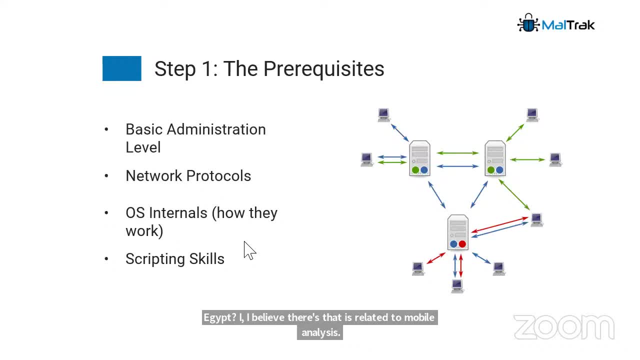 a malware announced department. uh, apart from each insert, i don't know. i haven't been into egypt since long time and i don't really i'm not really aware of the job market there, but i know that ages hurt because i worked in interest as a mother analyst. 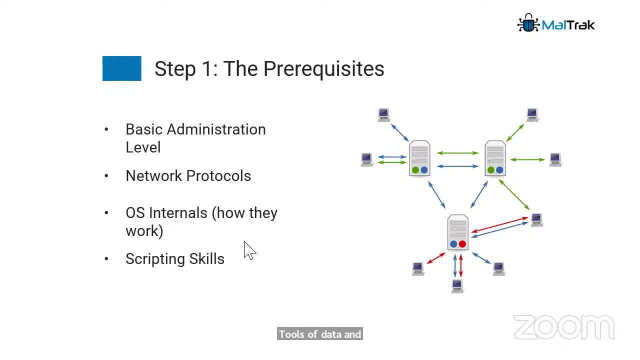 tools updates and changes along the way, you can see, at least try to contribute to a given tool, even if it's a small contribution. yeah, contribution, of course, really really helps a lot, especially if you are- uh, if that shows that you know how these tools work. so again, it's not about the tools, it's about learning how the tools work. 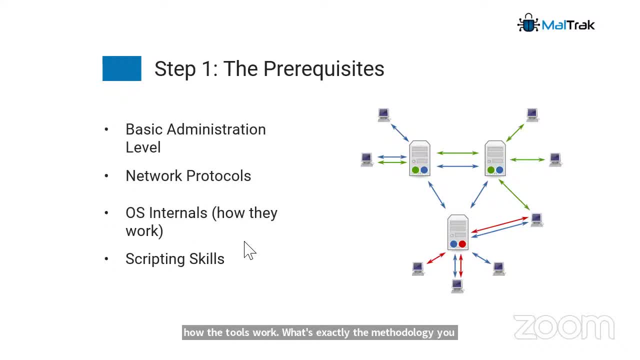 what's exactly the methodology you are using to detect attacks. this is what's really important. so, coming back to the, to the scripting skills: scripting skills: you need to learn scripting skills to just be able to automate some parts of your task. that is the most important. scripting is 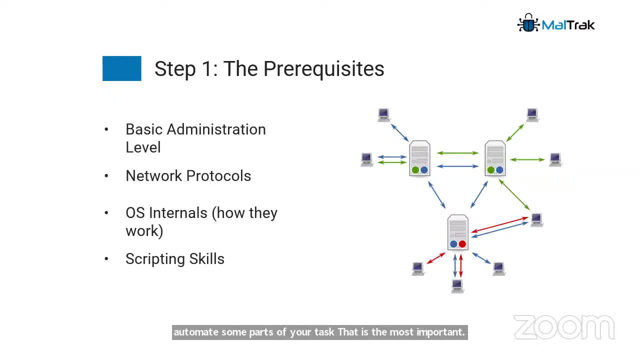 not programming. you can write a script. maybe it's 10 lines of code, maybe 15, 20 lines of code. that is, i think you know most of the sizes, the average, sometimes just one line of code really. but it is the job of it is to automate a lot of process. 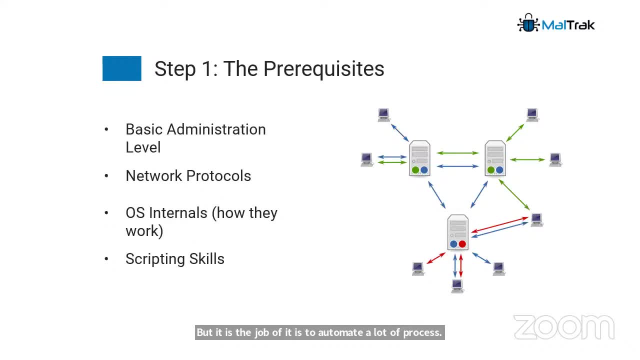 allows you to do what's called partial remoteing, which you can connect to different machines and run commands on these machines, and you can run it on 1000 machines at the same time and get the same output in one big table, and you can save that table into an excel sheet. 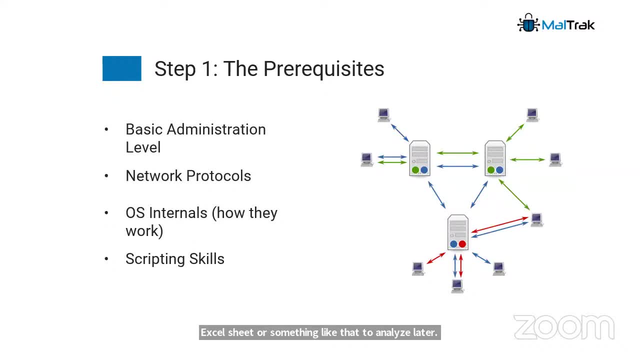 or something like that to analyze later. so that is what you need to be able to do in partial. i can run one command like getting all the updates on all the machine, all the machines, and then all the latest, you know, all the updates. getting them all pulse, they will be able to update, you know. 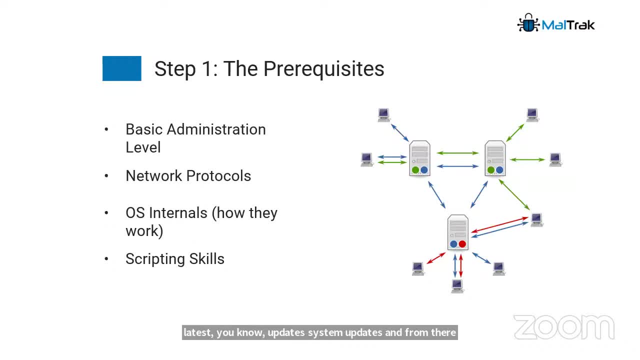 and in order to run all the updates, you need to run it in actually one line of code. i can run it as version 1 of code system updates and from there i can really start to look through the whole list and and see what's. what are the um? what are the machines that didn't, that wasn't updated with a specific update? what? 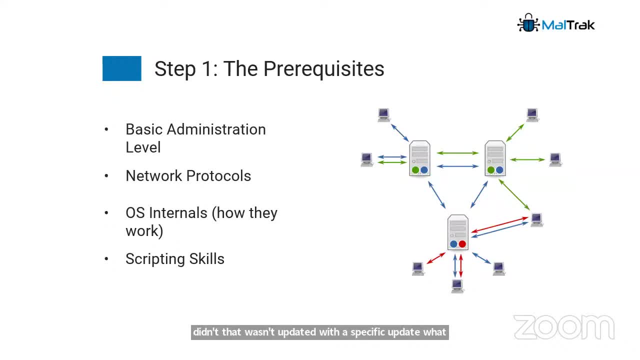 are the machines that were updated with that update and really manage with that. maybe for some machines or something like that, that could be like two, three commands that you need to really uh to collect all the updates that windows have have done in the last uh. you know, throughout the 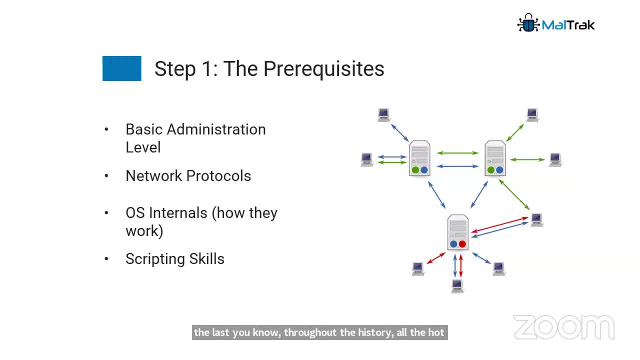 history, all the hotfixes, and then collect all the the information and export the excel sheet. that could be like five lines code. so that is basically what we do here in the scripting um. again about networking. uh, you don't need any certification on any of these steps, like 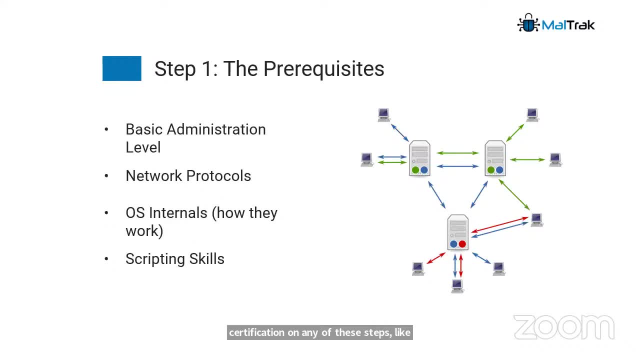 wherever that's scripting, wherever that's operating system internals, wherever that's linux or this network protocols, certification are actually are a killer in most of these prerequisites, because when you are going for certification here, specifically in the prerequisites, you learn as things that are a bit more way in. 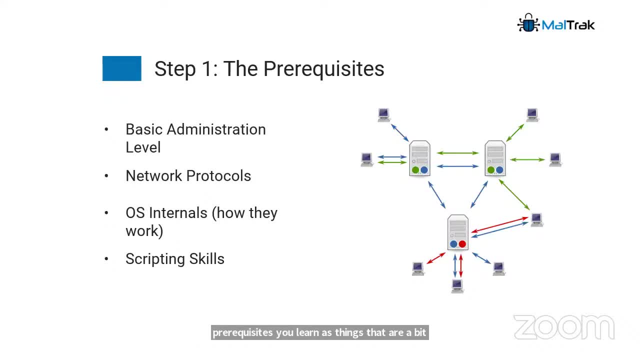 depth than what you need, like something like ccna, for example, is going to cover cisco. we don't need to learn cisco. we don't need to even learn routing protocols. these protocols are not really important in cyber security, but if you are a network engineer, they're going to be very useful. 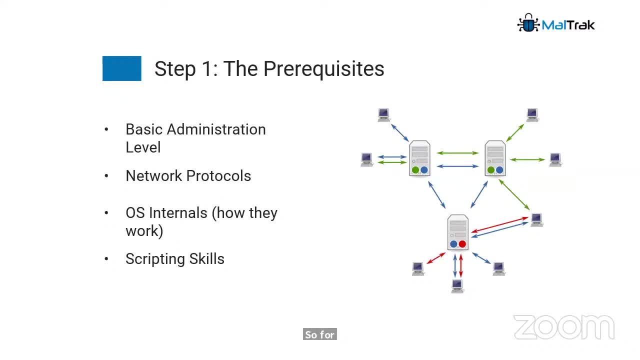 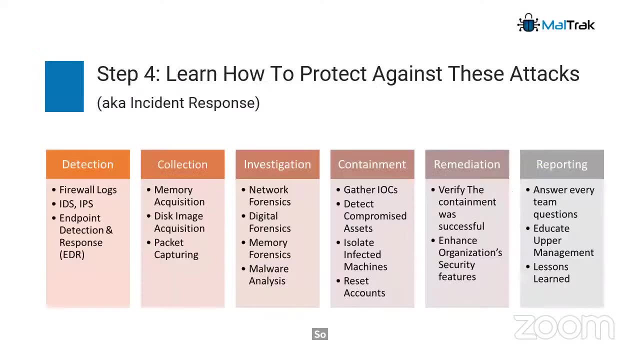 for cyber security. this, these uh, these specific uh, prerequisites are not really important. um so, okay, you have learned the prerequisites, that's fine. then we go to the next type, which is learning how to protect against the attacks. this is the instant response part, so you learn the. 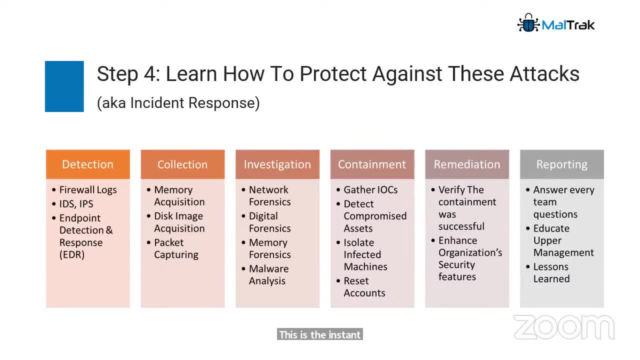 prerequisites. i don't know why step four here, but anyway, you have learned the prerequisites. now the time to learn the actual cyber security. and there are in. in responding to data attack, there's different phases. there's the detection- detecting an attack- um the collection phase, or the investigation collection, which means collecting different information about the attack. 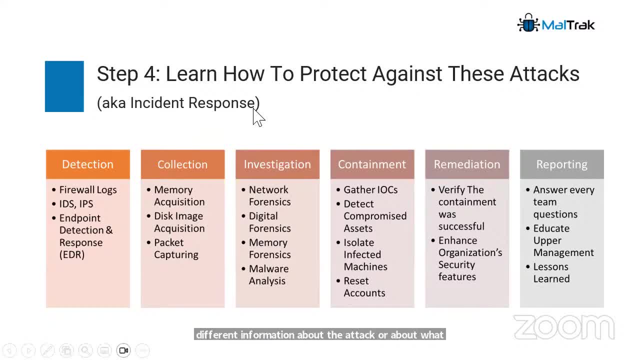 or about what had happened, and investigating them a little bit more in depth. and then you have the containment. so you basically, uh, you know, isolate the machines that are infected, uh, you know, like lock all the accounts are compromised, all of these things, and then remediating the attack. 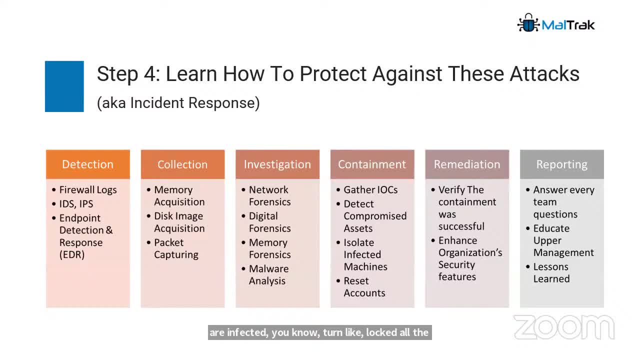 which means formatting these machines, resetting the passwords, removing everything that's treated to the attacker, and then report, answer all the questions about this attack: how it happened, why it happened, what are the weaknesses, what are compromised assets, what assets he has access to, what's exactly he was doing, why he was doing so. all of these different things, so um, all of these. 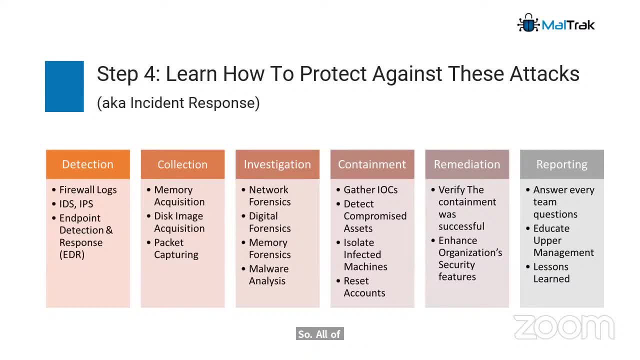 questions you answer in your report, so in you don't need to learn all of this to become a sock till one for sector one. for example, you focus on detection. you learn how, how this logs looks like. you are not detecting them yourself, but there are, let's say, alerts that you receive and you have to deal with them. 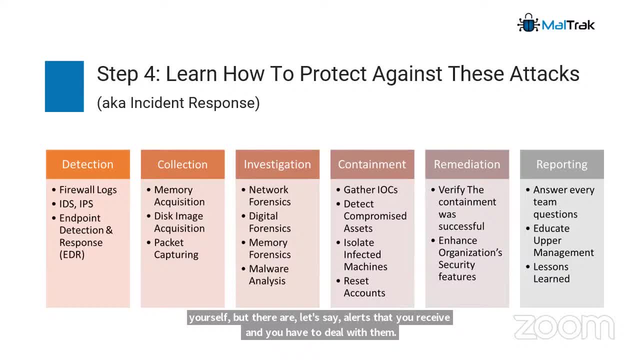 and that means that you have to to see what if this, if these alerts are real, you check different things in the log events, they check different things on the machine and see if they are real, real or not. and if they are real instance, then you you create a ticket about it, you report it to the next team. 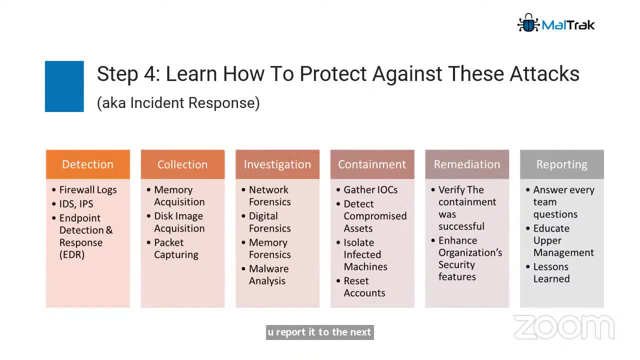 and that's it all right. and if they are not real, you just say that they are not real and you close the tickets about them and all of that. and this is what you do in the, in the sock tier one, most probably. uh, you still deal with different types of logs. maybe, uh, maybe, edr logs or system logs. 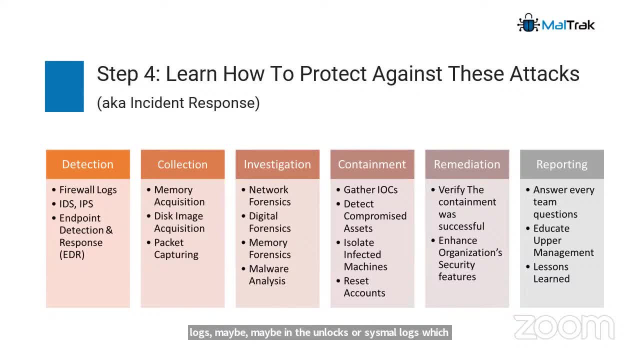 which is the host activities and new processes are being created and we are running from the temp, uh some different things like that. uh, strange domain this program is, uh is connecting to partial script that's unknown. uh, common prompt has been executed. all of these different things that's on the, on the host in the network, for example, you are dealing. 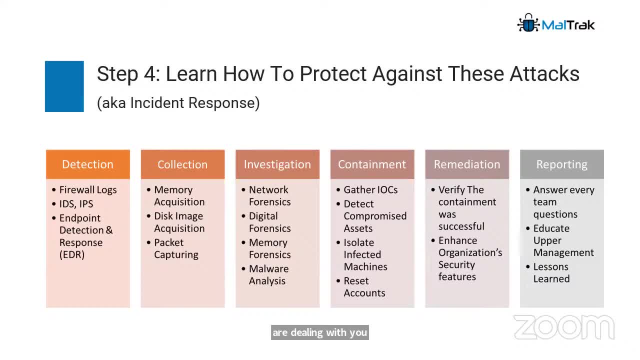 with you know, uh, you know ids, ips, the strange domain, suspicious internet activities, all of these different things, um, and also you have the identity, which is the host, and then you have the data, which is, you know, failed logins, stuff like that, right? um, so that is basically on the detection phase. then you go into the the investigation phase. 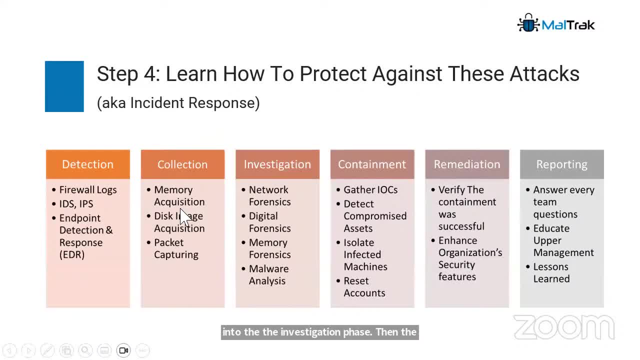 the investigation. the collection is basically um edr. you are taking these logs and investigating them further. so okay, there is. i found that this machine probably has been affected. let's see if it has done something else weird. right, let's see if the machine has done something else weird. 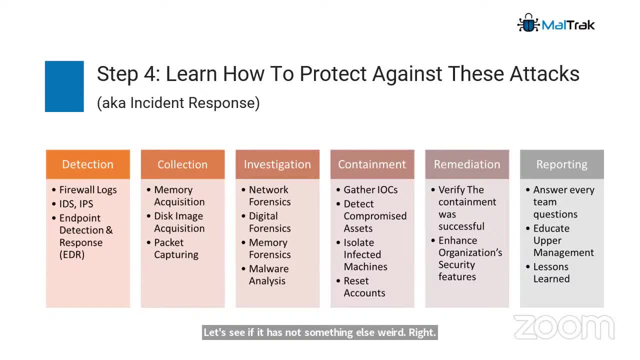 the same activities happened with other machines as well. let's see if this, this account, is also compromised and he did something suspicious and so on. i see a question here. if somebody use vbn and connect to that country ip, so how can we investigate? i am not. 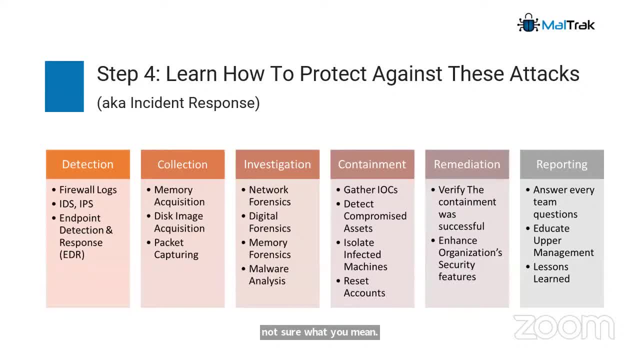 sure what you mean. connect to that country, which country or which company if you build a company, so that's the detection. the investigation is to go deeper and go deeper. that might require you to do also part of a little bit of forensics or collecting some artifacts from the machine itself. 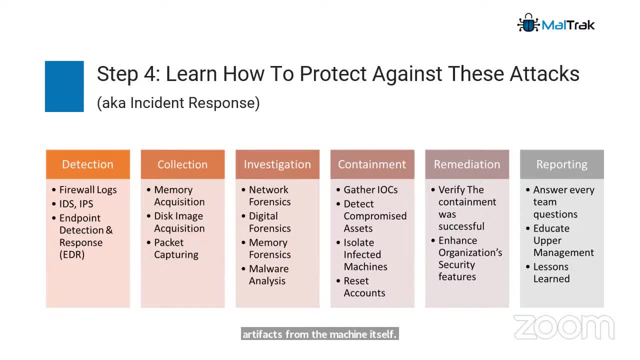 there's also part of uh, of the collection, of the collection and investigation phase. then after that you go into- this is instant response in sock tier 2 and sometimes sock tier 3, the in-depth investigation, then the containment remediation. that is basically done mostly by sock tier 2, which is basically 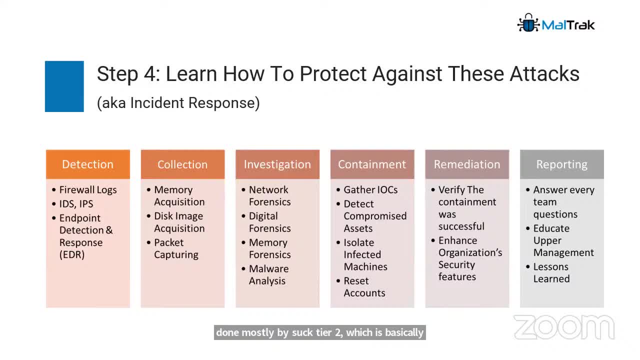 formatting the machines, come, you know, blocking ips and files and stuff like that, and hashes, resetting passwords and you know, and all that stuff. and then you go into the investigation phase, and then you go into the whole of this, cleaning everything up, returning back everything to where it was, and then the 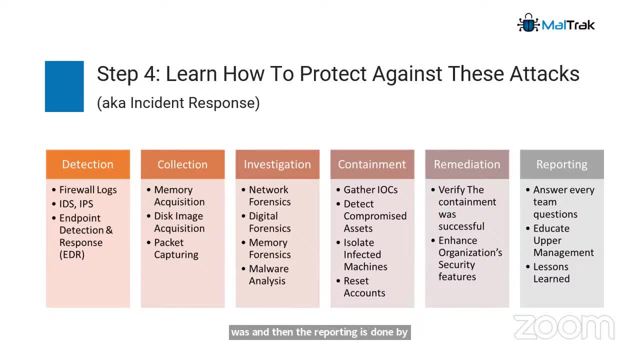 reporting is done by everyone in the process. so let's say: sock, tier 1, this is sock, tier 3, 2 and 3, this is sock, uh, tier 2 and 3, and this is everyone. makes sense. any questions about this part? any questions on this part? 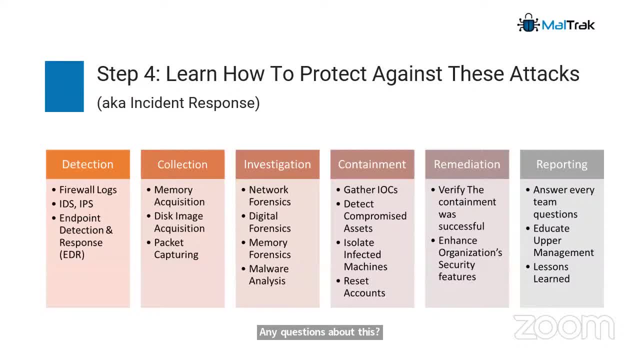 any questions on this part? any questions for you, Sam'. checked entire袋. any questions for you, Sam', here featuring Nizipo. any questions for you, Sam' here. this is the report from week 8, in which things to continue in the future. next um. 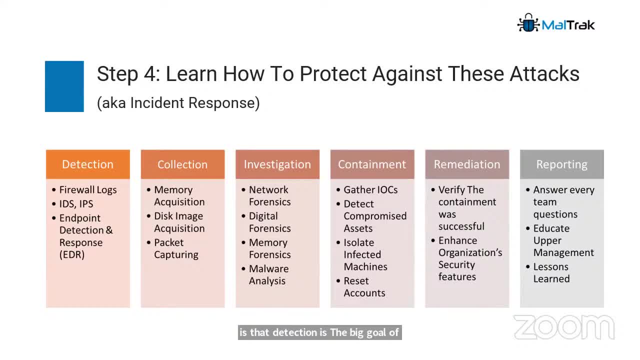 uh, what I am going to say for this did I let it work a bit, because this is what the test was doing. yeah, this is how how it works. okay, so just try all the way to the first. we guys will know you're not counting just the test time forward to r 한. 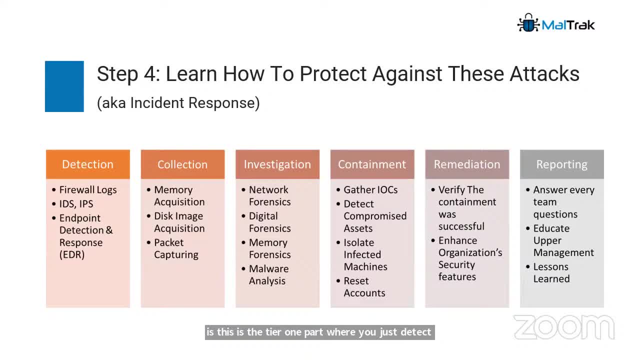 detect there's something suspicious, mostly based on alerts, and you investigate a little bit to see if it's true or not, and i'm going through every step now. so the detection is basically: you're sitting there as a sock tier one, you're receiving an alert from the ids, the ips, the firewall, the adr. 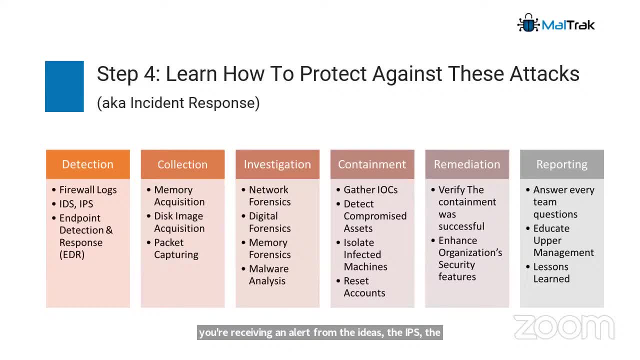 whatever that is in your send tool and you're investigating that- is it true alert if it's really a true attack or if it's not. if it's a. if it's a real attack, then you mostly okay it's a real attack. you create a ticket about it, you write information, you collect information about it and 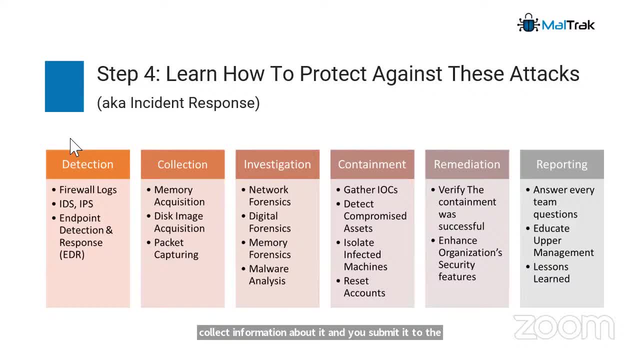 you submit it to the next tier- most of the cases right if you are in a multi-tier sock sock company or sock analyst team. so he push it to the next tier. the next tier does the investigation part, so he collects more information. try to dive deep. okay, we find that this suspicious domain, this machine connected to 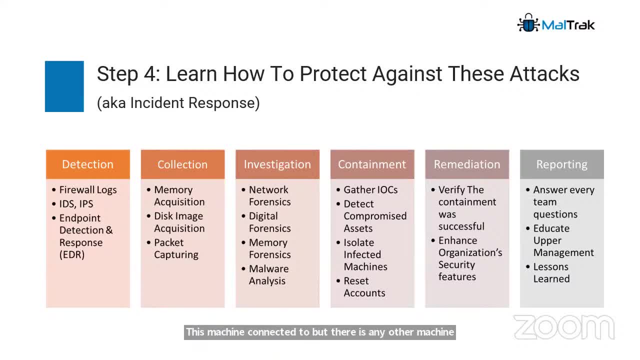 but there's any other machine connected to that domain. there's any machine connected to the ip of that domain. does this ip of that person try to log in somewhere else? what what this machine has done before this attack? what has done after all of this investigation process? that might require also that 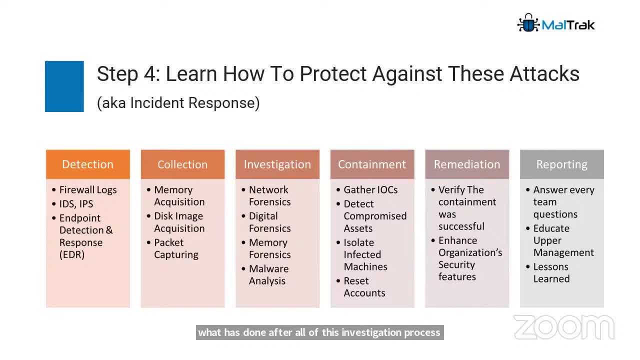 he goes into the machine and collect information, like memory dump or or some partial information, or use os query or whatever the tool he's gonna use to collect even more information from the machine to investigate it farther right. this is the collection piece, the collection and investigation process. um, so that is basically the whole next step then. then the third step is basically and: 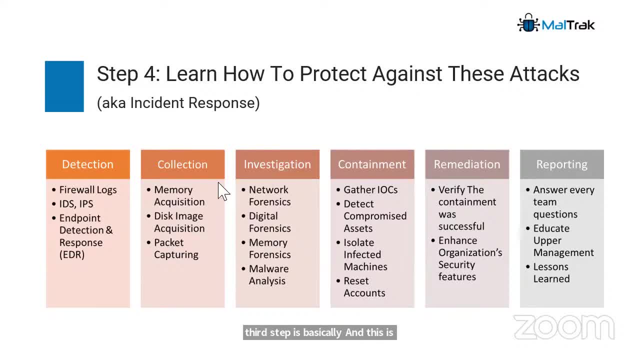 this is done mostly by tier two, this in-depth investigation, or tier three, and then the next step is containment and remediation. containment is basically okay. this is all the the. this is all the infected machines. let's isolate them. this is all the compromise that counts, let's, let's lock. 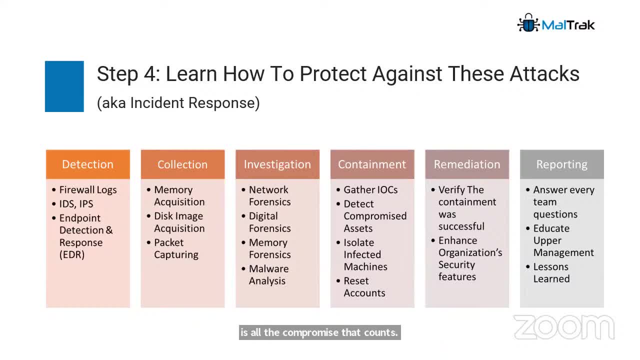 them. uh, this is all of the different uh domains. let's block them, all of these different things. and remediation is, you know, i isolated them. let me clean them up. reset passwords, you know, do all of this stuff and and make sure that i have removed the attacker completely. um, and then 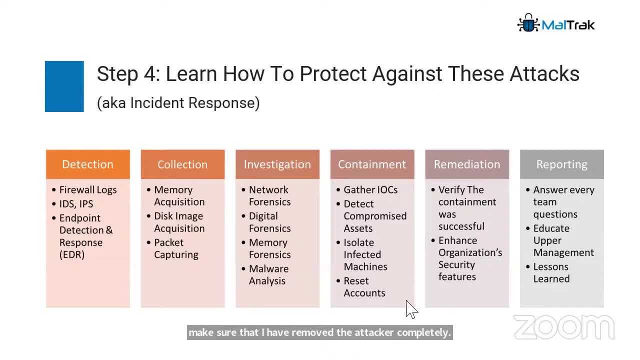 uh out of the system and now i can uh, i can basically uh, you know, i can say that this, the company, is clean again. this remediation process is mostly done by tier two, but it it's based on the investigation that had happened. i see a lot of companies when they have like security analysts. 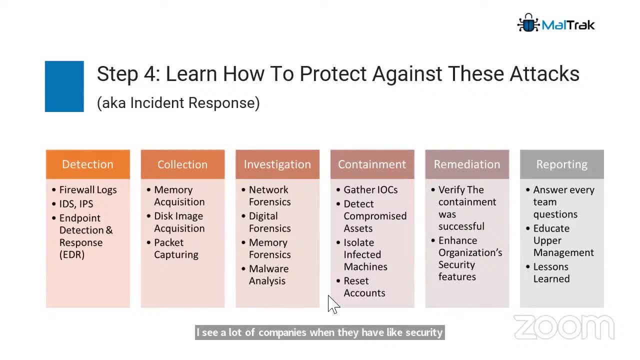 they don't. they don't do investigations a lot. the security analysts, they do only the containment and remediation and then back into the detection of new attacks and they don't investigate the things further, mostly threat hunters or, uh, or you know more, senior instant handlers or let's say, sock tier 3 in many cases that does in-depth investigation. 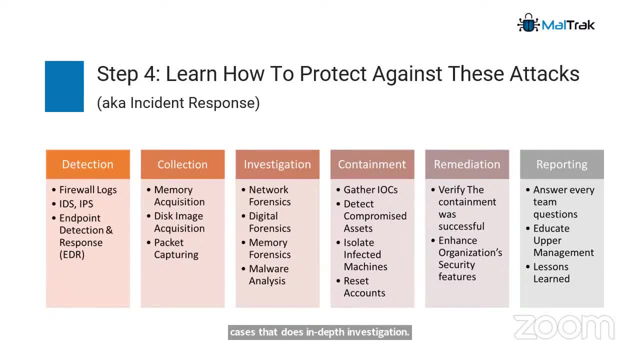 and after that you have the reporting, which happens in all cases. anyway, and i hope that answers you guys questions. is this session recorded? yes, it's recorded on youtube as you see it currently, and it's gonna stay on youtube on the exact same link and for you guys on zoom, you can go to my youtube channel. it's at maltrak security um. 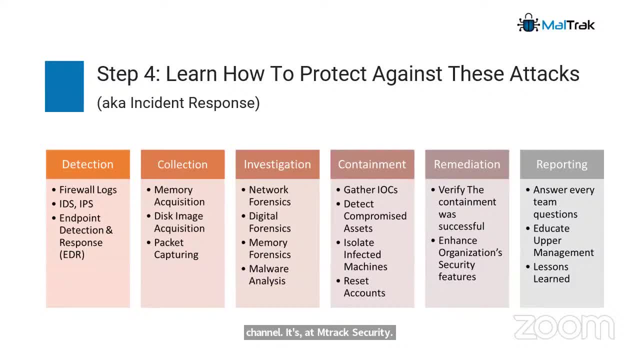 it's: um, i think youtubecom slash ads maltrak security. i think that's how it's written. let me check. yeah, that is how it works and it is there. it's called live demo. let's analyze the cyber security attack together and you're gonna see it on my youtube channel if you want the recordings as well. 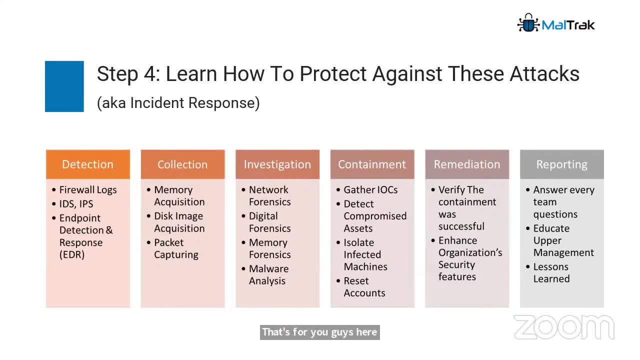 that's for you guys here on um, on zoom: perfect. so is it better to keep the contained devices connected to other security tools like edl, just to keep it under monitoring before recovery? depends on your edr if it does have the ability to isolate the machine, sure. 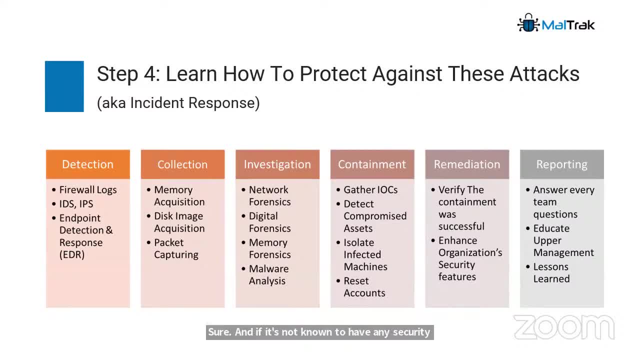 And if it's not known to have any security weaknesses that the guy can use in that communication and take over your. if there's a zero day or something, that's going to be a problem. But apart from this, yes, How I can go through everything. 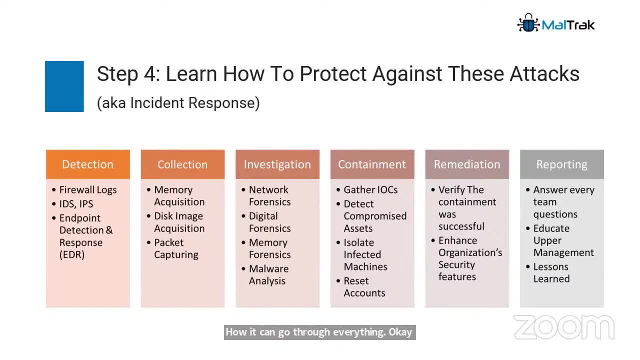 Okay, Please share a list of open source tools to build your own SOC environment for practice. I actually have a SOC. you know something that can help you with that. We have a project called Purple Team Cloud Lab Purple. It's basically on. 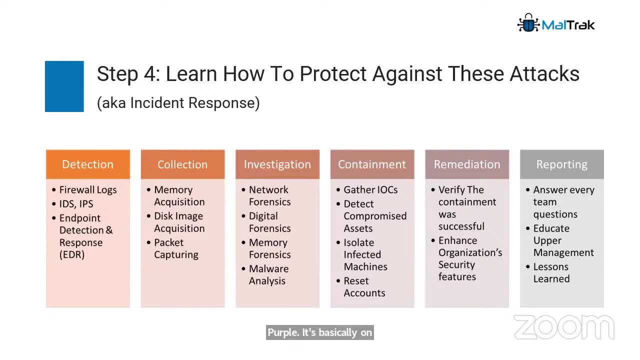 let me share it: Purple Team Cloud Lab. So I have a project that I have open sourced which allows you to build a SOC environment and an attack environment, like attack and defense, and you can test attacks in the cloud. It is called Purple Team Cloud Lab. 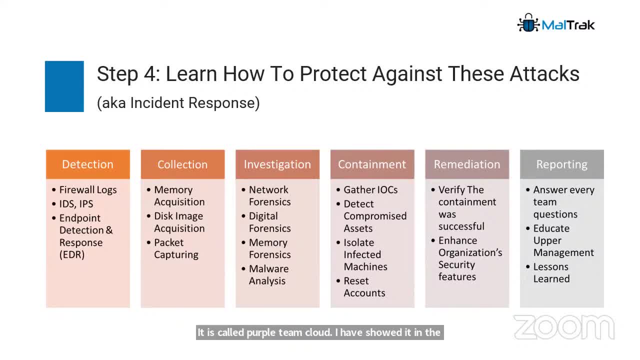 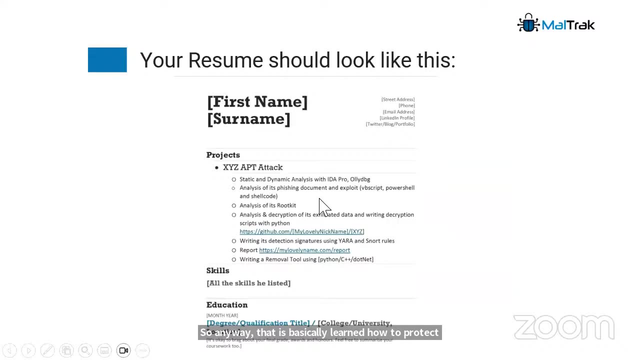 I have shared it in the link. You can guys take a look at it. We do also cover that in depth in our trainings, But yeah, So anyway, that is basically learn how to protect against the attacks. So, after you learn all of the skills, 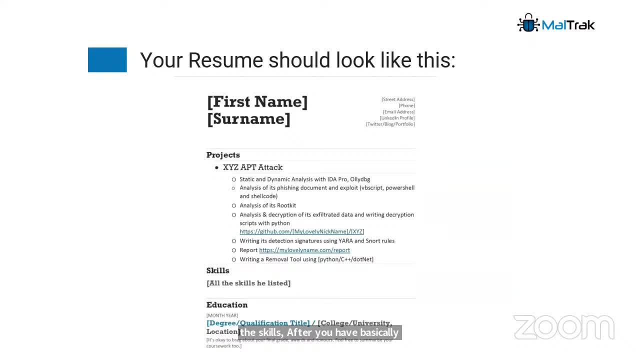 after you have basically analyze that attack by yourself, we go into the part where you're reasonable, right And a lot of people focusing on like I'm going to put my education here, I'm going to put all the certifications, then the skill set. 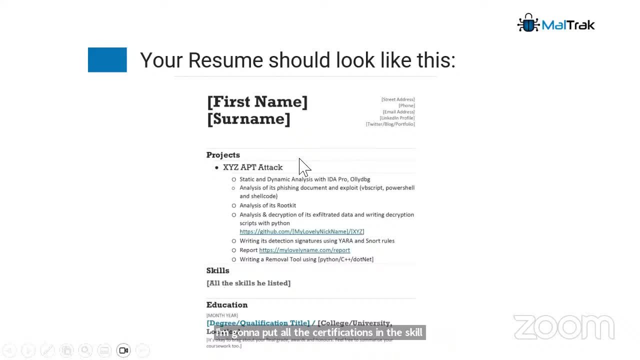 then the experience. If I have experience, I'm going to live by the experience first. then have all the certifications, then the education and then everything else, which is all good, But if these are your strength, if your strengths are certifications, 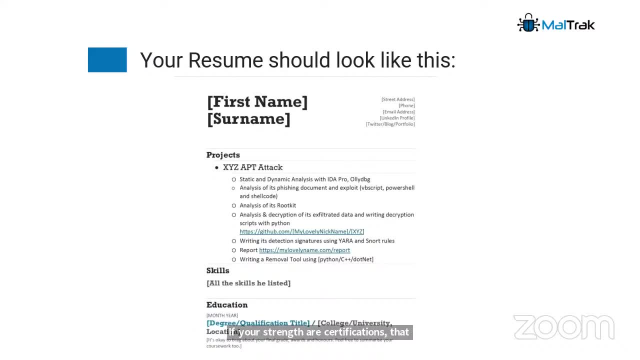 that is like everyone else has it. If your strength is experience, great. If you have already a few years of work experience, that sounds great. Put that in First. if they are a really big company, if you have not a lot of achievements. 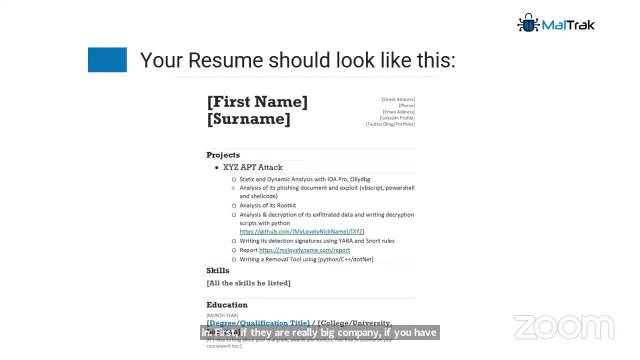 then write that down. If you have a few years of experience, write that down. If you have a few years of experience, then write that down. Sorry for that interruption. If you have anything in your experience, write that down. But what if you don't? 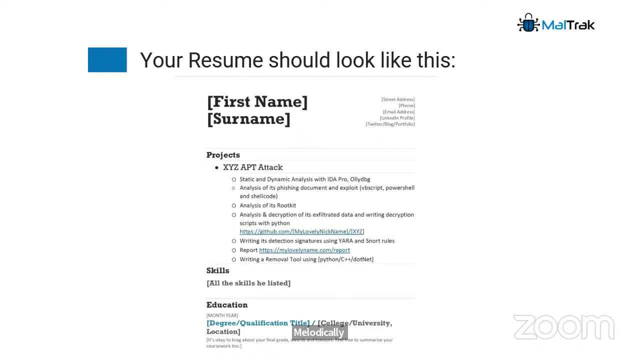 Well, there is a better option than certifications and degree. It's not better than having real experience, of course, but it is the second best after that, which is having having projects that proves your skills, As we talked about that in your blog. 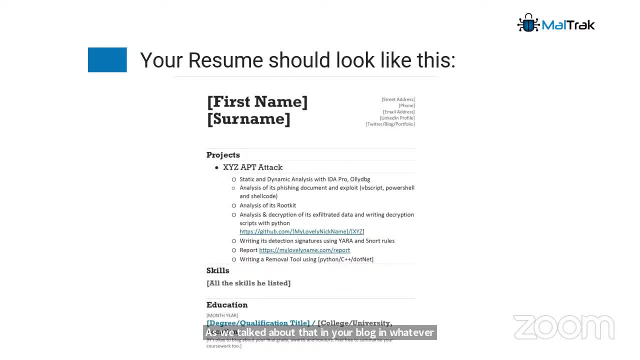 in whatever, wherever it's, in your website or mediumcom or whatever the app you're using. it works like that. You write here, let's say, the announcers you have done, the name of the project or the name of the blog or whatever. 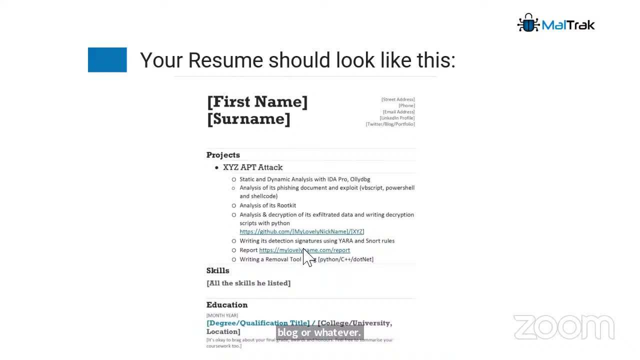 and then you write down all the things you have done in this attack, in analyzing this attack, based on the job description and based on the skill set they require you to do. So you're applying as a manual, for example. then you're going to take the same keywords they have. 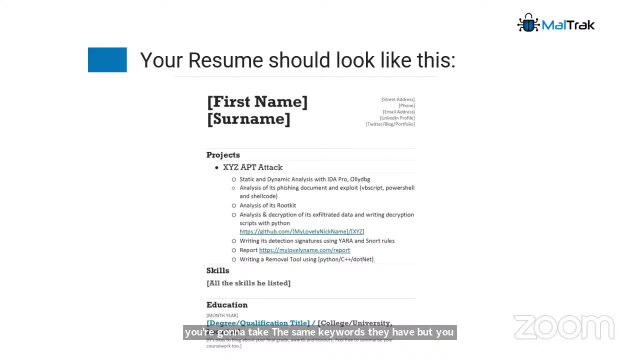 but you need to already. that's to be real that this you already have been using. this stuff You can take. basically, you can do static and dynamic analysis. You can write: okay, I have an analysis attack. I see that they require static and dynamic code analysis. 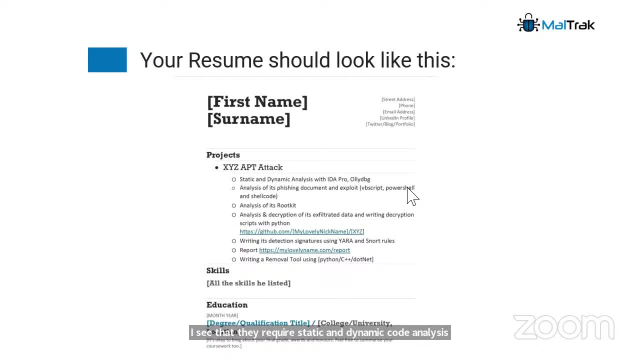 They require IDABRO and the Oli debugger. I'm going to take these, all of these, all of these keywords, and put them under under the project. I have done So I have done on this attack. I've done static and dynamic analysis using IDABRO and Oli debugger. 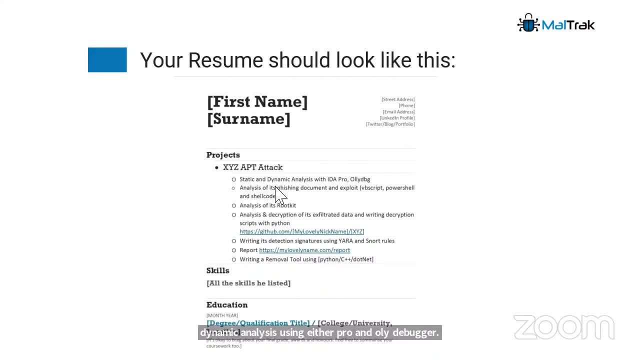 He wants me to analyze phishing and VBA macro. Okay, I'm going to write that down here: Analyze this phishing document and exploit VBA script, power shell shell code, blah, blah, blah. You put all of the keywords they have in the job description. 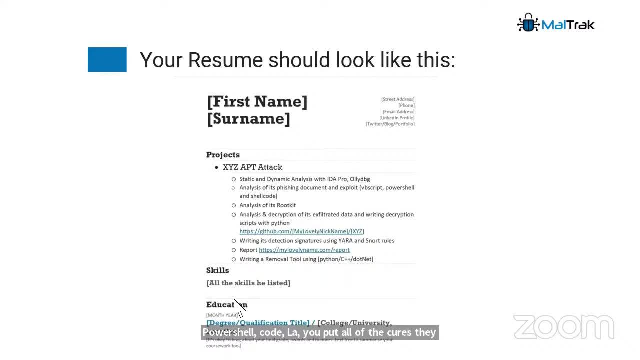 under your projects and then you have them again under your skills, But they have to be that you already have done this stuff for real on this attack. So you just need three projects like two, three projects with real skillset under them. 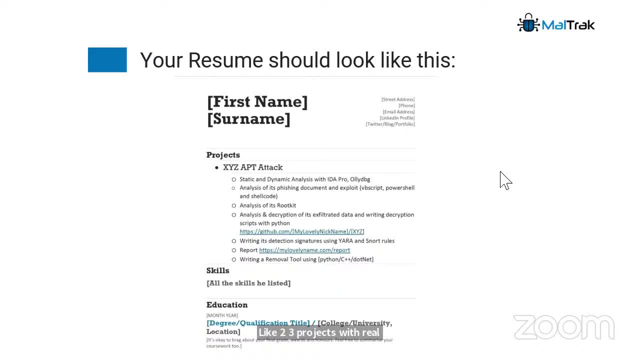 that basically represents the job description you're applying for. You're applying for instant response. They want you to almost stand Splunk or sem tools, So you're going to write that you have analyzed it in the same tool which is Splunk. between brackets: 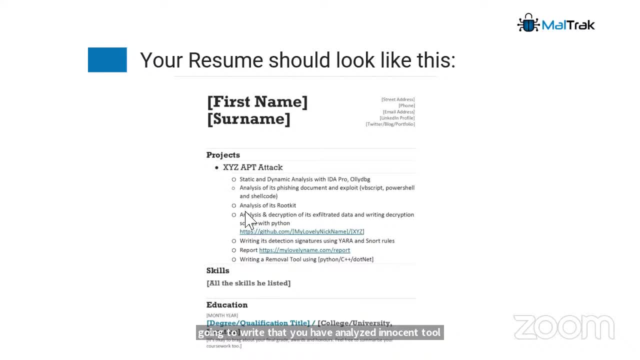 And they want you to be able to detect suspicious activities. I have performed in-depth investigation, detected suspicious activities throughout data mining in Splunk or queries in Splunk. you need to be able to create Sigma rules. I have created Sigma rules here. 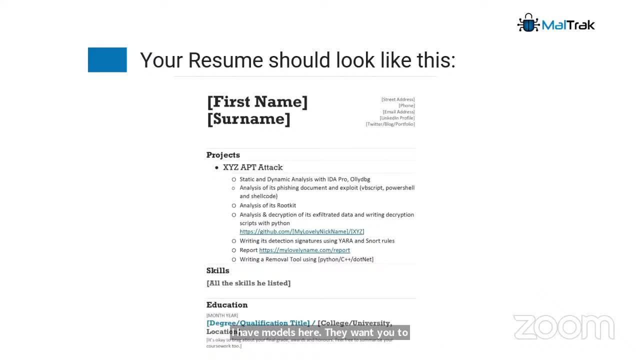 They want you to be able to create new IDS tools. I have created Snort rules, Snort IDS rule for this attack and so on, And then a link to your article And this resuming- and that's what happens to most of my students actually. 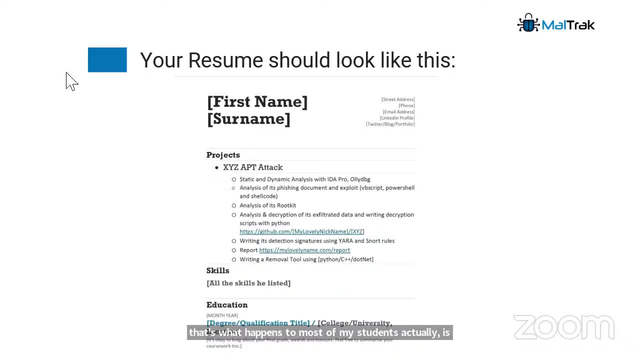 is that this resuming will help you pass the HR phase, because you have the same keywords as the job description, So it passes the data filtration. It shows that you have this under project, So most probably that you have done stuff. You're not just lying in your resume. 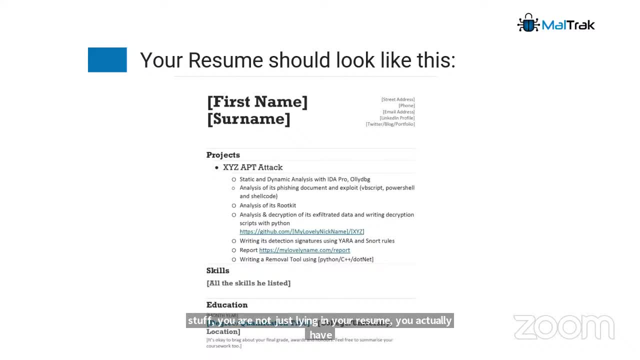 You actually have done this stuff, So that gets you to the interview. Also, if you share that in your LinkedIn over and over and you're gonna find other recruiters and hiring managers, they're reaching you out on LinkedIn to say: oh, we have this project. 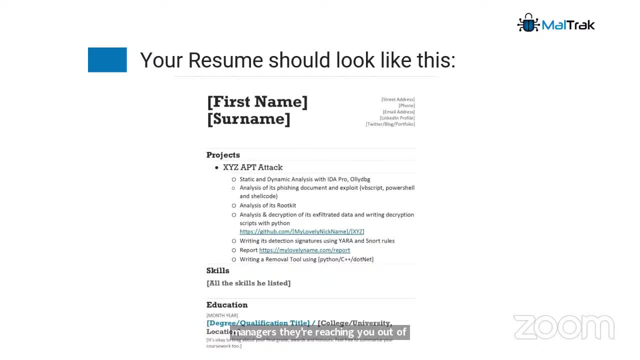 and we have this, this position, and we have seen that you are really good fit for this position. Why not work with us? And I had a lot of people who- a lot of my students- were actually getting a lot of recruiters in their DMs in LinkedIn and others. 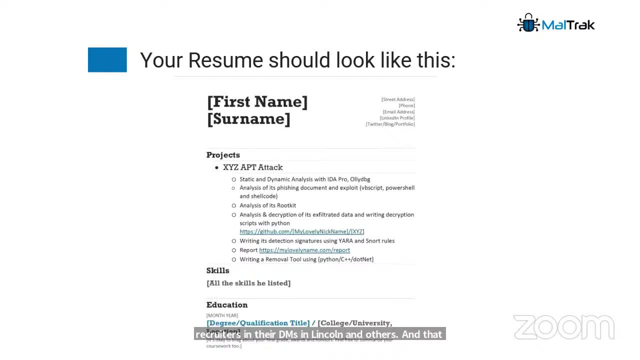 And that happened to me as well: from Microsoft to Kaspersky, not Kaspersky from Microsoft to other different companies in Germany and in different companies, different countries around Europe that were reaching me out to work with them on my LinkedIn. Why? Because okay. 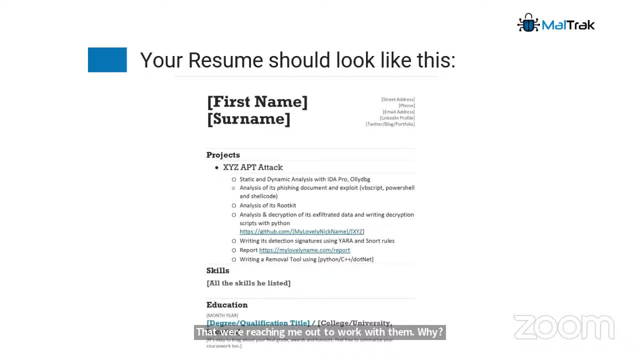 your. my LinkedIn profile is very optimized and, at the same time, I do share my own projects there And that's why I'm getting that visibility. So this is the most important part. So does that make sense for you guys? Is that making sense for all of you? 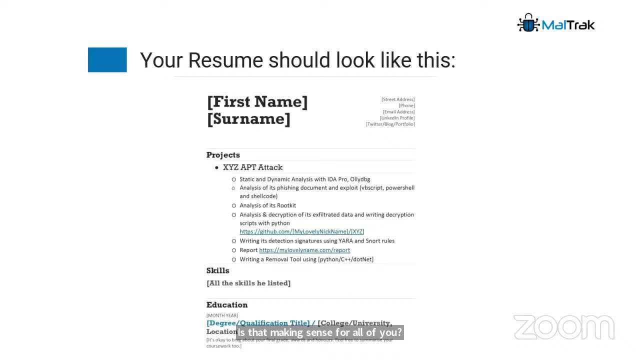 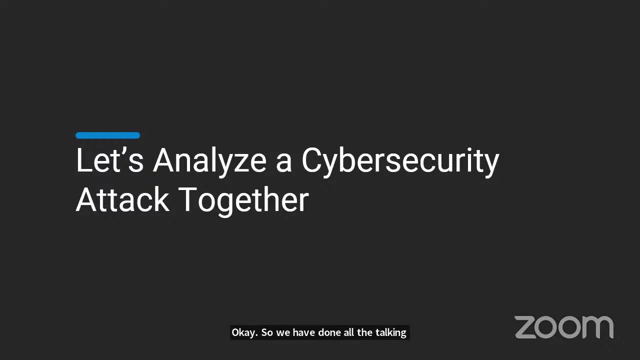 Thumbs up if you're still with us, Okay, Okay, So we have done all the talking. Andrei, do you have any questions? I guess Anybody has any questions, anything, Okay cool. So, Komlen, you have a question. 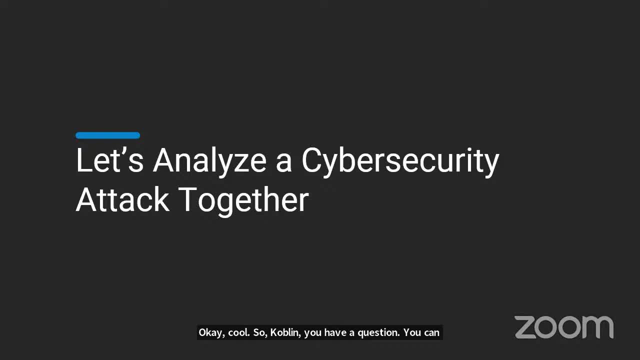 You can write in the chat. Can you write your question in the chat, Komlen? Yes, Komlen, can you write it in the chat, in the Zoom chat? I think he's trying anyway. So anyway, we're gonna get into the main meat of the presentation. 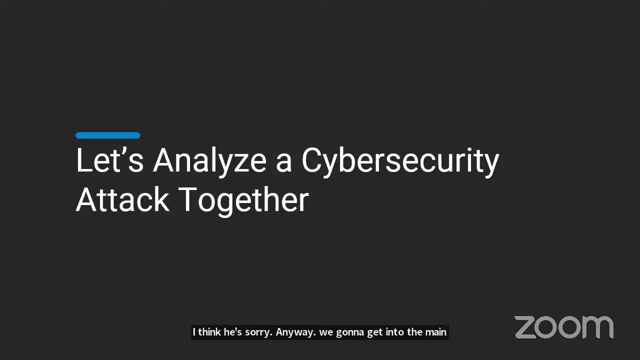 So, anyway, we're gonna get into the main meat of the presentation. So, anyway, we're gonna get into the main meat of the presentation today, which is analyzing an attack I took for too long And I'm also sick, so I'm talking a bit slower than usual. 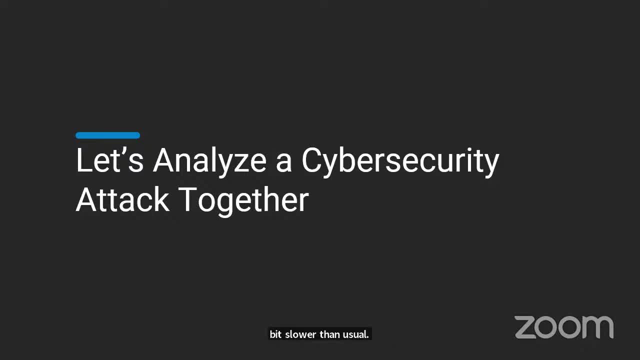 I mostly talk really fast, So today I'm talking in the normal speed and I feel like the time has wasted Anyway. So what we're gonna do today is that we are going to analyze an attack together, And this attack is basically gonna be: 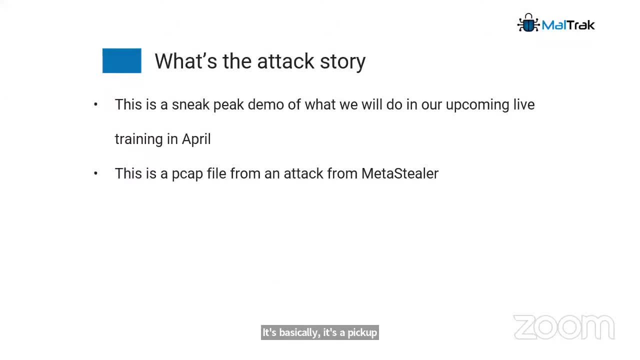 it's basically. it's a pickup file. We're gonna look into how we can analyze it through Wireshark. We're gonna look into how we can analyze it through Wireshark shark with a cheat sheet that we already have and, um, and this is basically a small demo of what 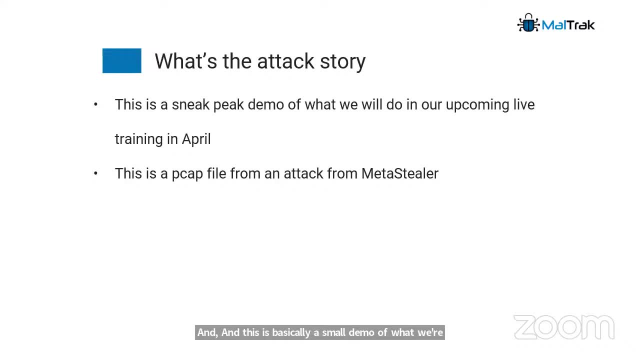 we're going to have on 20th of april, so intuitive april, 21 of april. uh, in this weekend, saturday and sunday, the- not the next weekend, but the weekend after- we are going to have a small live training where we will cover, uh, how we can analyze a full attack together. it's not going to be me talking. 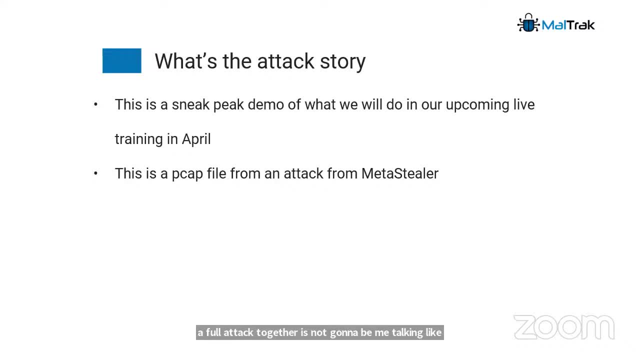 like that all the time. it's going to be mostly working together, analyzing different attack over zoom, and i'm going to share more information about this training as well. you're going to get the cheat sheets that we are going to use today and other cheat sheets as well on how to that. 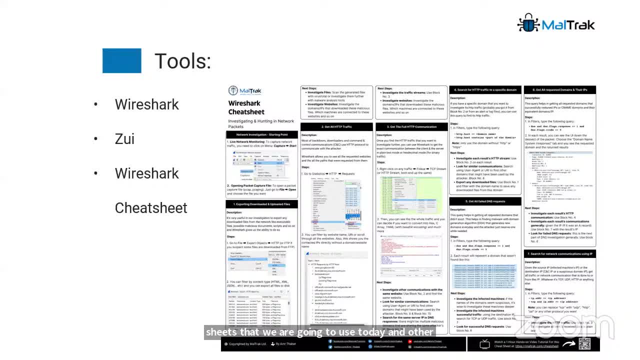 will going to help you investigate um an attack more in depth. this is basically have all the step by step to analyze an attack, so it's not just a demo of how to use wild shark. it's not about that. it's not like a cheat sheet that you see online. it's basically a step-by-step analysis, so you're. 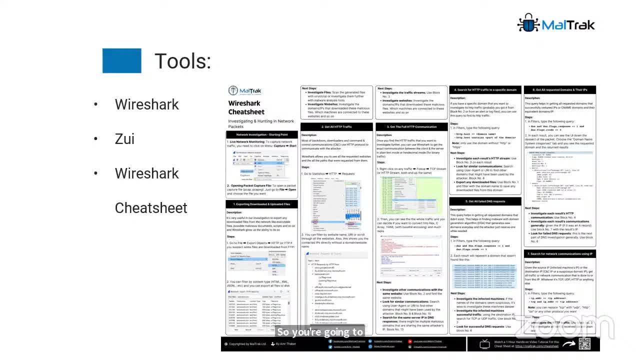 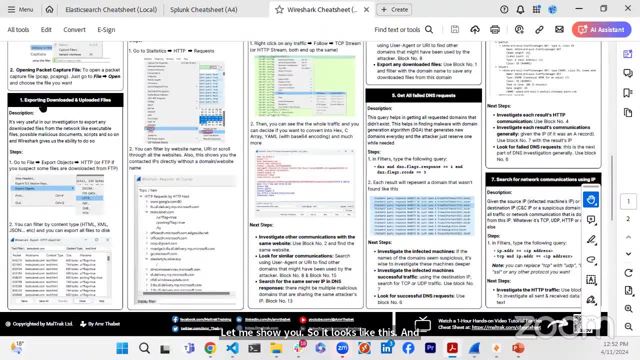 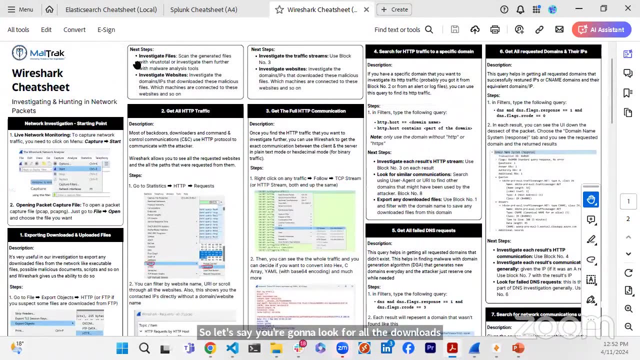 going to have. let me show it to you. so it looks like this. and basically, if you invest, if you look further, there's a step-by-step analysis. so let's say you're going to look for all the downloads, uploaded files. if you find download, upload files, you're going to have to do one, two, three, four to investigate. 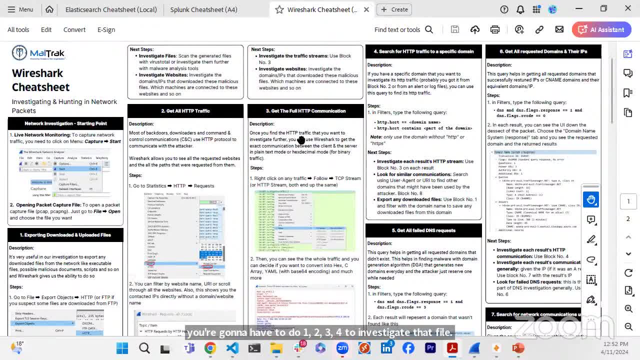 that further. each step of this will take you into another block. let's say, i want to scan the, the- okay, the scanning and virus total. but also we want to investigate the domains and the ips to get a domain and you're going to go into this process and you're going to investigate the domains. 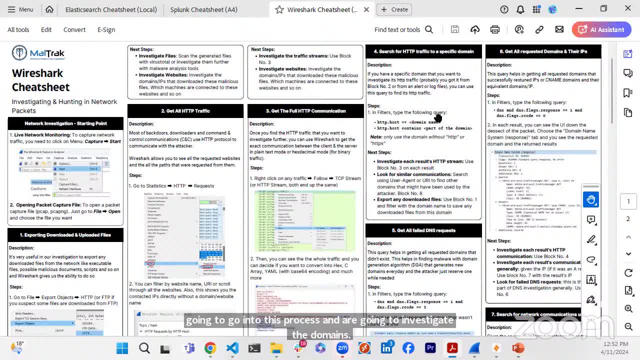 once you find domains, you're going to have next steps and you just following these blocks, one after another, after another. each one, each block guides you to the next block, and then to the next, and then to the next, and after that you are analyzing a full attack just throughout this. 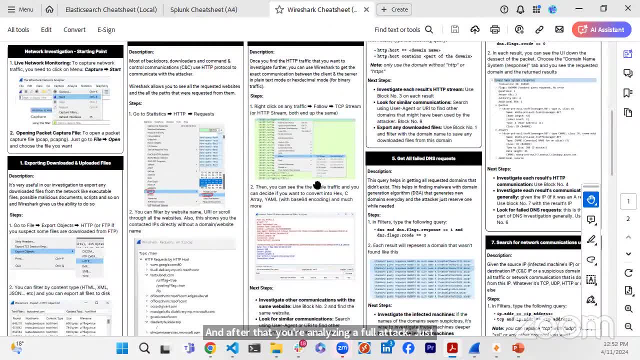 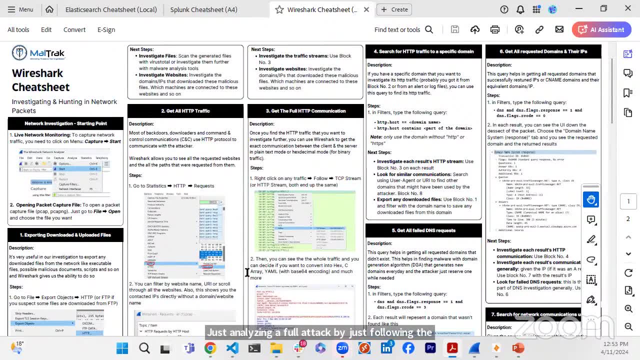 process right, just analyzing a full attack. uh, by just following the blocks one after another until you have a full attack analysis, and we're going to put that into a test. right now, we're going to use this wash, this wireshark cheat sheet. but throughout our training in april, we're going to have not just 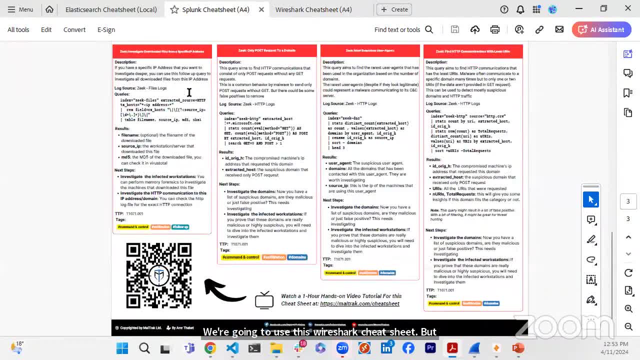 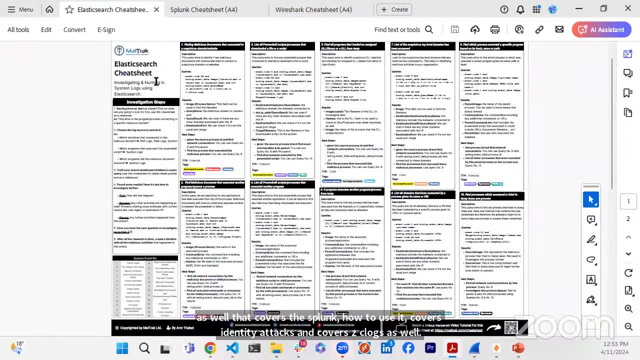 this one. we're going to have one for splunk as well that covers splunk, how to use it, covers identity attacks and covers zeek logs as well. and we're going to have elastic search that is focusing on elastic search and, as well, system logs, and we're going to invest to use that as. 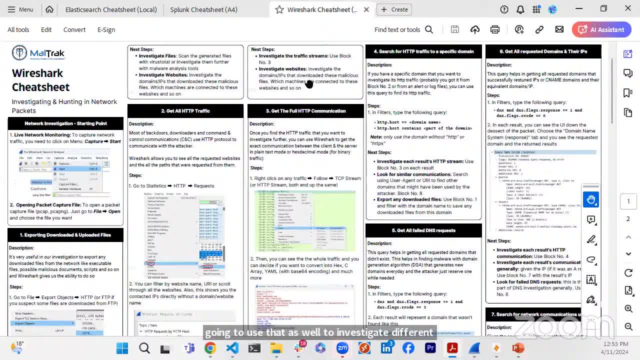 well, to investigate different attacks, and all of that is going to be used in this process. we're going to cover, you're going to get all these cheat sheets and much more in our april training. i'm going to talk more about that training in a in a minute, but for now let's get into an attack. 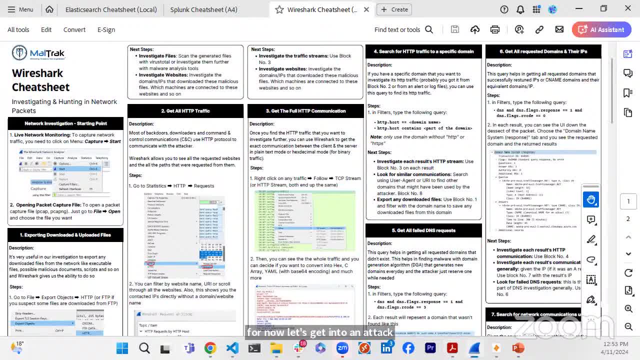 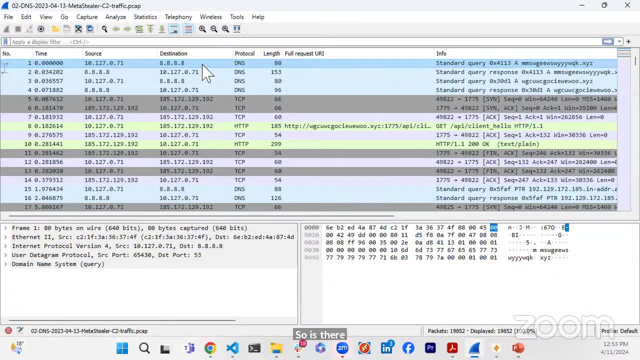 together, shall we? let's go. so here's the. so we have here a pickup file for a malware called metastealer c2 traffic. so this is from malware traffic analysiscom or net and, and this and this has, we believe it has- something suspicious, but we don't know what's. 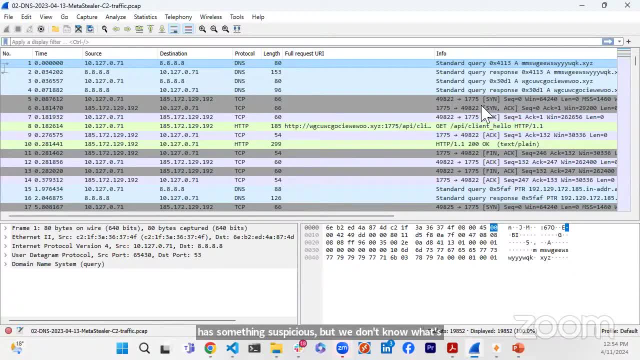 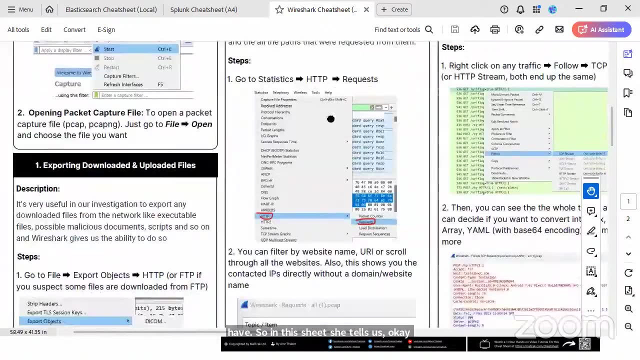 going on and what we're going to do is that, if we don't know what to do, what's exactly the next step, let's go to the cheat sheet and see what ideas we can have. so in this cheat sheet it tells us: okay, there is multiple starting points you can start with. you can basically export: all downloaded. 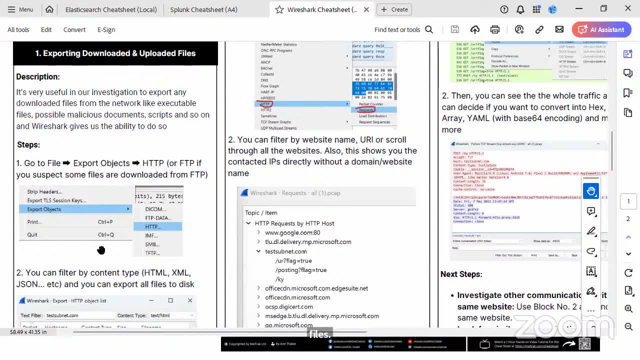 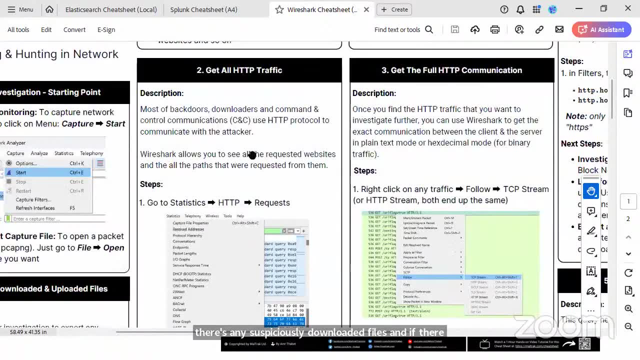 uploaded files. look at all the downloaded uploaded files and you can export all the files and see if there's any suspiciously downloaded files and, if there is, do something about it. or you can get all the hdmi traffic and see how all of this traffic looks like and see. 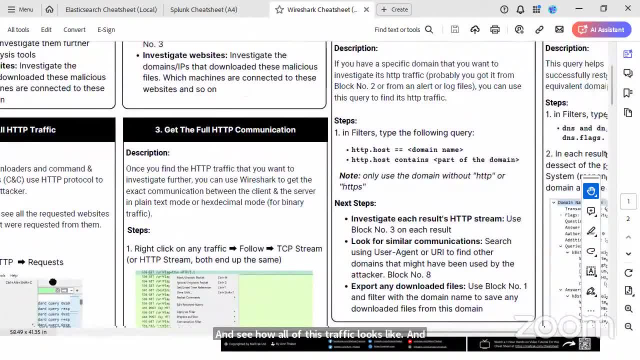 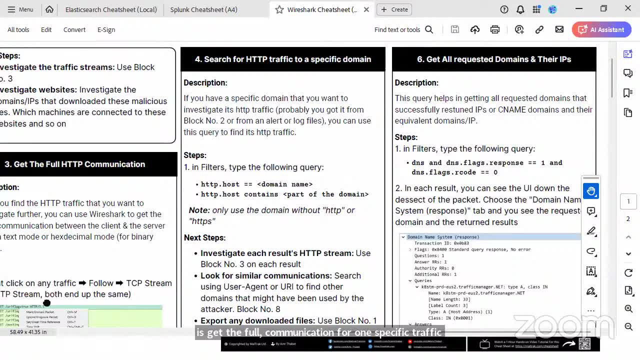 what are the domains and stuff like that? um, and then you, this is get the full communication for one specific traffic, so that's not a starting point. um, there's also here, good, all requested domains and their ips, right, and if there is a good basis and you can get the full communication for the different ways. 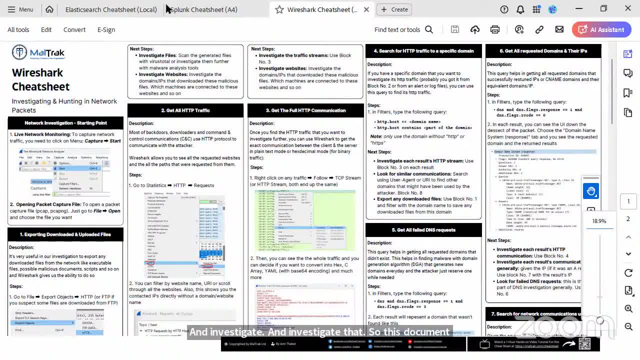 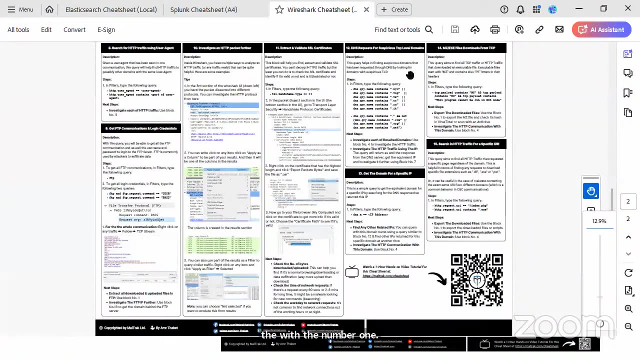 you can get the full information for the different ways that you can get your data, and not just the hdmi traffic, and you can also. okay, so in this case we can search for sql and we'll go to the page with all ideas you can investigate further. so all of this, most of these boxes, you can start. 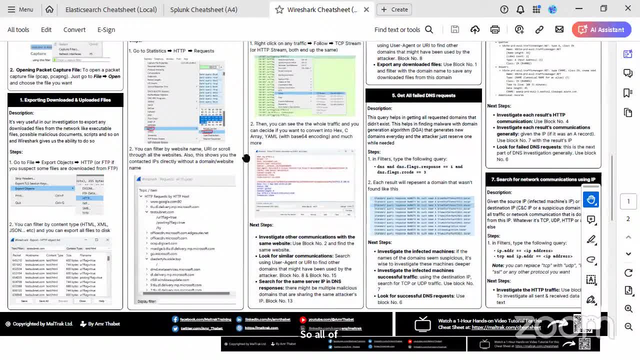 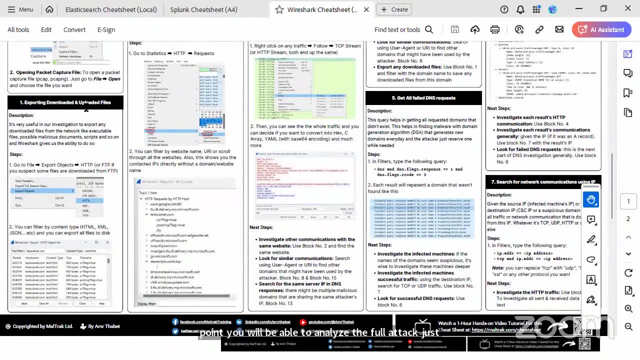 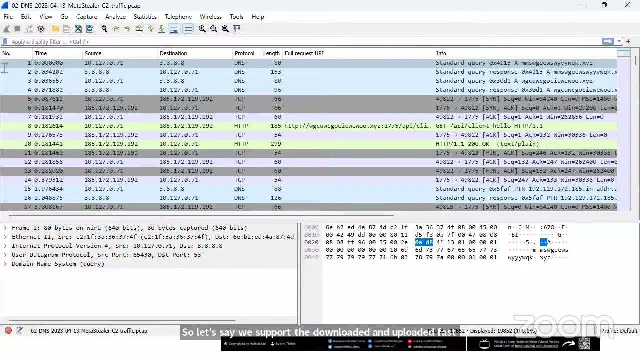 with as your first initial step and, whatever the starting point, you'll be able to analyze the full attack just following through all of these different steps. so let's say we're going to export the downloaded and uploaded files. let's go to our shark and follow the cheat sheet in the 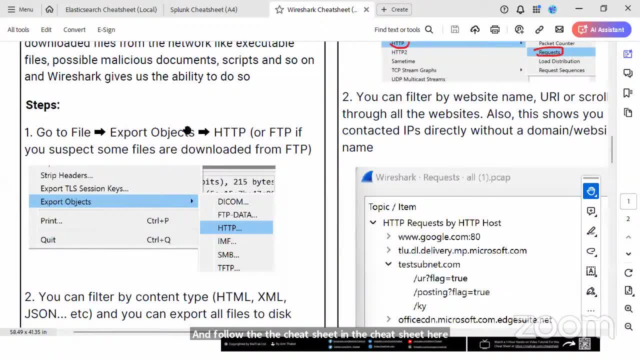 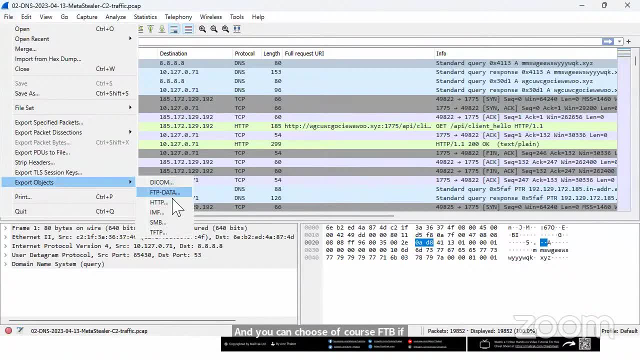 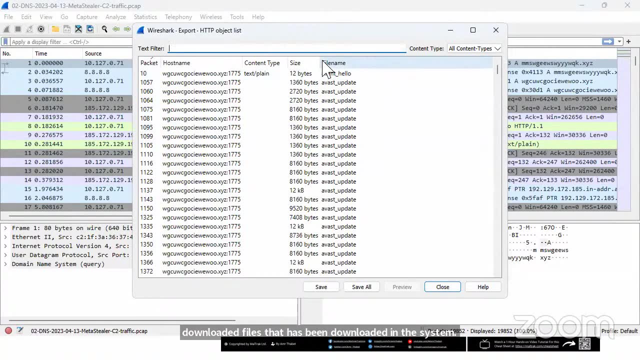 cheat sheet here is saying that go to file export objects and then hdb, and you can choose, of course, ftb if you have ftb traffic. so export objects, hdb, and here we're going to see all the downloaded files that has been downloaded in the system and their exact size. we see here that there is a 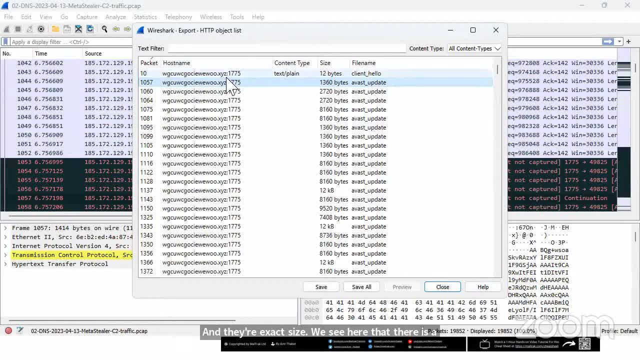 specific file called avast update that has been downloaded at xyz from this weird domain dot xyz, which looks very suspicious by itself, and it does have the port 1775, what, which is not a typical port- that's really suspicious port- and avast update. avast will not update from there, so that is. 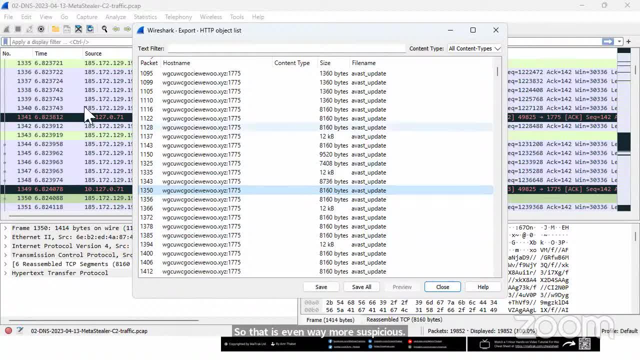 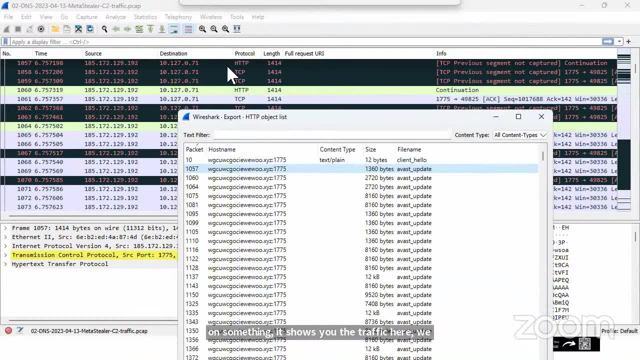 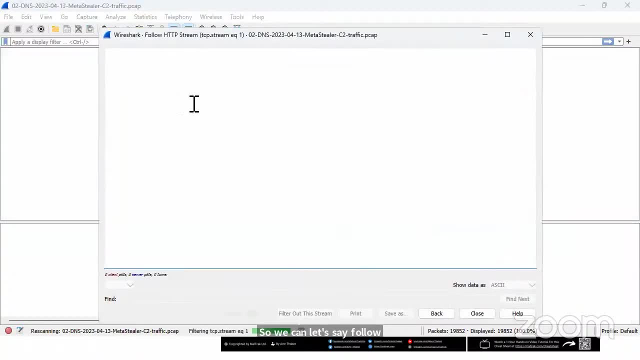 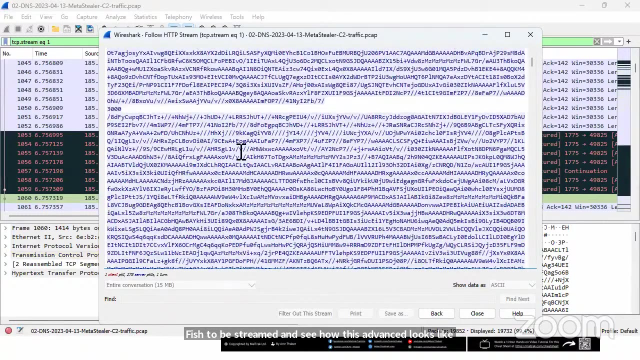 even way more suspicious. we can go and investigate that further. we can see that once you click on something, it shows you the traffic here. we can look into that traffic so we can, let's say, follow hdb stream and see how this avast looks like. it looks like just random data being sent up here. 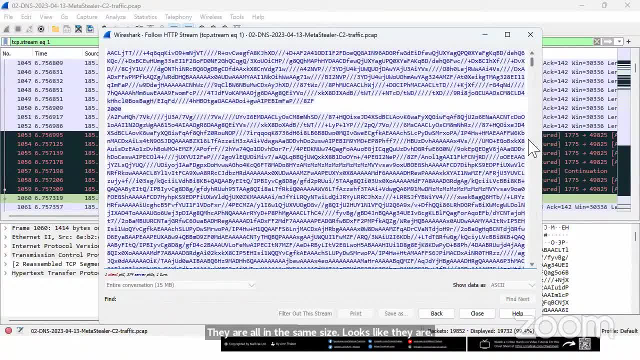 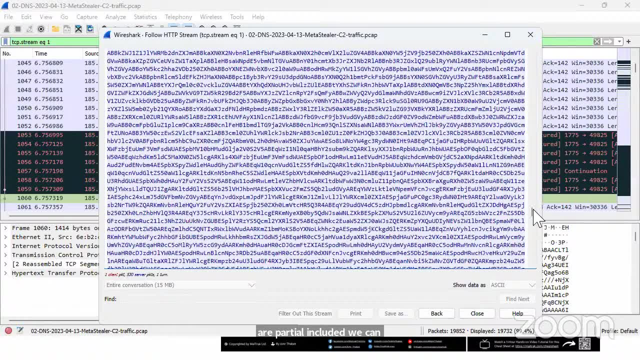 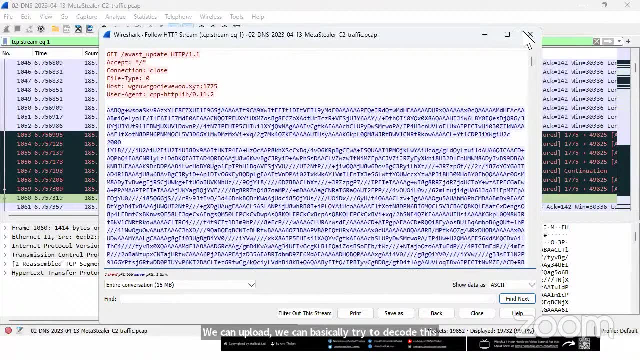 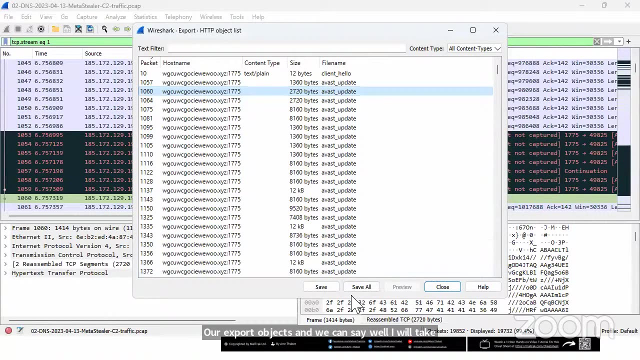 they are all in the same size. it looks like they are. they are partial encoded. we can basics for encoded and they are really long data we can upload. we can basically try to decode this base export data. we can just go back into our export objects and we can say: well, I will take that and then I'm gonna save that one into a file up here. I'm. 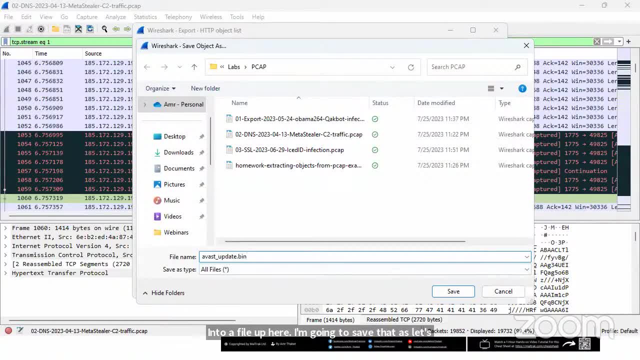 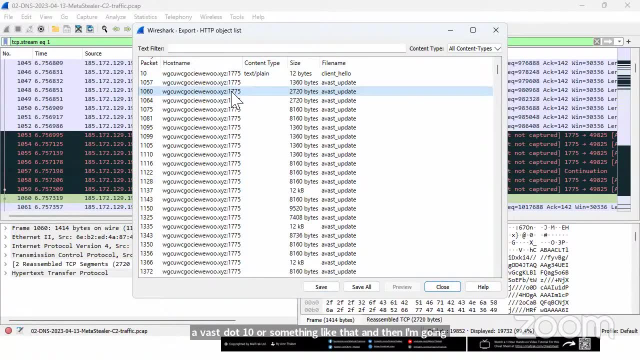 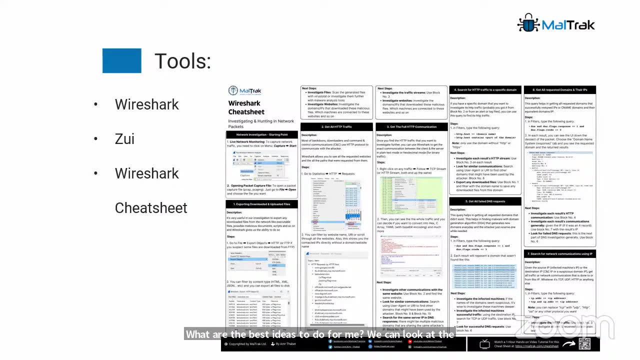 gonna save that as, let's say, a bastpen or something like that, and then I'm going to upload it to virus total or do something, or I'm going to do something about what are the best ideas to do from here. we can look at the cheat sheet again. sorry, the actual cheat sheet. 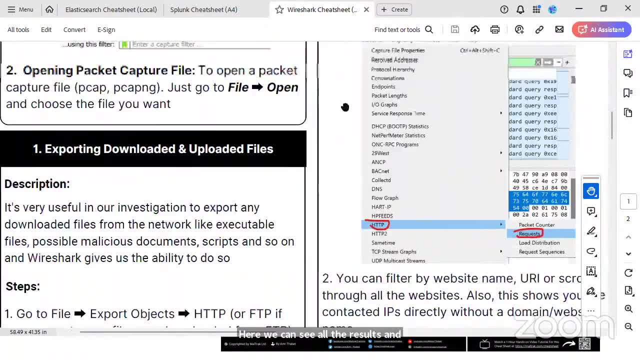 Here we can see all the results. and it tells us this: well, let's say, here we can almost see these. we see these three mind games and some privacy problems here, and also we will have to process moreכ. and it tells us this is the continuation up here. 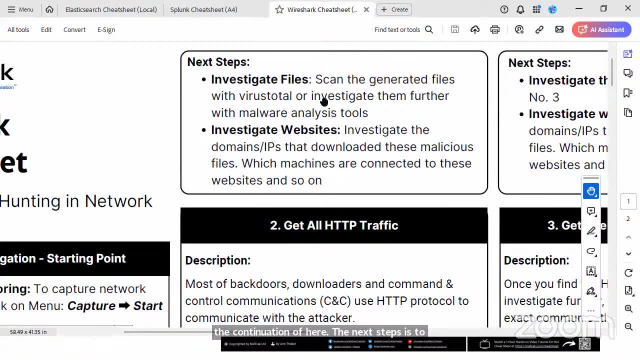 the next steps is to investigate the files, scan the generated files with VirusTotal and investigate them further with modernized tools so we can take that Avast update. and okay, let's try to investigate this Avast update by, let's say, by virus, by, like, let's say, B64 decoder. 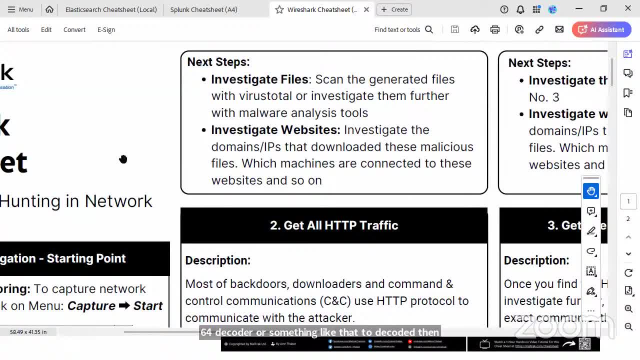 or something like that, to decode it, then start analyzing like what's this file, you know, finding what's this data is, This is one thing, one step and put uploaded to VirusTotal and so on. The second idea that we need to follow: 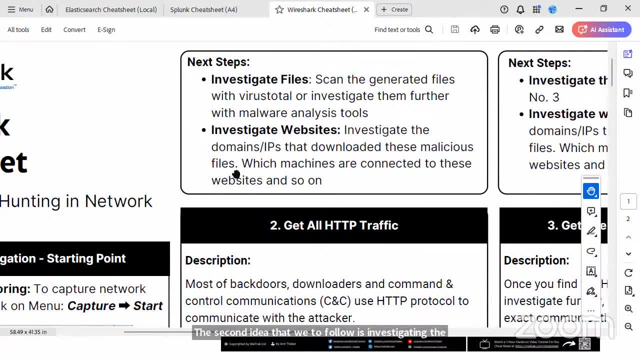 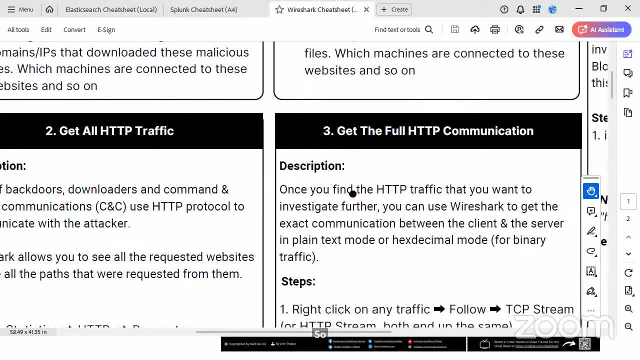 is investigating the website, investigating the domains or IPs that these files have been downloaded from. So how are we gonna investigate them further? Well, there is here something that allows us to get the full HTTP traffic, which, what we did, right click, follow TCP stream. 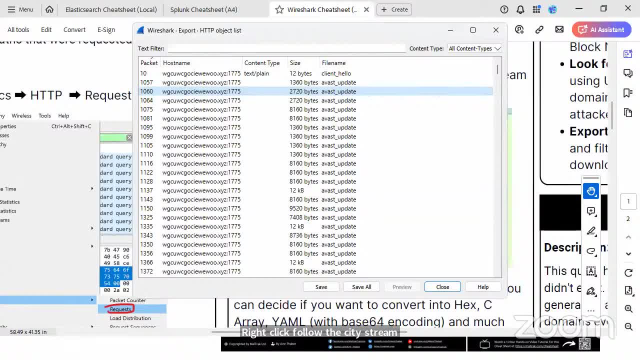 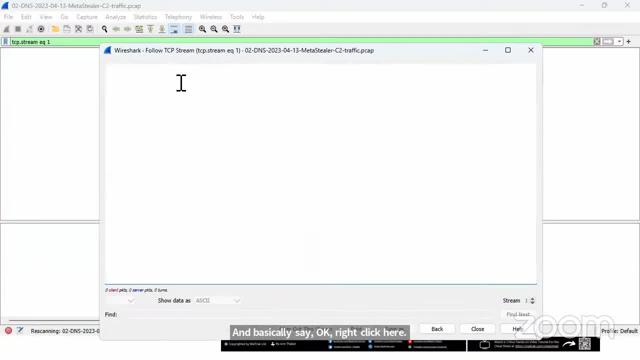 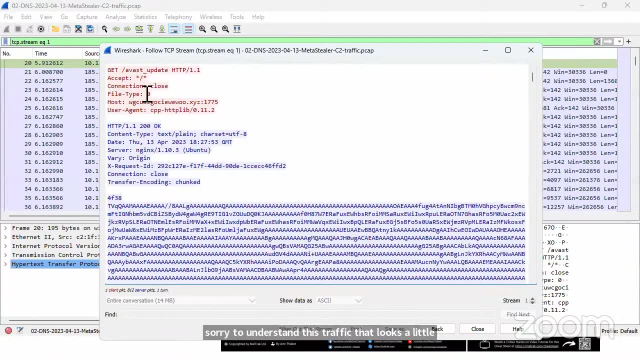 so we can go to a backup file and basically say, okay, right click here, follow TCP stream and see how the traffic looks like, And then I'm sorry to understand this traffic. It looks a little bit different here. We see that basically that is the host. 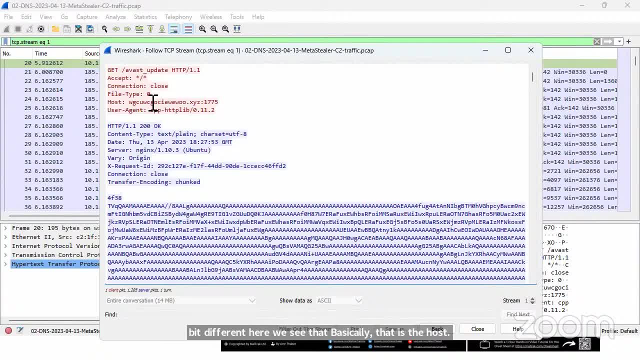 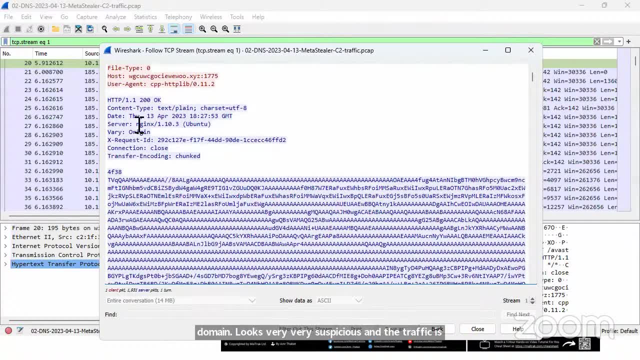 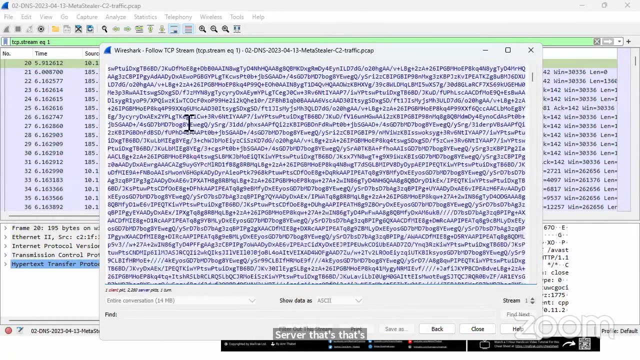 The user agent looks really suspicious and this is the domain- looks very, very suspicious And the traffic is coming from also a NGIX server. that's a Ubuntu server like Ubuntu, Ubuntu machine, and there is, you know, kind of a very long data also this weird data. 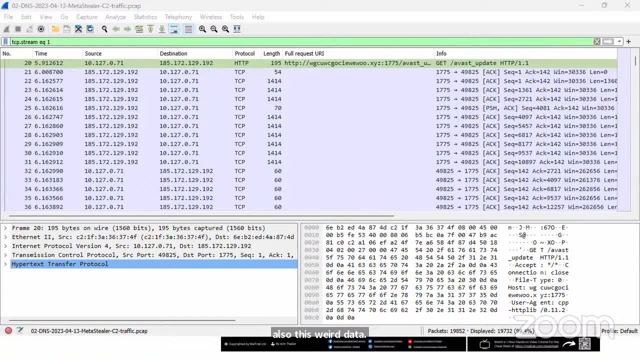 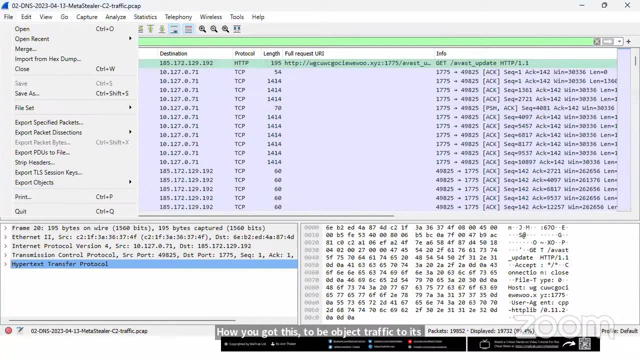 So this is the response we are getting up here, And okay, so what to do? how you got this? HTTP object traffic. So it's files, export objects, HTTP, and also you can find it in the cheat sheet as well. That's why we keep it in the cheat sheet. 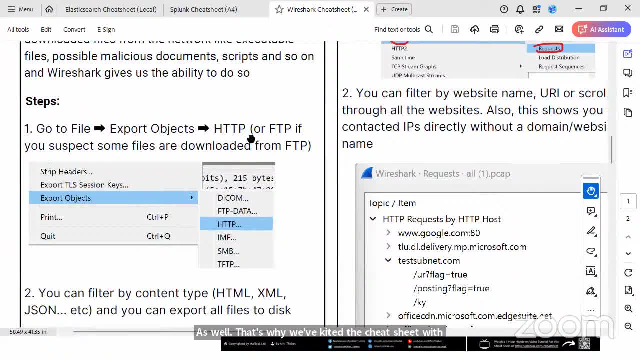 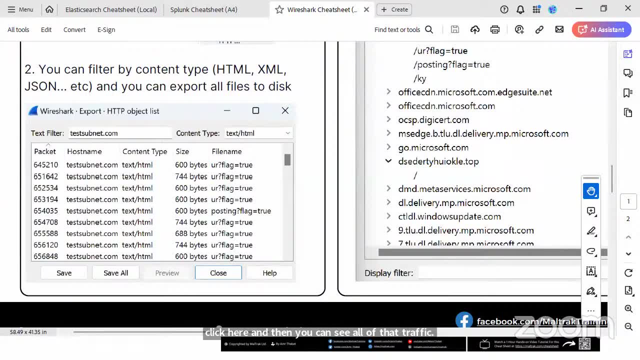 with pictures and stuff, File export objects, HTTP and basically click here and then you can see all of that traffic. Does that make sense for you guys? so far, Thumbs up. yes, That is one way I can investigate. So I can investigate the domain. 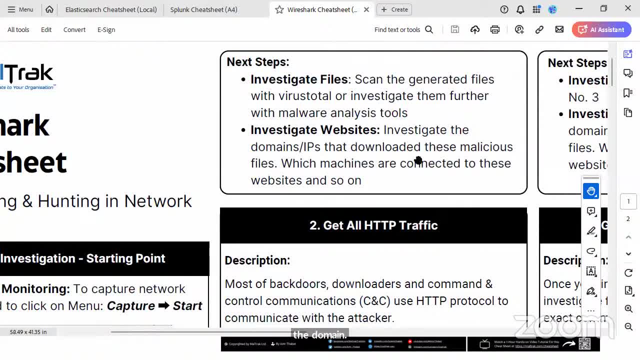 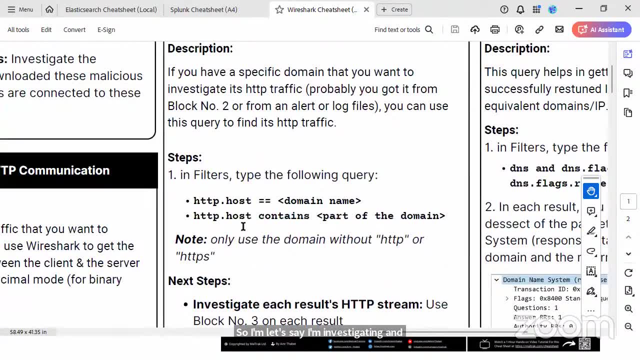 and then from the domain I find suspicious traffic. What's the next step after I find the domain? So I'm let's say I'm investigating a domain up here. I can investigate using that request, for example, And then, after I get the domain, information. 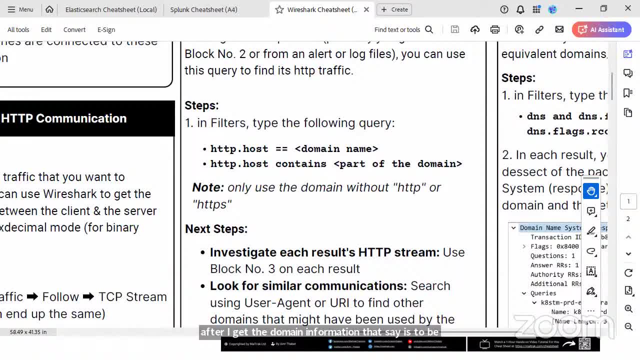 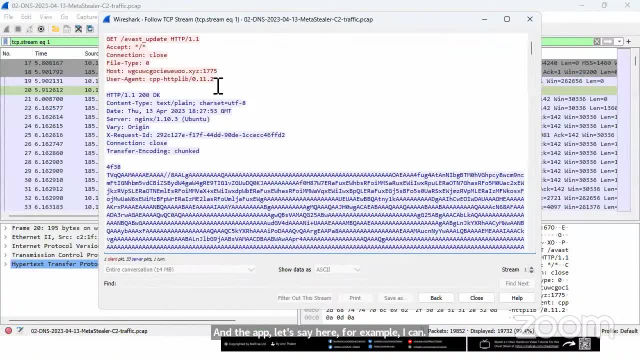 let's say htphost and then write that domain that we have in the app. let's say here, For example, I can follow the cp stream, I can copy the name of the domain, the whole thing, Just copy the whole thing here. 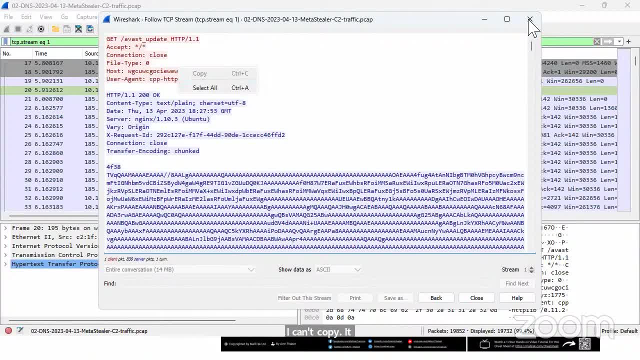 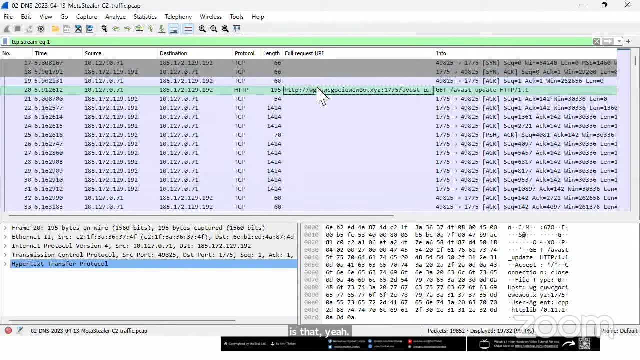 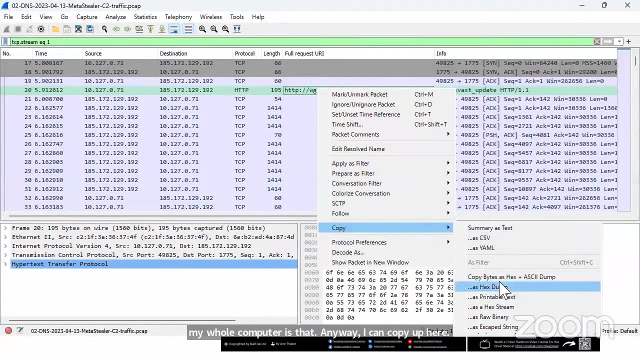 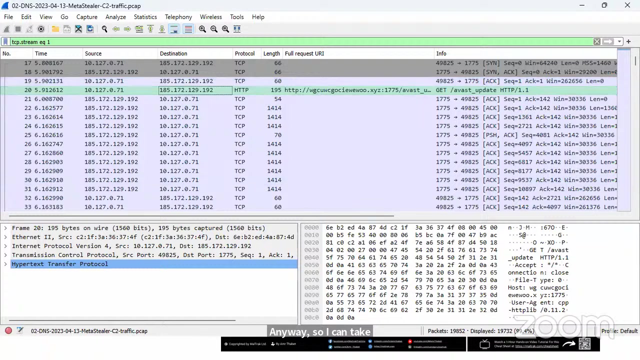 I can't copy. It doesn't copy. I think my whole computer is dead. yeah, Yeah, my whole computer is dead. Anyway, I can copy up here. I can copy, Anyway, so I can take that domain name and search for that domain name. 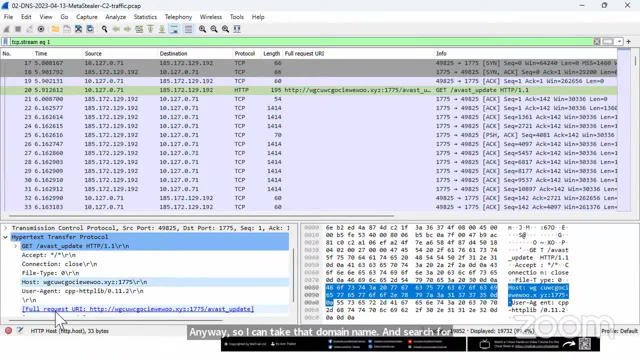 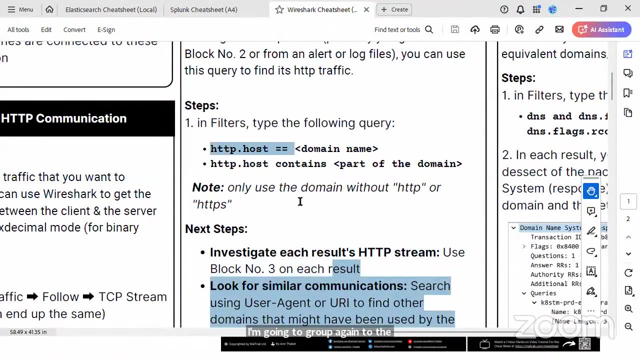 I can take it from here. actually, I can take that copy, copy the value and say: okay, this is the value. I'm going to go again to the Wireshark. I'm going to search up here. search for htp-traffic to specific domain. 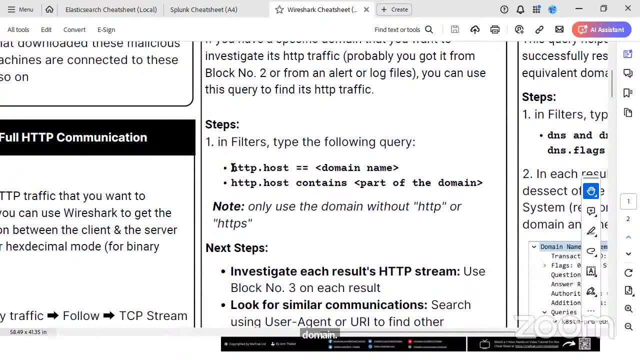 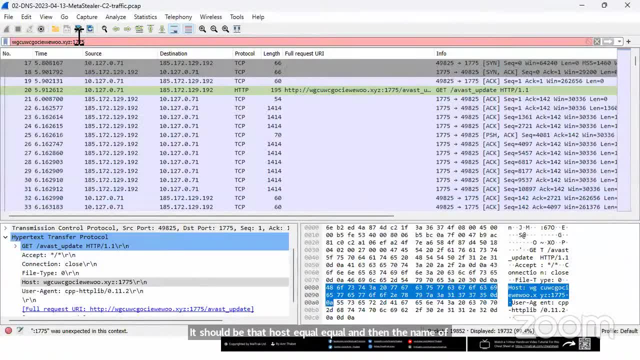 If you have a specific domain you want to investigate, follow these steps: Use htp-traffic, htphost, equal, equal and then the name of the domain. Sure, let's do that. So I will go to Wireshark and then host equal, equal. 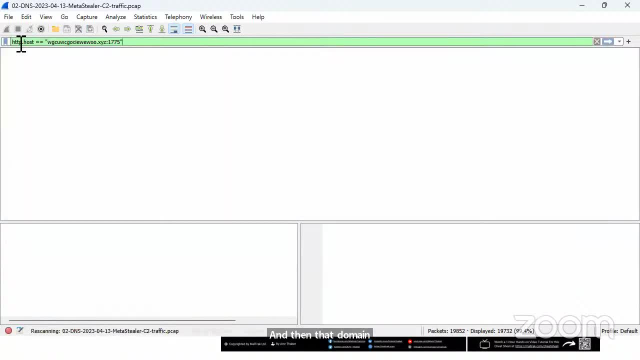 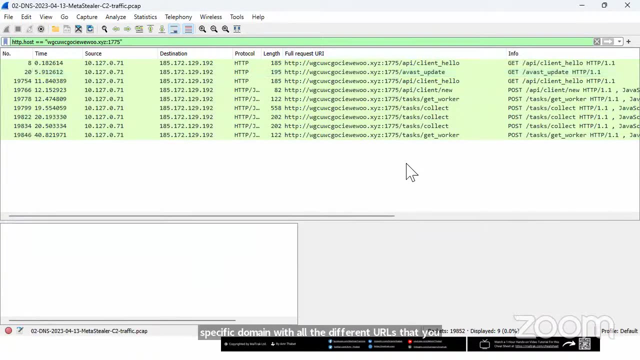 and then that domain with the IP and click enter. Now I have all the traffic. I have all the traffic to that specific domain with all the different URLs that you can see up here. Great How I can. so this I have done. 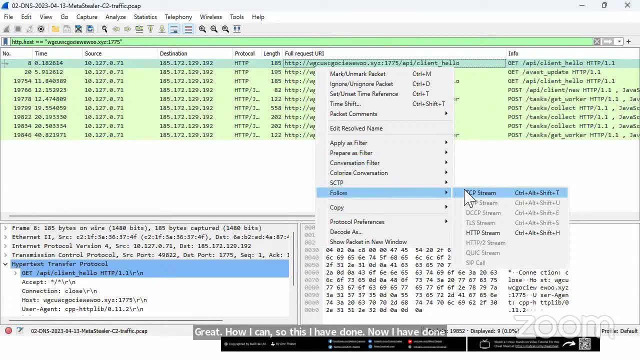 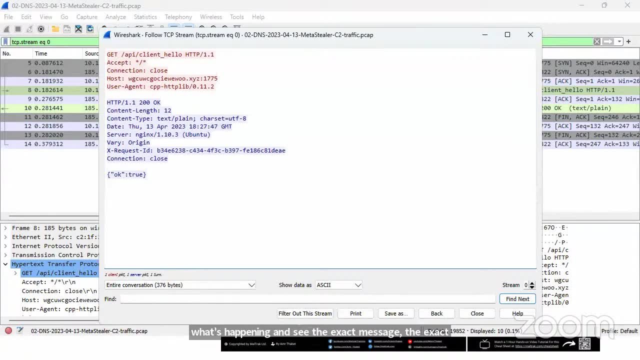 Now I have done the research and I can follow each stream, see exactly what's happening and see the exact message, the exact response, everything. What's next? Well, I can go back to the Wireshark cheat sheet and look at the next step. 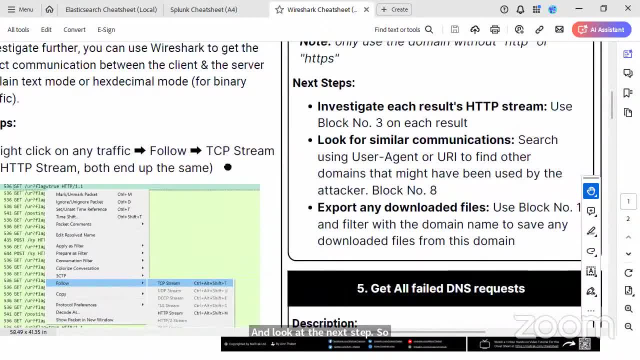 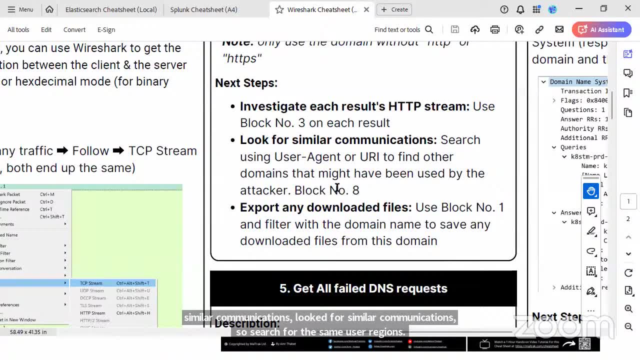 So investigating the full stream, like how we did follow TCP stream- look for similar communications. So search for the same user agents or the same URI and see if there's any other websites that he actually requested this. he actually sent the request with the same user agent. 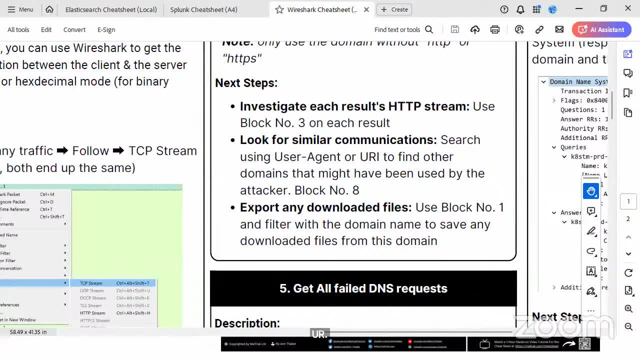 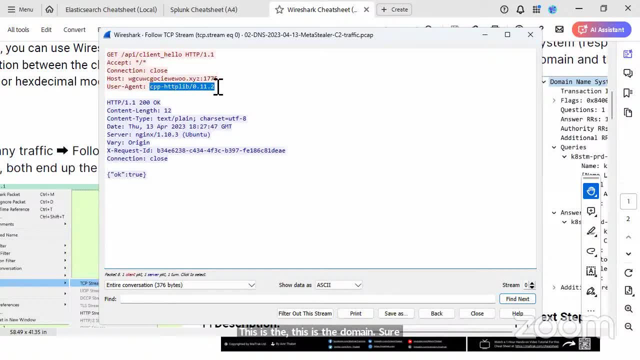 or the same URI. Let's look into that So we can go here. This is the domain, Sure, this is the user agent. that represents the browser that you're using. that represents that that I'm using. let's say here: 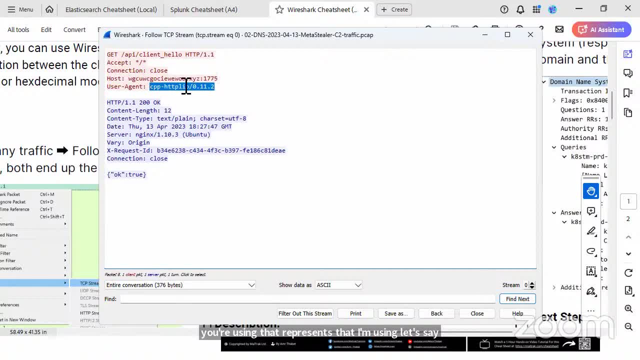 In this case it's using like a C++ H2B library. So that is, it's doing it from an H2B application, from a malware in C++ right? Sorry, a C++ application. If it's using Chrome, it's gonna have the word Chrome. 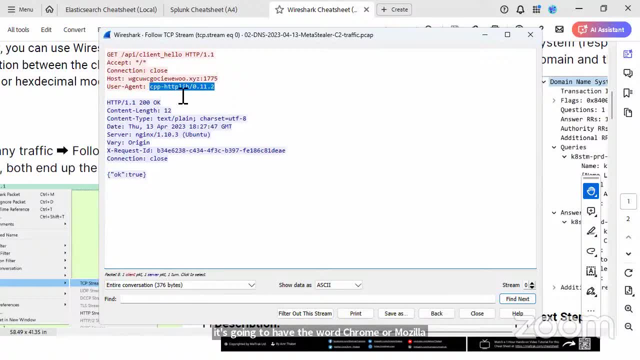 or Mozilla, something, something right. So the user agent represents the app that actually does the communication Here, for example, is that user agent? Probably, if we search for that user agent, we probably will only find the communications being done. 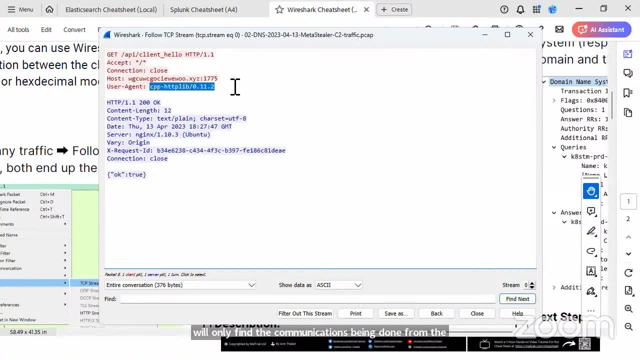 from this malware And probably we're gonna find a way to detect these attack. you know, to detect other domains that this user or this malware tried to connect to from the exact same malware. So we can search by that Or we can also search by the URI. 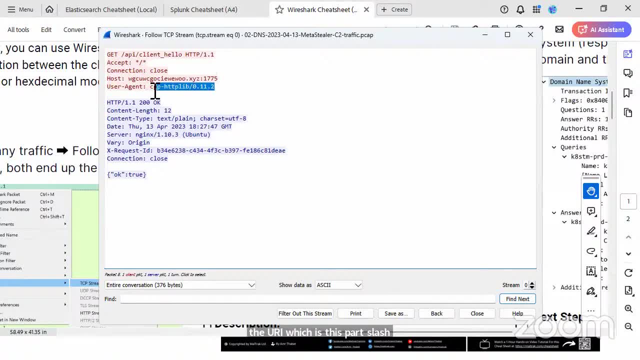 which is this app, slash API, slash client hello. Many cases when a malware connects to- tries to connect to- multiple domains is using the same URI with all the domains, So you can see that slash API, slash client hello is being sent to everyone. 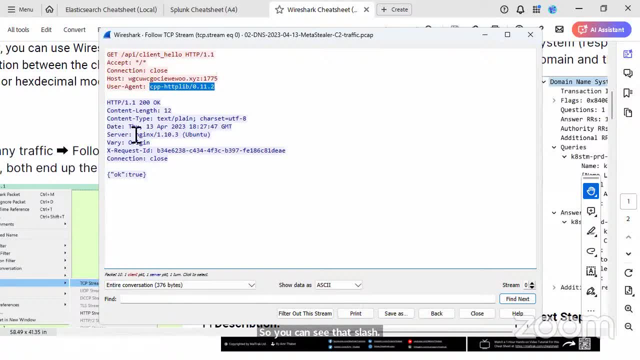 Not just to this domain. this is sent to multiple domains in the same machine. Or search through all the machines we have with the same URI and see if there's another malware. another machine is being infected and is connecting to a different domain using the exact same. 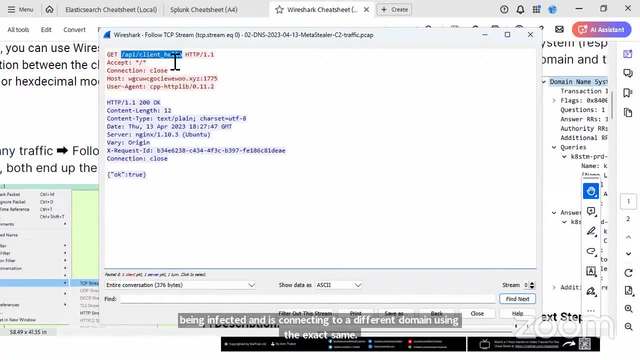 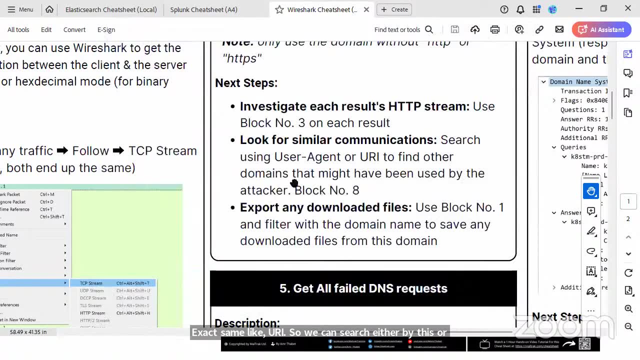 slash exact same like URI. So we can search either by this or that, which is good idea. And third is that we can also search by the IP. We can use the IP to search for more information, to search for other domains that use the same exact IP. 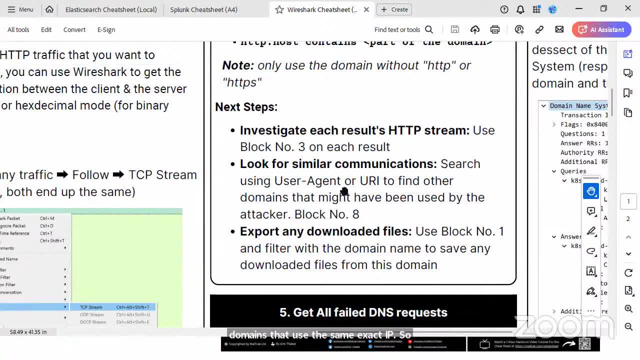 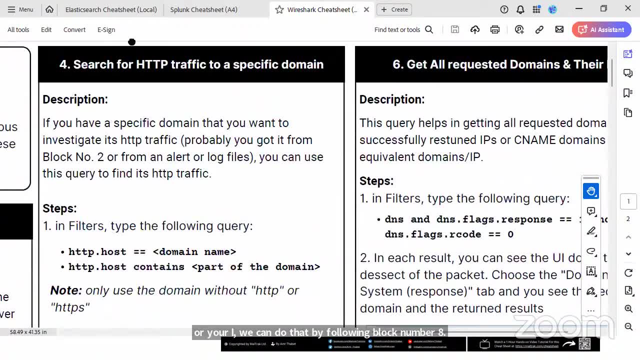 So let's try to do one of them. Let's look at so here we'll search through the user agent or URI. We can do that by following block number eight. This is block number four. six here, five, seven, Okay, so eight is the next page. 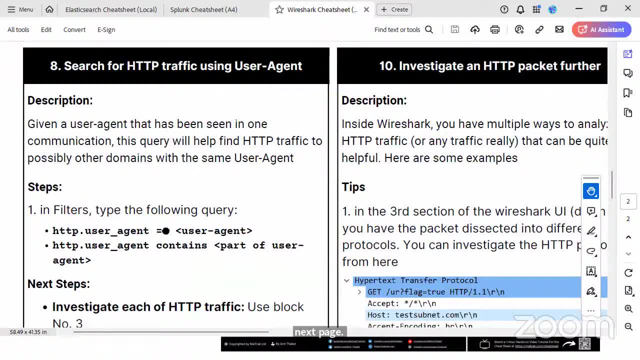 And this is number eight: H2Buseragent equal, equal, the user agent. So let's do that, Let's select that up here. Let's say: okay, let's go to Wireshark first, Close that To Wireshark. 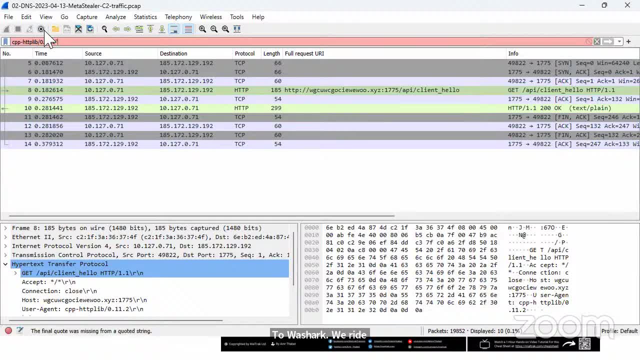 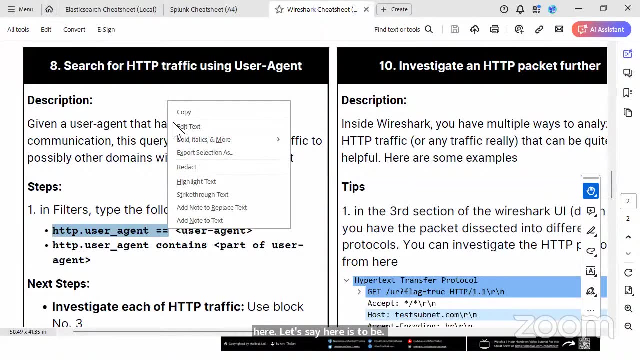 We write first the user agent. This is the user agent, And now we are going to take the exact command from here. Let's say here: H2Buseragent- equal, equal. We're going to take that copy and then go to Wireshark and paste that. 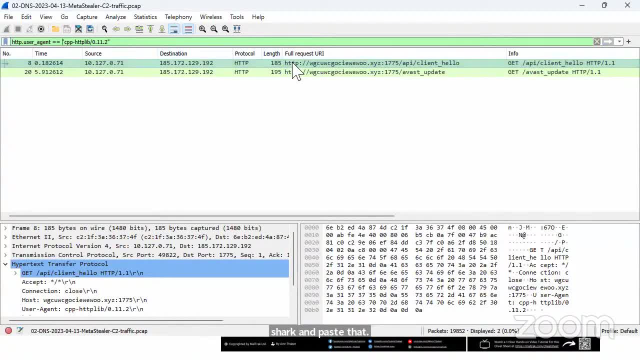 So now we can search for the user agent, And now we have. luckily, we have only the communication to this domain that uses that user agent, But nothing else. So this user agent hasn't been used by other domains. We didn't discover new attacks. 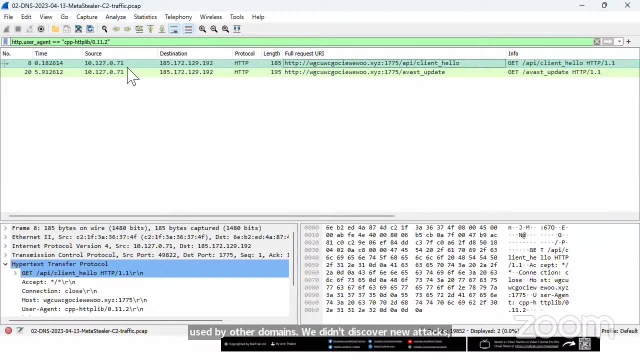 but that was something. we could have found other domains. We can search by the IP As well. we can search by the slash API, slash client, hello. We can search by any of these stuff So far make sense And with Wireshark we can here, for example, let's in this: 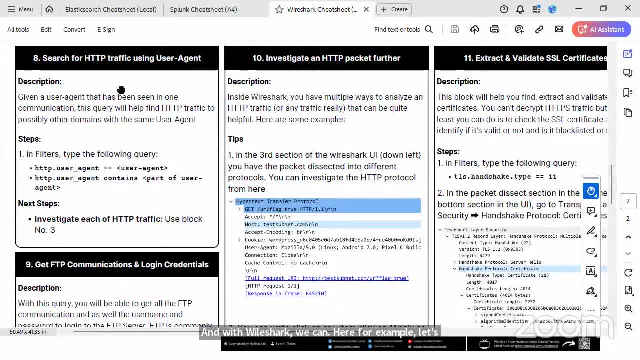 and with Wireshark. we can here, for example, let's in this, and with Wireshark, we can here, for example, let's in this: investigate the traffic much deeper. This is the next step here. 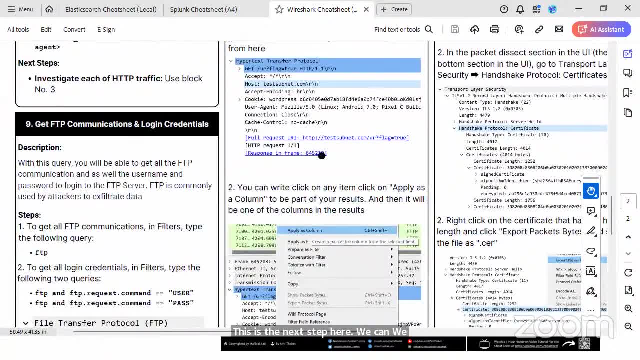 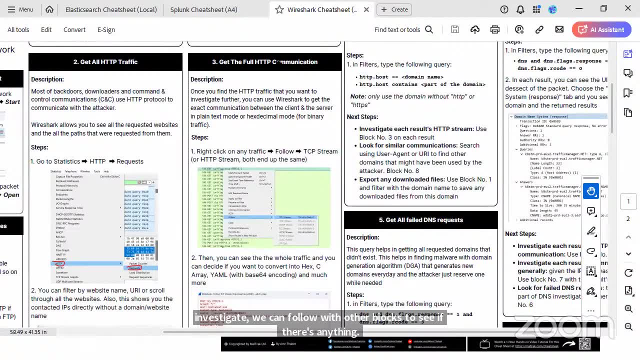 We can also investigate, we can follow with other blocks to see if there's anything else we can find, Like let's say get the full H2B or let's say get all the H2B traffic. We can follow again with that. 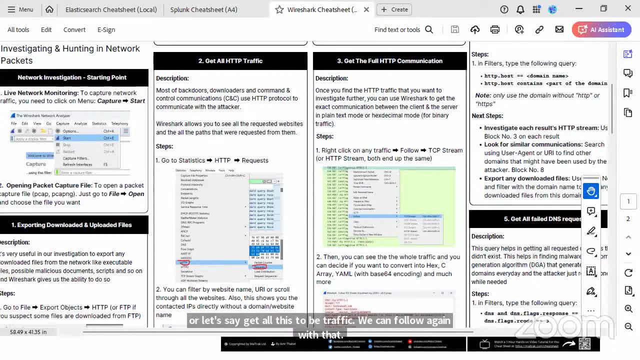 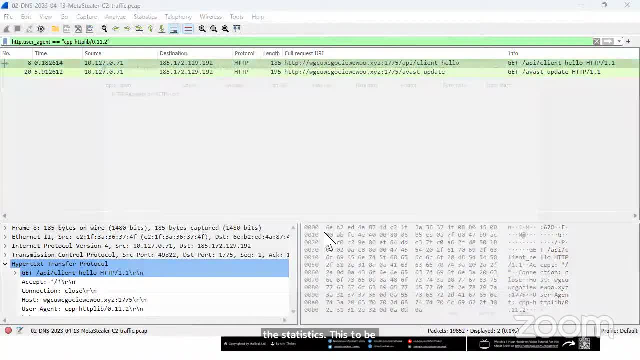 Since this is H2B requests, you can go to Wireshark, go to the statistics H2B and then requests, and you can get all the different H2B requests that's been done on this bcap file, just in a list like that. 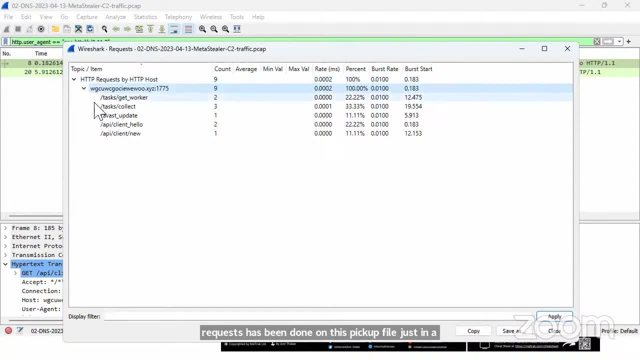 And you can see, okay, there's only one domain we find in this bcap file And in this one domain we have find these five different requests, different URIs that have been requested. The whole communication- this is statistics- allows you to really find. 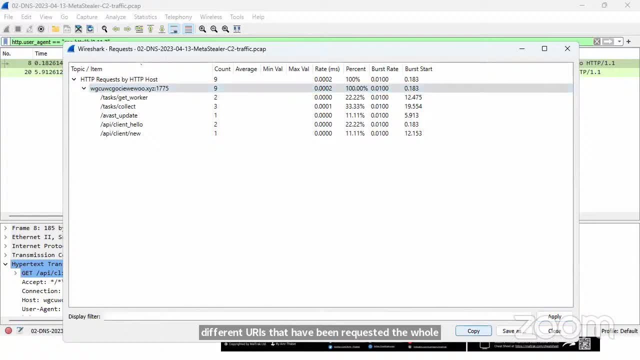 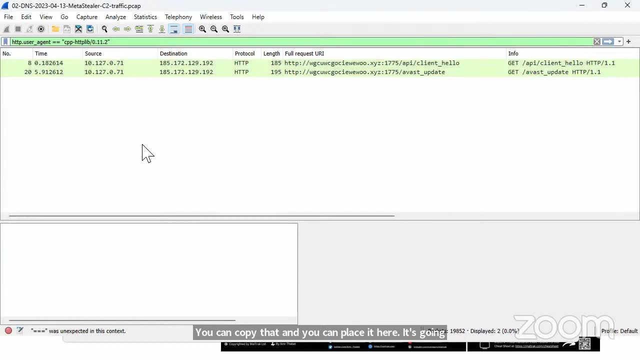 and nail down exactly what you're looking for. You can copy that and you can paste it here. It's gonna be super long, But you can paste it somewhere. take some domains and start searching for that. You can filter them out in a different tool. 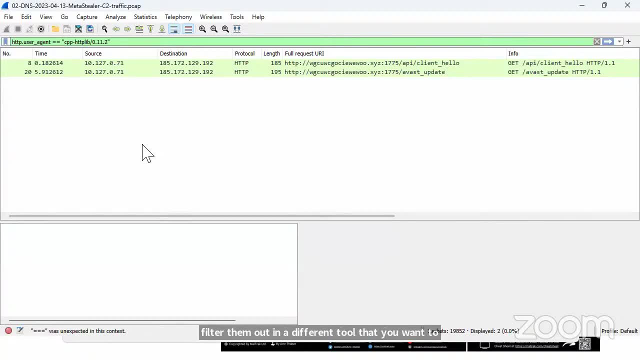 that you want to use as a search or something like that. So far, so good. Did anybody learn something new so far? Anybody has learned anything new? Yes, sure, great, So very good question. So awesome, yes, for sure, yes, very good. 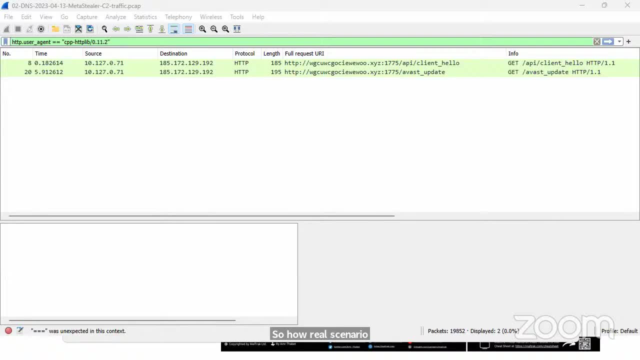 So how real scenario the SOC team can get the bcap file. Mostly there is. mostly you will not get the bcap file. You mostly have either, let's say, Wireshark reports or something like: sorry, not Wireshark. 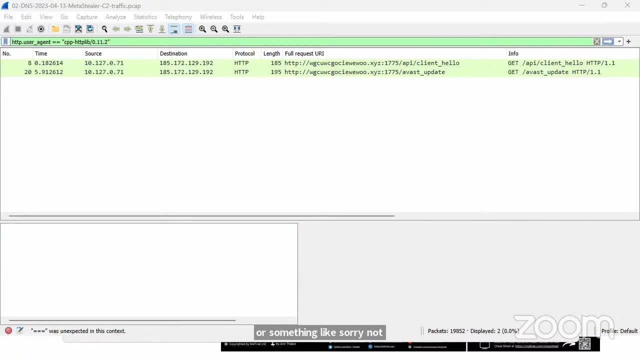 but Zik logs, for example, or RDS, IPS logs. Some tools like, let's say, tools like NDRs, like Network Detection Response, can store small bcap files for some suspicious activities And that basically can help. 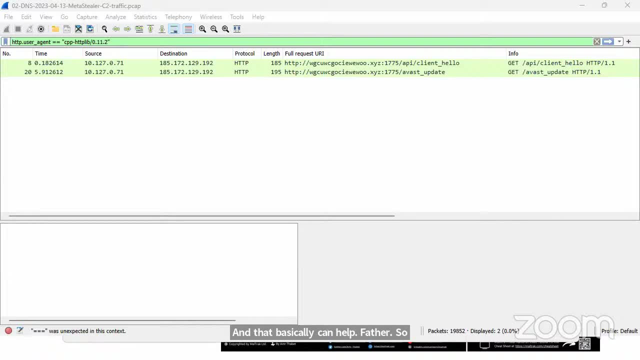 Pardon. So it basically sorry, My train of thought has gone. So basically either you have Zik logs or stuff like that, or you have an NDRs that actually takes bcap of suspicious activities and you can download these bcap files and analyze them further. 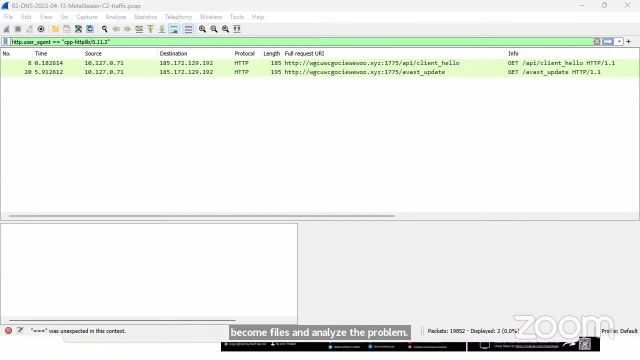 That depends on the system you have. Some expensive systems do have the ability to take bcap files or they already take bcap files of suspicious activities. In many cases not, But some things can apply on logs and we're gonna look into that. 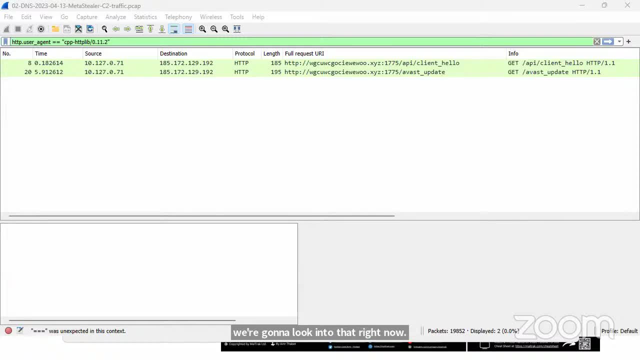 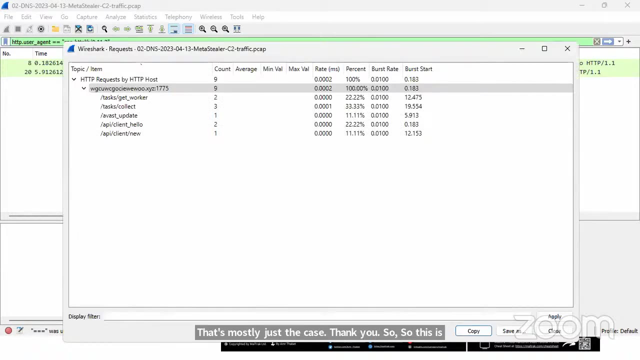 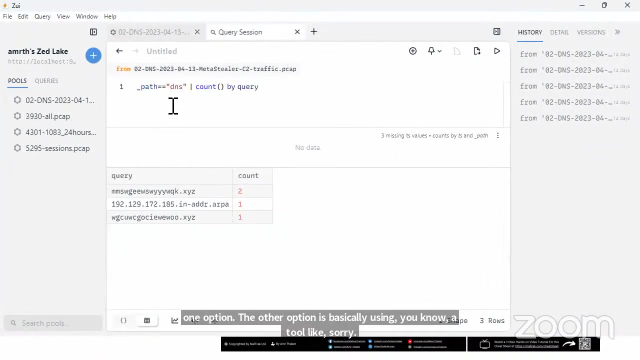 right now. so, um, we'll get filtered files and pre-analyze from some sim tools and get it to get to analyze it. that's mostly, yes, the case. uh, thank you. uh, so this is one option. the other option is basically using, um, you know, a tool like sorry, a tool like um zoe. zoe is a tool that is. 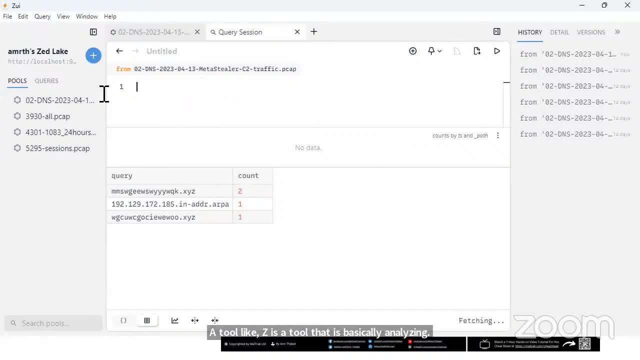 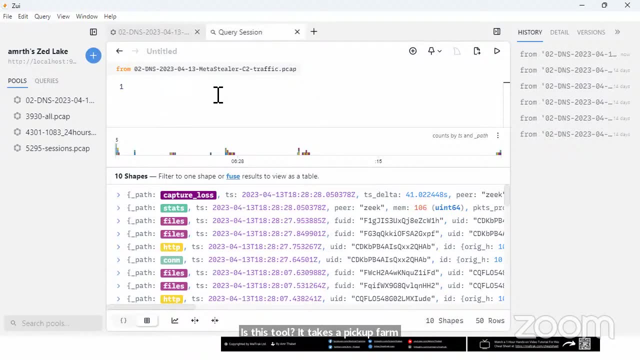 basically analyzing- let's start from the beginning- is this tool. it takes a bcap file and it converted into zig logs. many companies, or some companies do, have zig installed. that basically takes a copy of all the network traffic and convert it into logs where we can analyze and they convert it into. 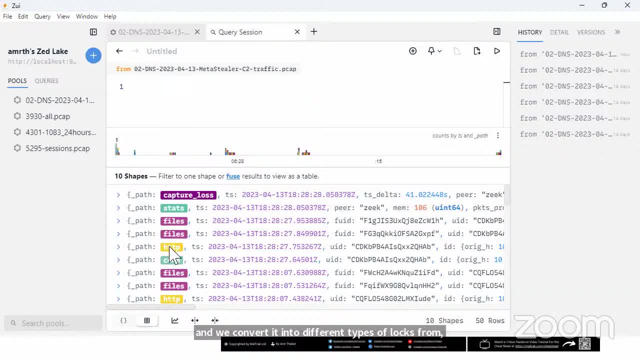 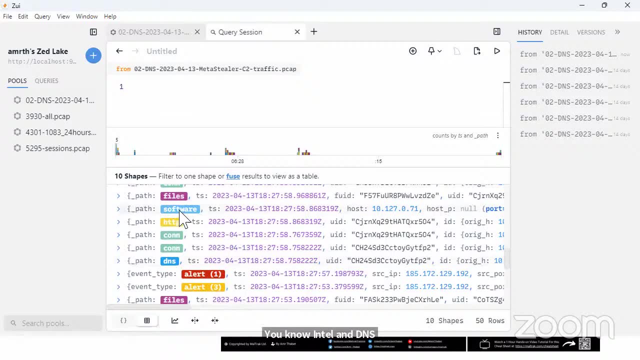 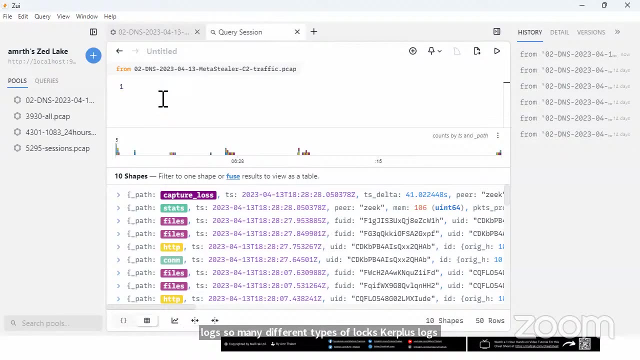 different types of logs from: uh you know, from stats files, hdb connections, um you know intel m dns logs, uh software logs, um you know, ssl logs. so many different types of logs. kerberos logs everything and you can investigate these logs farther to detect suspicious activities. so you can basically say: well, in this case, for example, i want to look for any dns logs. 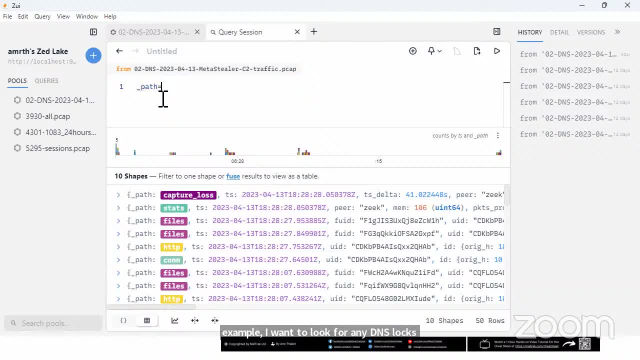 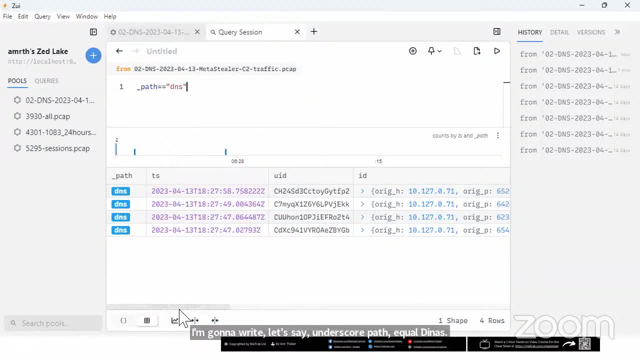 so i'm going to write, let's say, underscore: path: equal, equal dns, and i'm going to get all the DNS activities that have happened on the system. So in DNS requests, let's say: here we can see that domain that we already have, We can see that there's another domain that we have. 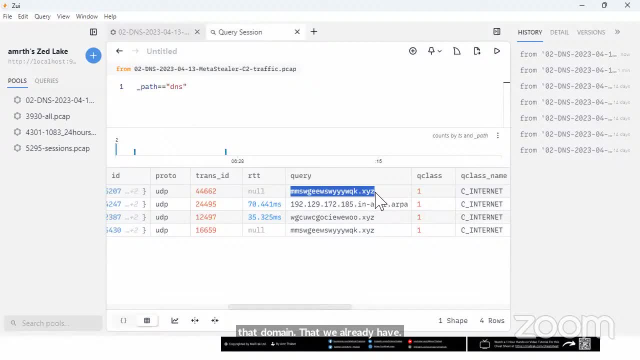 found that we were able to get up here. This domain is basically a new domain. That is not really the domain we have found. to all of our analysis, We found it in the DNS requests and basically this DNS request did not really come up with an IP. 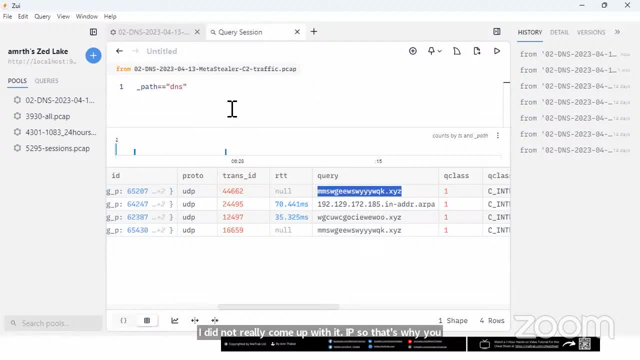 So that's why he didn't connect to it. So we found two different domains. We can even filter that out even more and use something like this: Okay, I want to get the count of all the queries. or let's say: 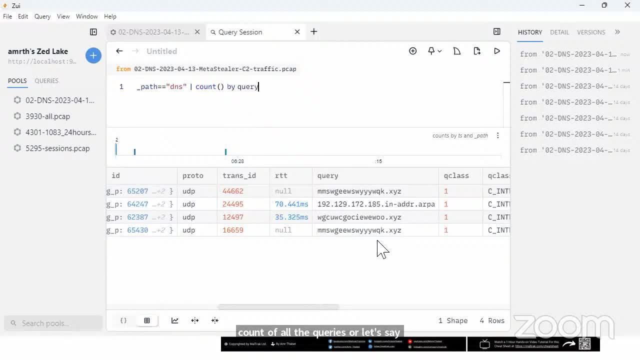 count by query, which I want to get a table of all the different queries and how each one of them appear, how many times each one of them appear. It looks like a same tool. You can do the same in Splunk or any data analysis tool. 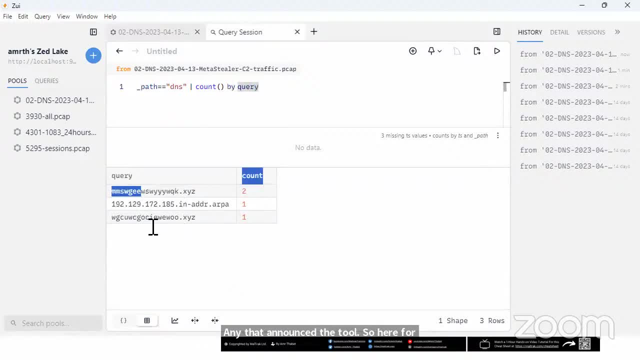 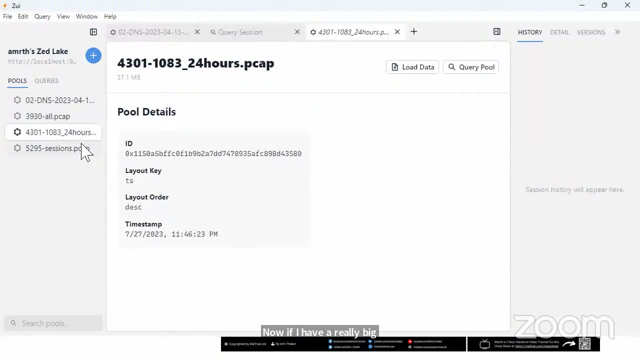 So here, for example, you can say: okay, I have found these three domains. Now if I have a really big file, let's say really big backup file, or you just have like let's say, I want to query tool, and let's say 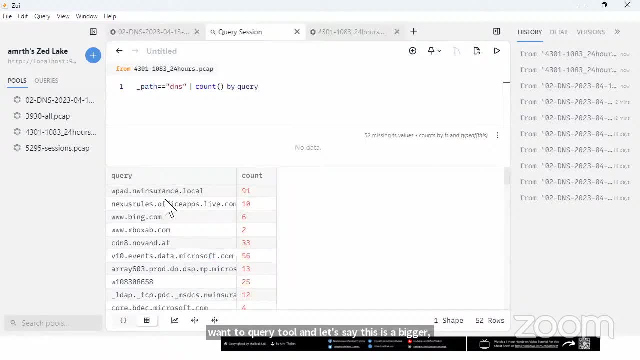 this is a bigger backup file. I can do the same and I can find all the different domains up here. So if you are analyzing a backup file that's really large, you can use something like that, or you can if your company have Z-clocks. 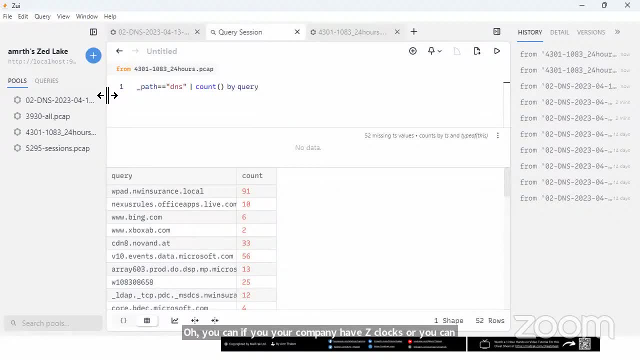 or you can actually add Z-clocks. you can use the same Z-clocks to investigate further different attacks and find suspicious activities. So how to deal with Z-clocks? I have a lot of questions. Let me get to the questions Just a minute. 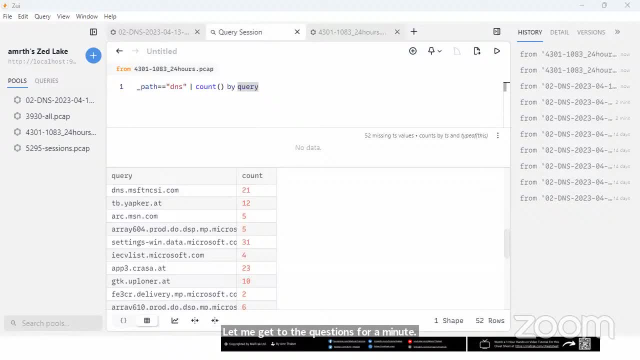 Just, I don't want to forget you guys. So so is SOC collecting all the log files from any time. So SOC team collects all the log files anytime. It wouldn't be the team, it will be the tools. So you will have tools installed. 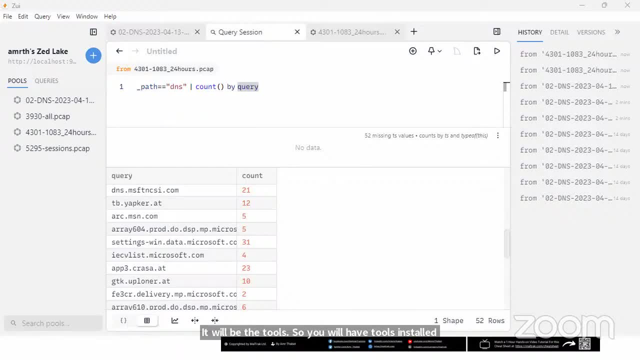 that collects logs all the time. Let's say that is, you have Z-c installed, you have, you have, let's say, Firewall logs, DNS logs, IDS, IPS- all of these softwares being installed in your system. 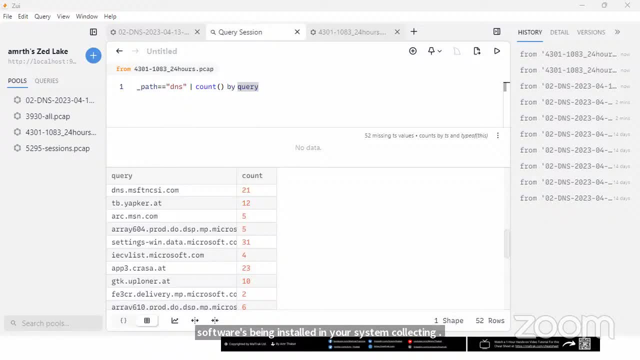 collecting logs, And the SOC team are basically the one looking at the logs and investigating them further, looking for alerts and all of this stuff. But it is the. it's not your job as a SOC analyst to collect logs. It's your. your job is to analyze logs. 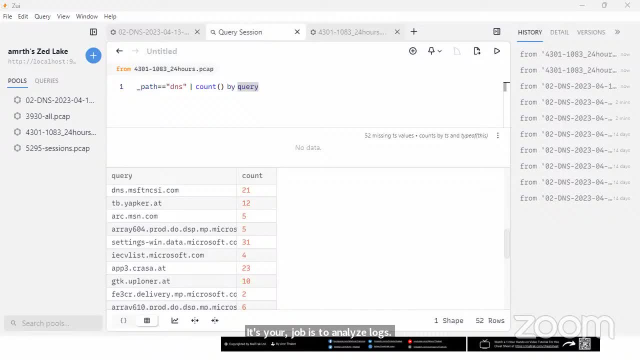 Makes sense. So so there is a question and there's a reply to that question, So let me read both. Is there a way, if we can use AI to do all of this? AI is already implemented on many modern SIEM tools. 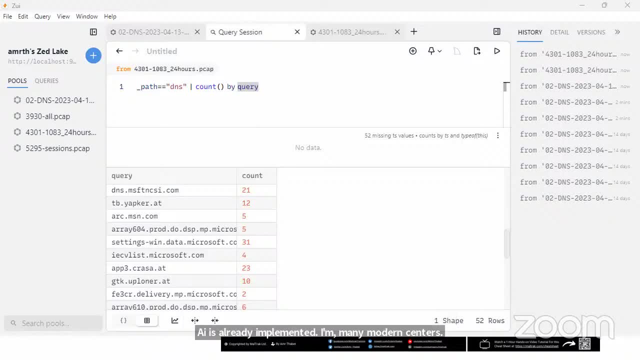 It's important to learn what's the process behind and why you are doing something. Any tool is not magic. It can make false, negatives or positives. That's why we need to know the manual process. take all the techniques to understand the process of analyzing. 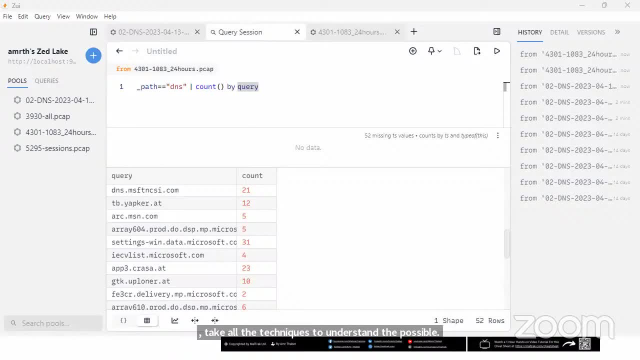 That's definitely sure, And also it's good to feel, okay, AI can do all of this. AI can do all of this stuff. AI can do all of this stuff, It can automate everything. But there is there's really important AI of a SOC analyst. 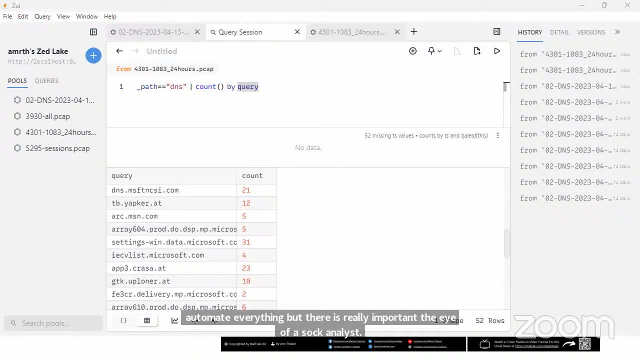 And, at the end of the day, AI can automate crappy work, but it cannot automate a really professional like top tier SOC analyst, because he'd be able to spot stuff that AI won't be able to spot. He will be able to understand attacks. 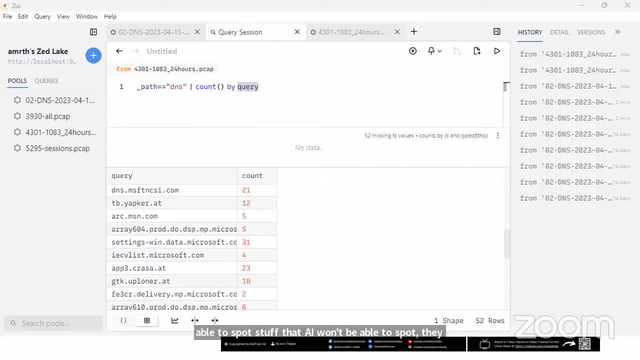 because the attackers are still humans, right, So they are doing stuff that are that are new- new attacks, new techniques, new ways of hiding- And this needs people also with creativity and really smart that can detect this stuff. AI can automate things. it's already known. 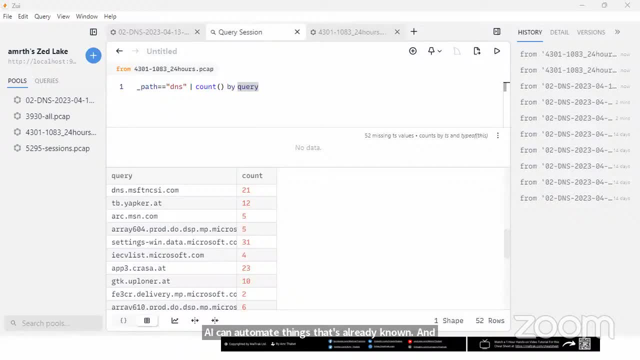 and can and can basically go through this whole process, And AI needs to also maintain between being being smart and being fast And both. you cannot really have both together, So AI wouldn't be really the top notch in most of things. 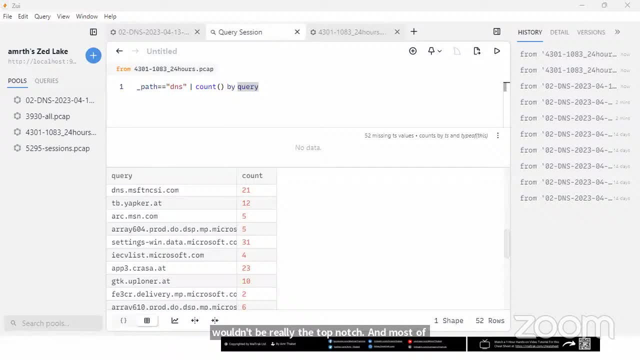 You need the SOC, You need the team to really investigate attacks deeper and farther than ever. That's the only way you can actually get stuff. Maybe I can help to authorize, filter out some stuff, or show you know, or or, let's say, add more context. 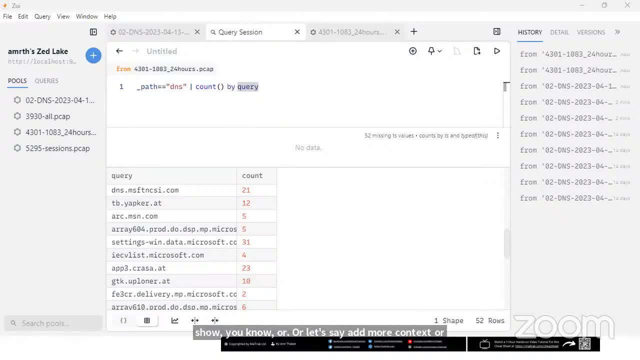 or add his own filters, but he's not able to replace, you know, the human. if that makes sense, And also attackers might use AI as well. So that's, that's, that's the. that's the, that's the key. 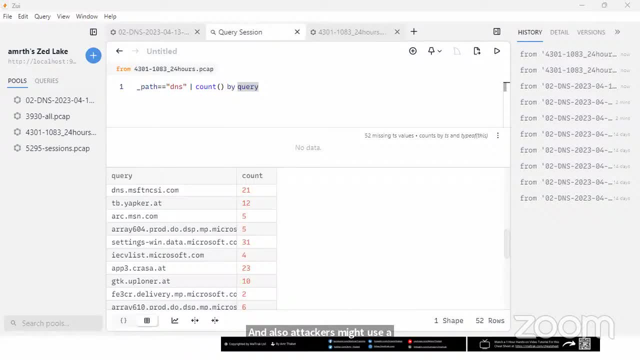 And the other thing that I want to talk about is- and I want to talk about is Zik logs for backup generation, And that's what I do. So a Zui or or or a Zik logs are basically logs generated from traffic network traffic. 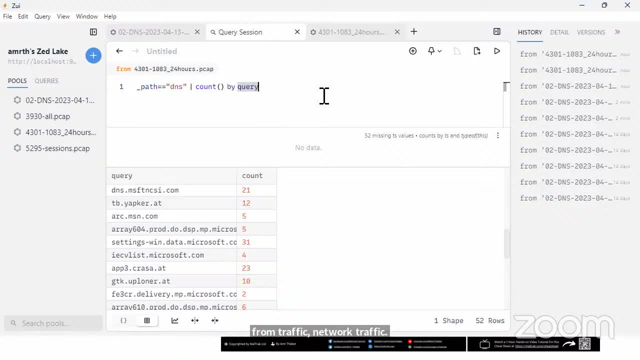 You can generate it from a backup file or from live traffic. Zik is mostly created to generate it from live traffic. Zui is a is an app that you can upload a backup file and it will run Z Zik on it. 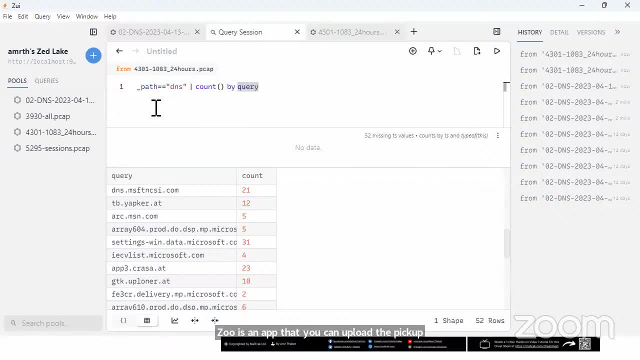 And it's going to convert it into into, into, into into into Zik logs. So this is from a backup file, but also you can have the similar logs from, let's say, from a real traffic. Also, Zui is using a specific language called Z. 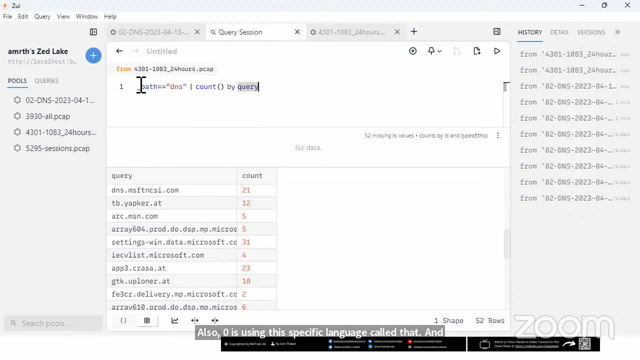 And this language is. you know, it's only. it's really. it's a kind of like a SIM tool, but this language is. you don't need to learn it. really, You don't need to use this app, you can just export. 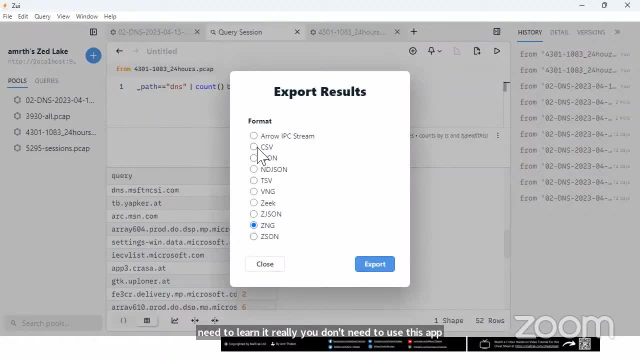 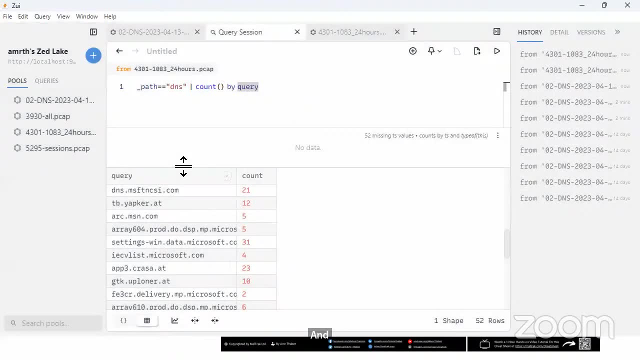 all of this traffic. export all the results into see Zui into JSON file and analyze it by by using Splunk or something like that. Does that make sense So you can investigate further using something like Zui We actually have here in Splunk cheat sheet. 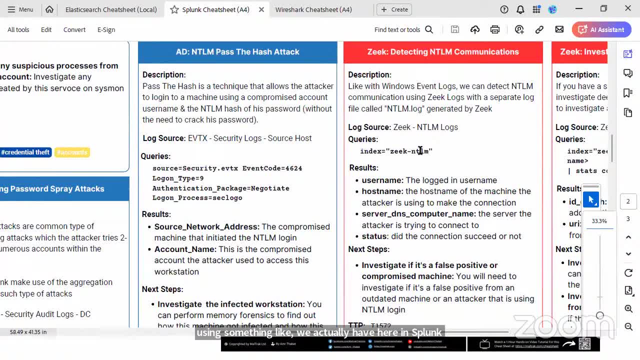 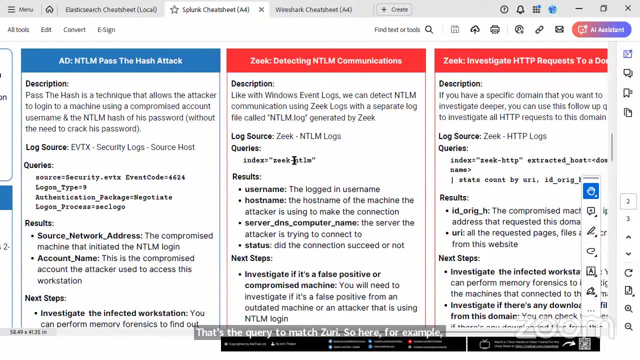 a way to use these logs. let's say, for example: but that's on Splunk, but you can apply the same things on on something like Zui, just change the query to match Zui. so here, for example, detecting NTLM communication. 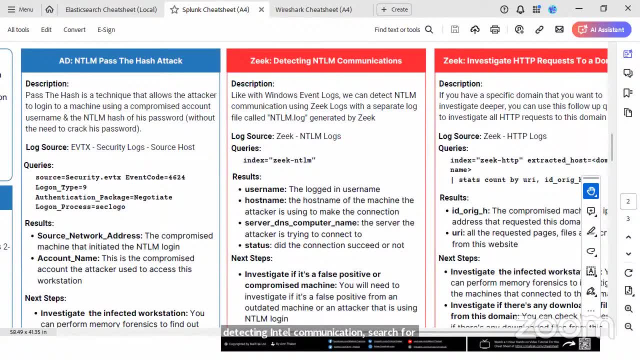 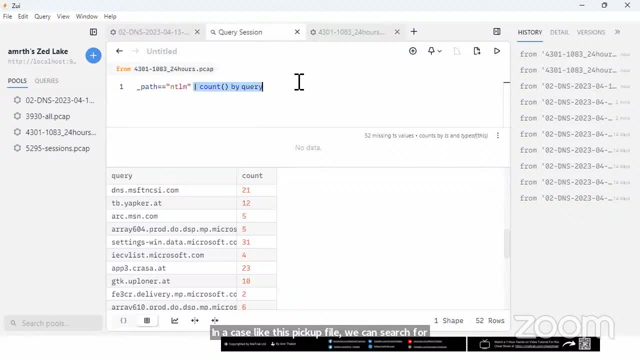 search for NTLM, for example. We can do that in our backup file So we can go to our- sorry, not the backup, the Zui, For example in the. in a case like this backup file, we can search for NTLM and look for any NTLM communication. 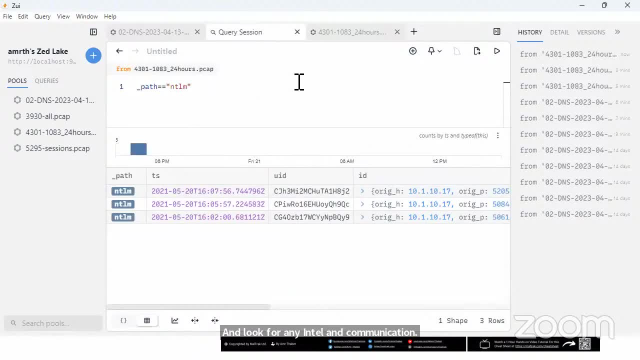 So if you don't know what's NTLM, NTLM represents an kind of an obsolete type of of protocol to log in and to log out and all of that like authentication- sorry, yeah, authentication protocol And and NTLM is kind of obsolete. 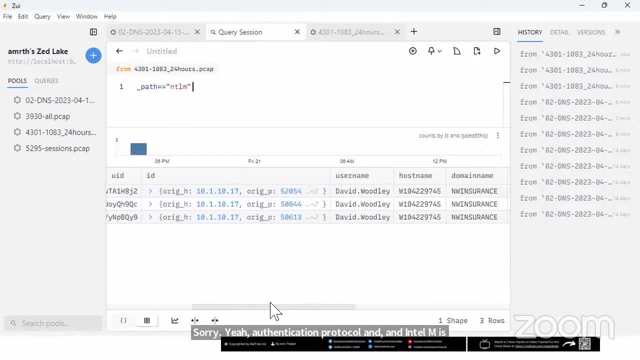 So it's rarely to see it in real traffic And many cases it's going to be used to as a as a way to escalate privilege or to to use pass the hash attack, which is a known attack. So there's big, many cases where this attack 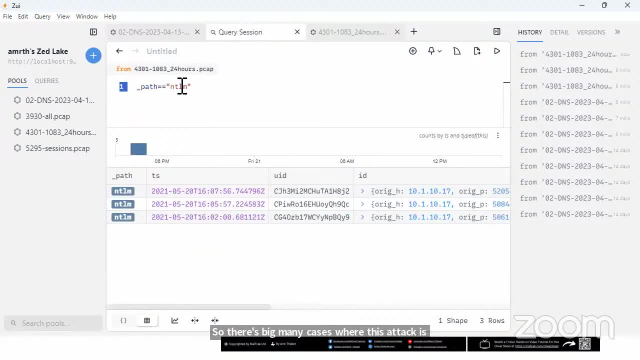 is pass the hash attack. We can see here that we, if we search for path NTLM, we can see that we have found multiple cases with a specific user. We can investigate that further and see how did that happen. Who is that guy? 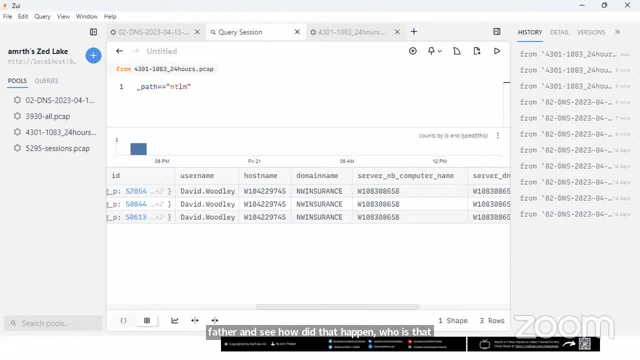 Who is attacking? blah, blah blah. So we can use. we have strong logs that we can use it to investigate attack further in this way And we can go through different ideas. So here, for example, we found some attacks, So what's the next attack? 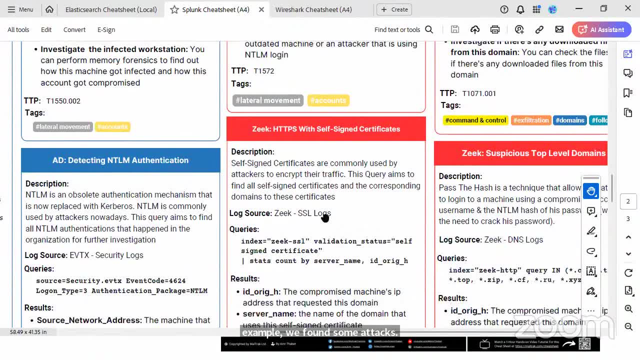 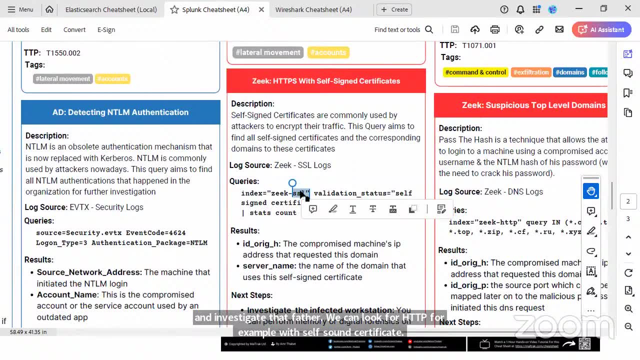 We can go back to the index, investigate it- If it's a false positive- and investigate the problem. We can look for HTTP, for example with self-sign certificate. We can do that by looking at the SSL traffic in the inside ZOE and look if validation status. 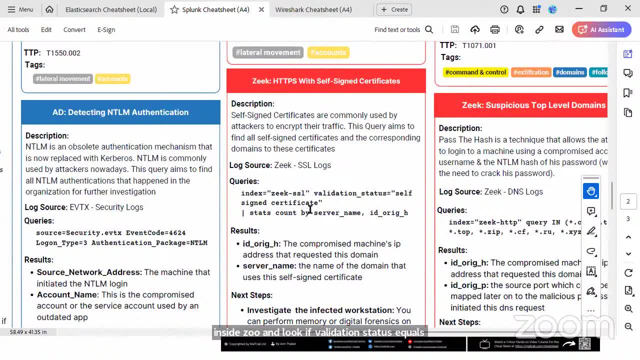 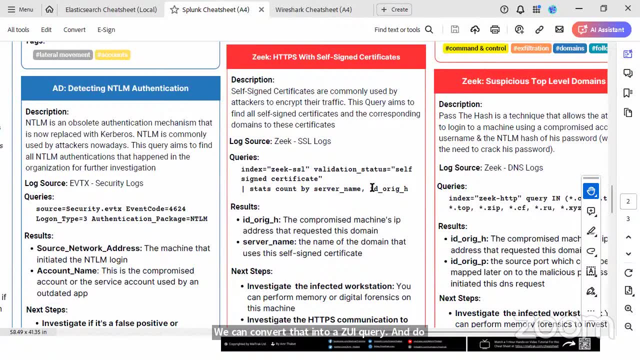 equals self-sign certificate, And then we can get all the information about. We can convert that into a ZOE query and do the same, Or we can just upload all the log files on Splunk, Otherwise it's Splunk. any questions so far? 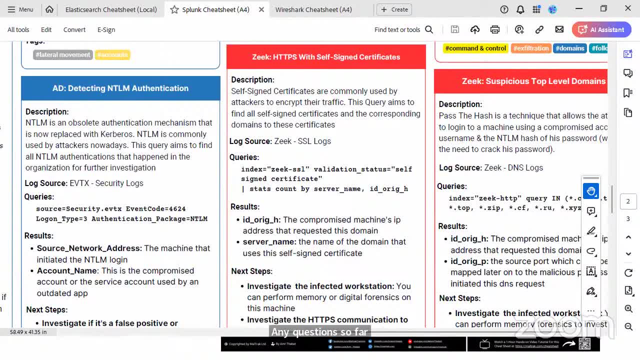 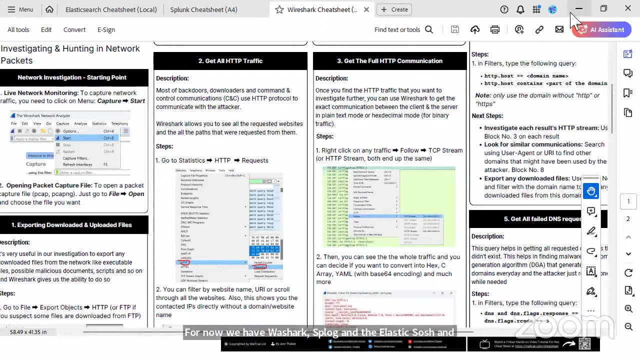 we are working on Sentinel, but I can promise it's going to be soon. but we are working on having a Sentinel as well- cheat sheet later on. for now we have Wireshark, Splunk and Elasticsearch and yeah, so that is what we have so far, any. 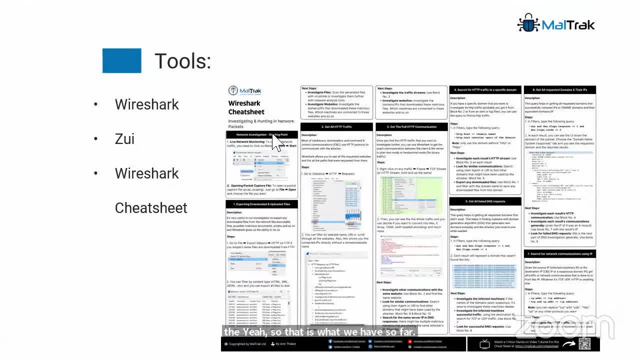 questions. guys, I know we are over the time, but if you guys give me 10 minutes, I want to share with you something really important. I have been working behind the scenes for a training that's going to come up this weekend. it's called let's analyze a cyber security. 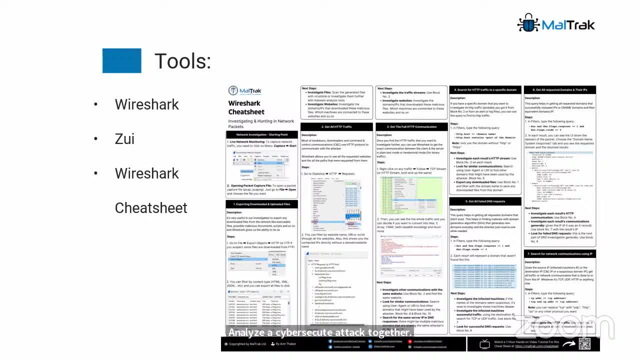 attack together. this is a small demo. what we're going to do very, very small demo, like super small demo. and here we just looked at this Wireshark bcaps and what they can do. we only had like 10-15 minutes. sorry, a little bit sick, but yeah. 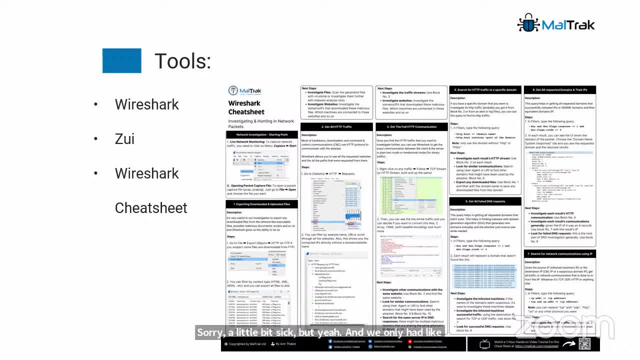 and we only had like 10-15 minutes to analyze a full attack. but what we're going to do for two days is that we're going to take a full cyber security attack. we're going to investigate the attack through three different processes. one is looking at 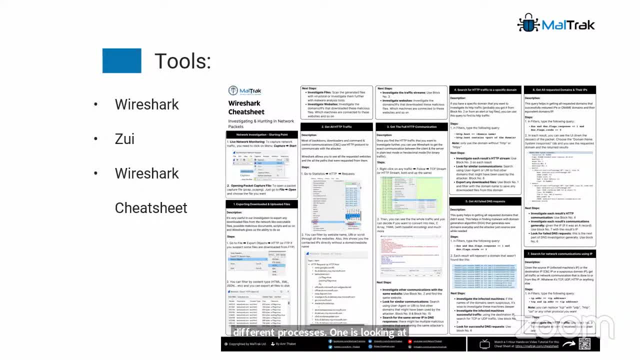 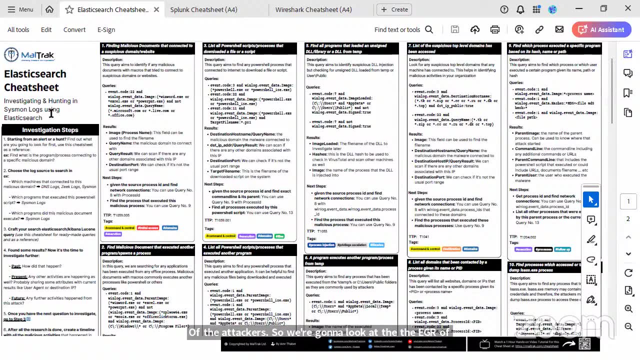 the behavior of the attacker. so we're going to look at the EDR or the sysmon behavior. so what's happening on the machine itself? we're going to investigate different machines. so we're going to have a full attack, a full cyber security attack on different machines, different servers. 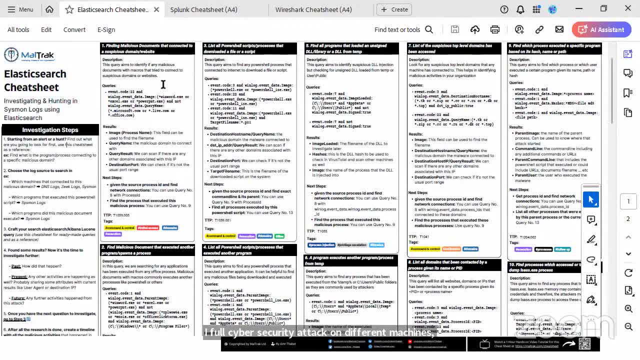 and we're going to investigate the sysmon logs in Splunk. we're not going to use Elasticsearch, we're going to use Splunk in that investigation. so we're going to analyze the attack on Splunk. that's one part we're going to look into. 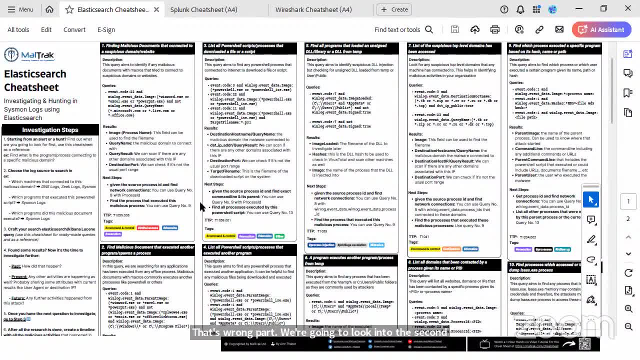 the second part we're going to look into is the bcap files. we're going to analyze the bcap files in Zowie and in in Wireshark and we're going to investigate that further, see what's happening on the network. so we're going to see what's going to. 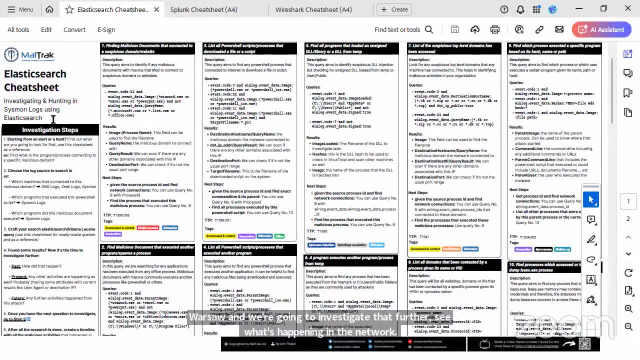 happen on the here, on the, on the host machine? what's going to happen on the bcap file? what is how the attack, the whole attack happened, the identity behavior as well, if there's any pass, the hash attack in the brevis escalation. all of this and we're going. 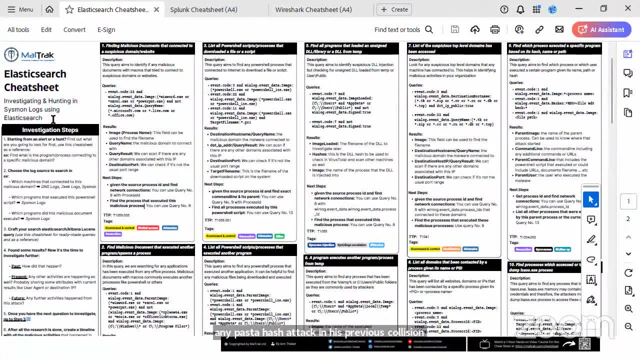 to draw the whole attack, how the attack happened from A to Z. we're going to look into. we're going to look into how, the, how, the how the attack started and what's the and basically we're going to investigate it step by step until we have a full map of how the attack happened through. 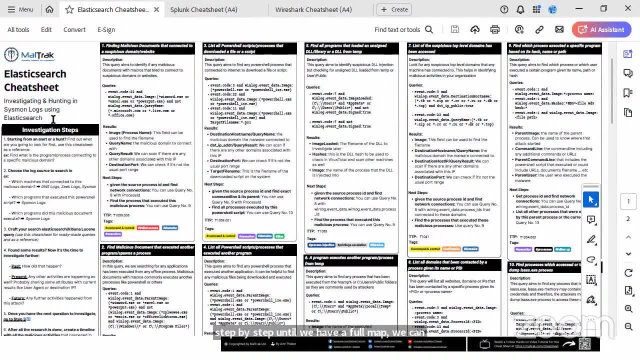 our different machines until he took over the whole domain and we'll be able to take over the, will be able to understand the full attack and prepare a report about it. we're going to help you guys create your own first blog in your own blog. let's say mediumcom or something like that. how? 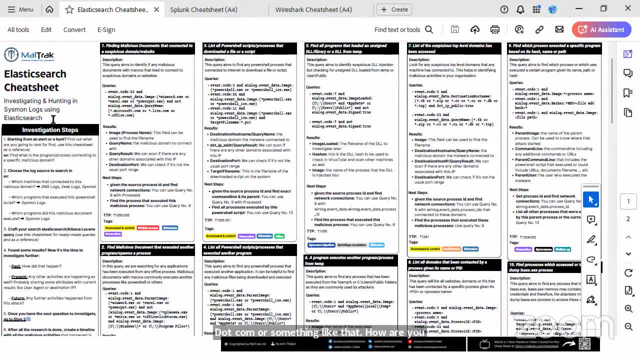 you're going to share this attack, so you're going to analyze the attack with me on on this zoom training. it's going to be nine hours, so it's not going to be 15, 20 minutes like now. it's going to be nine hours. no more of theory or no more talking about, like, how to land a job. do this, they're going. 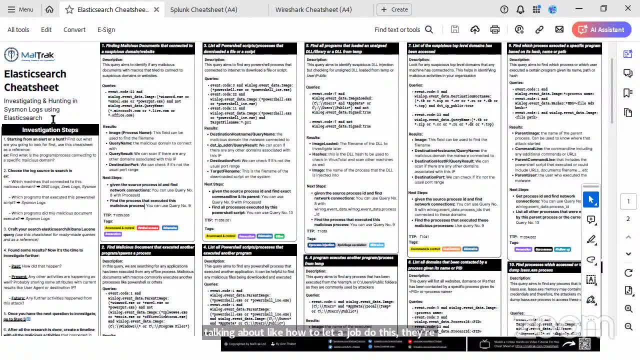 to be very, very focused on the attack and i'm going to analyze it together. so you're going to have extra samples or cheat sheets and you're going to analyze the attack with me and throughout the two to two days, you're going to analyze the- the system logs- and analyze the- the network. 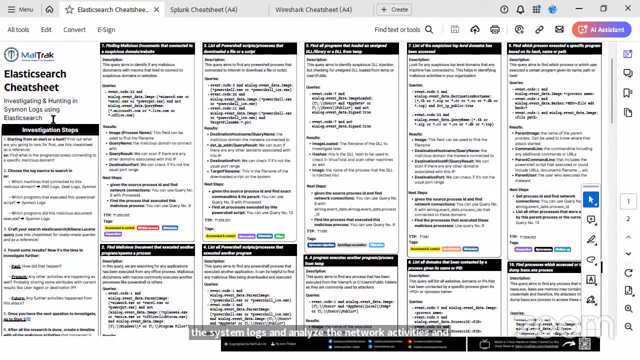 activities and you're going to start writing your own block. maybe you're going to have multiple parts of this block, but you're going to write your first block. you're going to review different blocks together and then you're going to share that on your linkedin or in your resume. we're 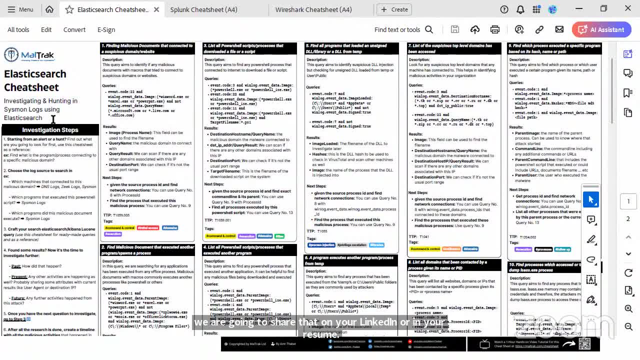 going to talk about how you can do that and, out of these two days, the main goal for me is that you have your own analysis of a full attack. you have your the, the draft of your first block, and you're about to share a blog that shows you as more professional. 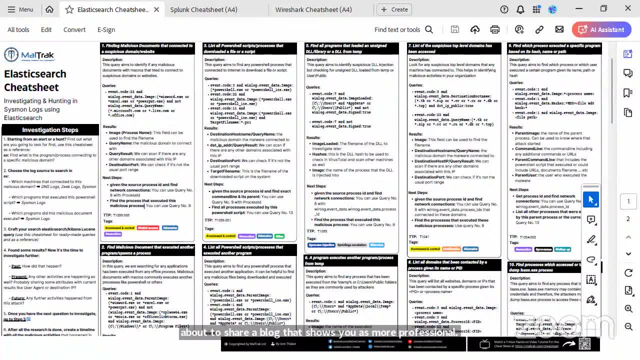 in the field and you're able to take that block and basically, um, you're able to take that block, share it in your linkedin, share it in your resume and hopefully you can get an interview from that, get your first job offer or, if you are already in SOC, this helps you to practice on investigation. 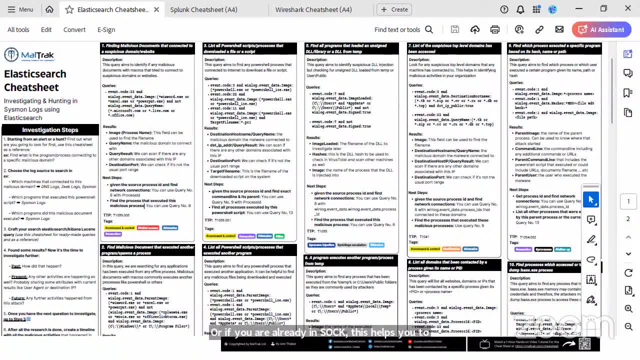 in the instant response process and get to the next step. if that is what you're looking for, does that make sense for you guys? so is that something you're interested in for you guys, thumbs up. if that's something you're looking for, only one, thumbs up. so there's this training, only interested for two people. 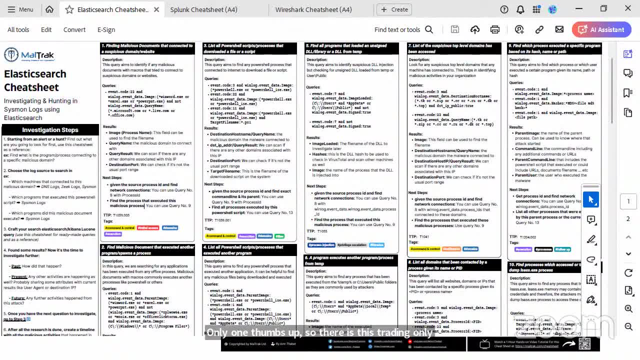 three: are you guys with me? okay, four cool. so this training is well, you know, you guys, most of my trainings were around 1000- 1600. that's mostly how i provide trainings, but i decided that this is a small training, that i'm gonna make it the most. 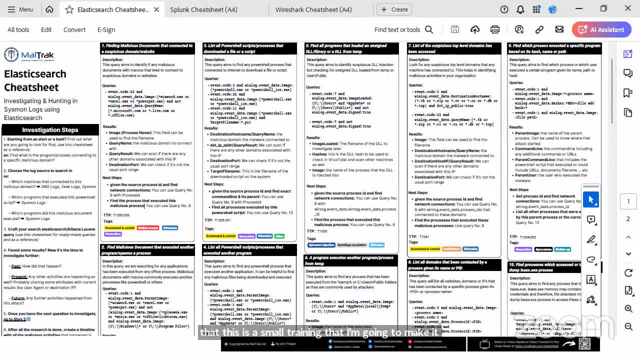 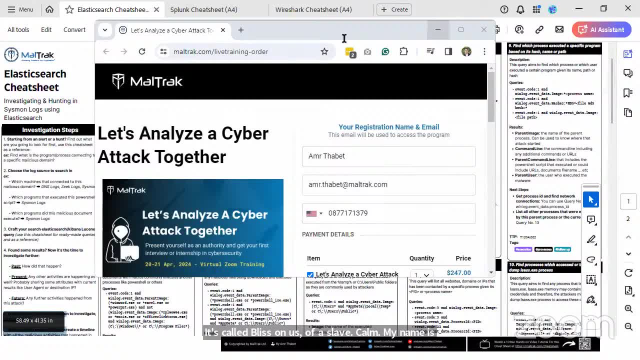 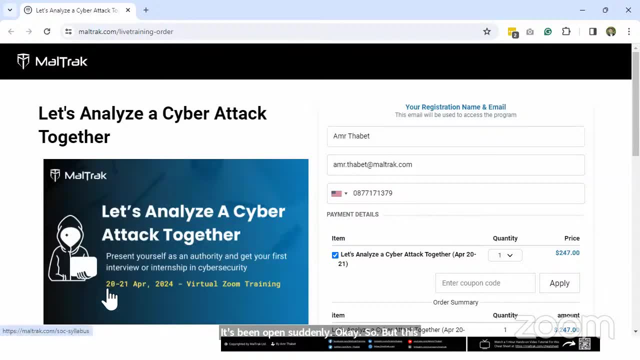 affordable training i have ever done. it's called let's analyze. my name is and i'm the founder of- sorry, that is my youtube channel that's been open. some of it, uh, okay, so this is how it's gonna be. it's gonna be from 2021, of april 2024, and i decided to make it. 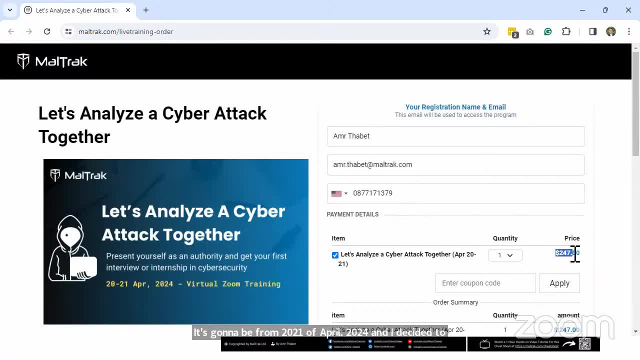 the most affordable training we have and it's gonna be around $247.. like we usually have most of our trainings, it's around, uh, which you guys know- around 997, 1200-1280, 1600, like mostly our trainings in that range. but this training i decided to make it very affordable so we can bring as many people to the event meeting so that it's going to look great from now through course, which is what we're really focused on blending through. so, yes, this training you can. 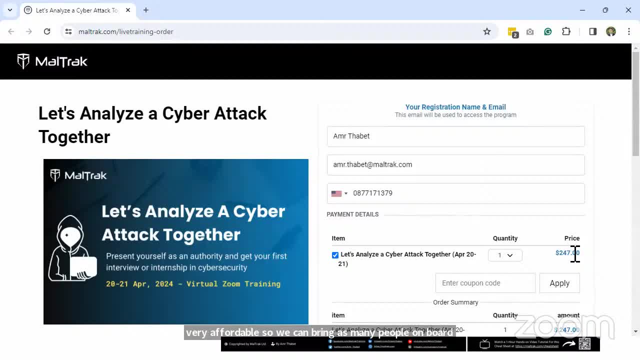 people on board. we can get many people to see how we do analyze the attack, how we actually do our, how our teams looks like and, hopefully, after you learn something out of it, you can basically take that knowledge, maybe applied, get your first job and work with us in your company, or you might. 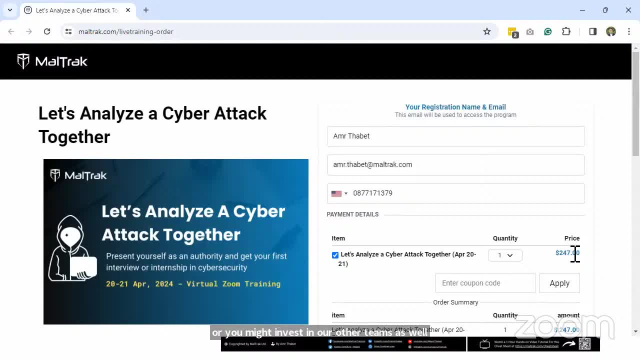 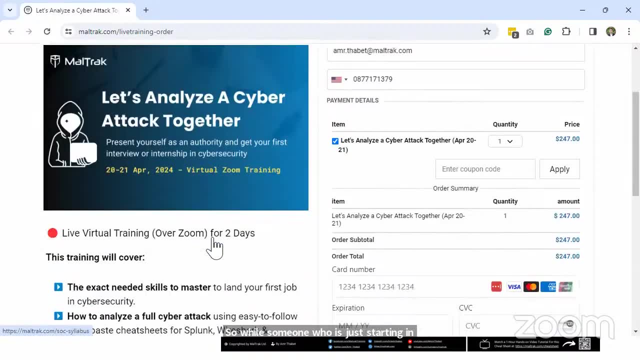 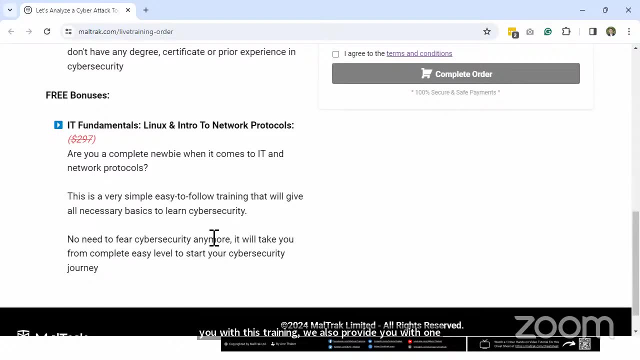 invest in our other trainings as well? um, so will someone who is just starting in cyber security will be able to do this? yes, and not only we provide you with this training, we also provide you with one bonus. if you are new to it and new cyber security, maybe you know just a little bit. 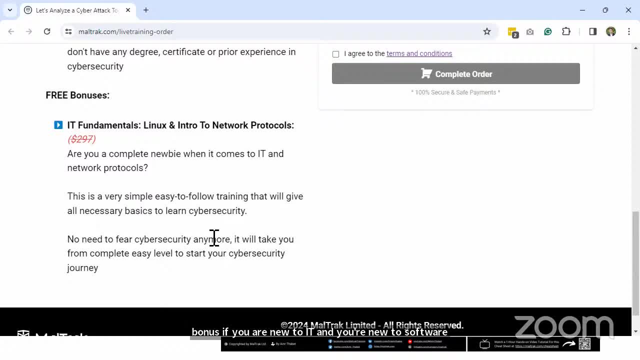 of stuff, not sure that you have the skills. i don't have the the it fundamentals, i'm not really good with networking yet and i don't have ccna and i don't have the network protocols and i don't know all of these protocols. we'll provide you with a bonus. actually, this training is 297 or i think. 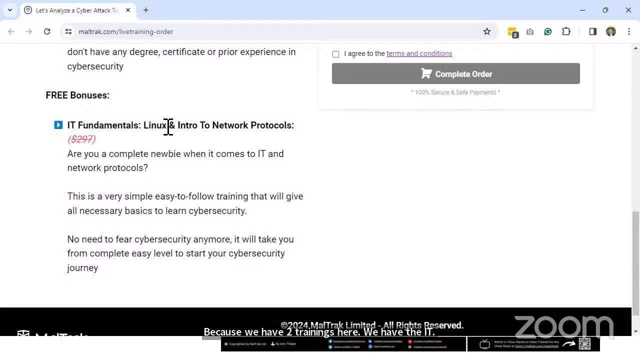 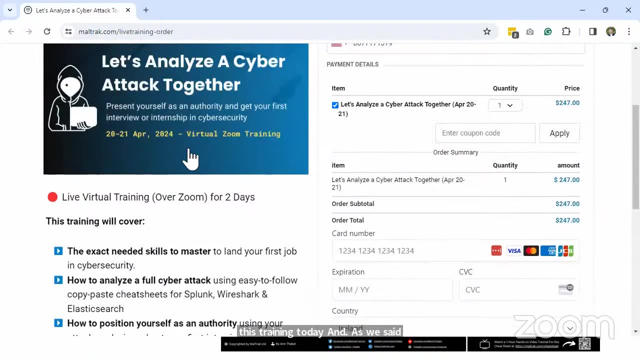 we have the it fundamentals, linux fundamentals and it fundamentals network protocols and you're going to get access to both these trainings as a free bonus once you sign up for this training today. and, as we said, we're going to cover this live training, uh, from um, from 11 am, gmt to 3: 30. 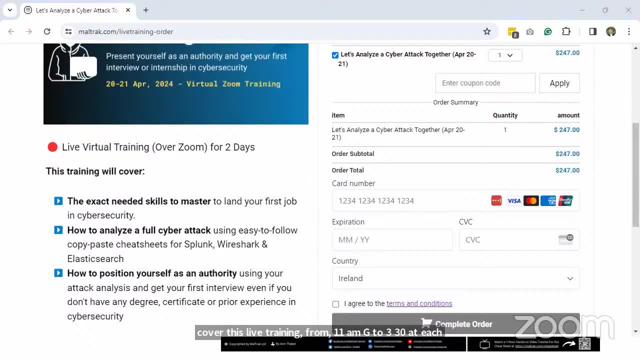 each day, so it's from 11 to 3: 30, 11 am to 3: 30 pm. that's gmt and so it's four hours and four hours and half a day. it's around nine hours. maybe it will be around 10 hours. we're gonna cover the the. it is really the most hands-on. 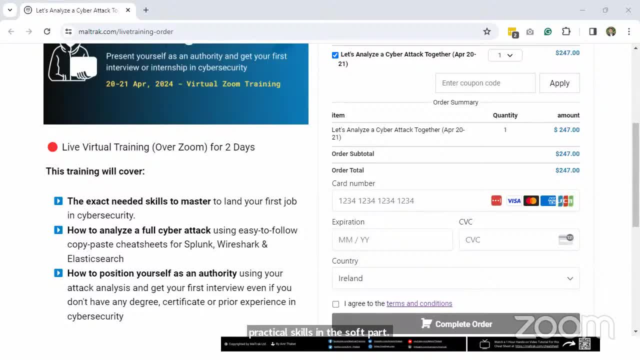 practical skills in the stock part. remember when we talked about learning the, the stock skills, the, the exact needed skills in the market. don't just learn things that are random like how to, how to you know um, use os, fingerprinting and nmap and try to find different- uh, infected machines and all of these different things. you need to learn what. 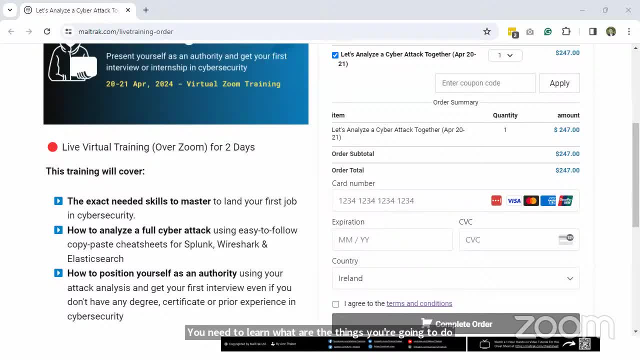 are the the things you're going to do in your day-to-day life as a stock analyst, and this is what we're going to cover in this training: what you're going to do in your um, um, what you're going to do in your day-to-day job in the uh as a stock analyst. what you're going to do it. 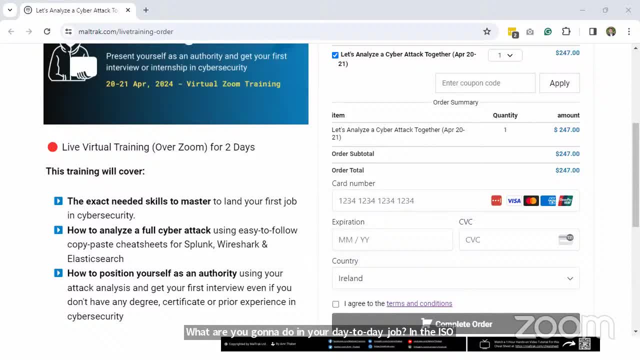 every single, every single day. that's what we're going to cover in the training. you're going to do it with me. so it's not just theory, it's not like ch, where you just go through the training, through a lot of theory, to learn. this is basically going to do it with me. live on zoom. we're going to. 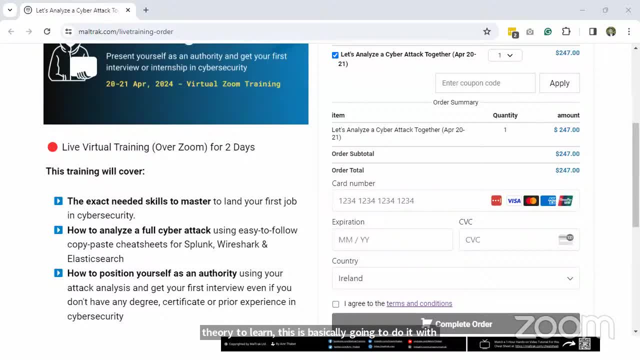 have break rooms. you're going to practice with other people. we have also another coach in will be live with you and he will be working with different, with different people, with different people of you guys, and you're going to help some of you throughout this training and then from all. 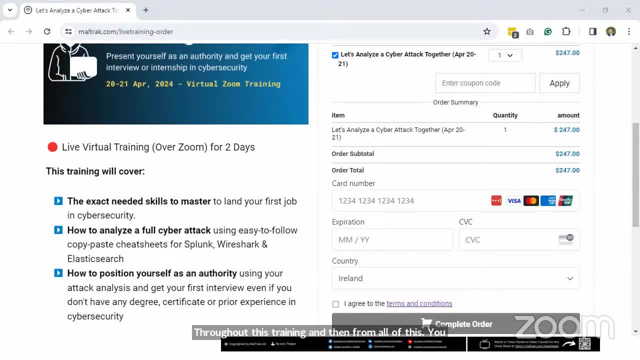 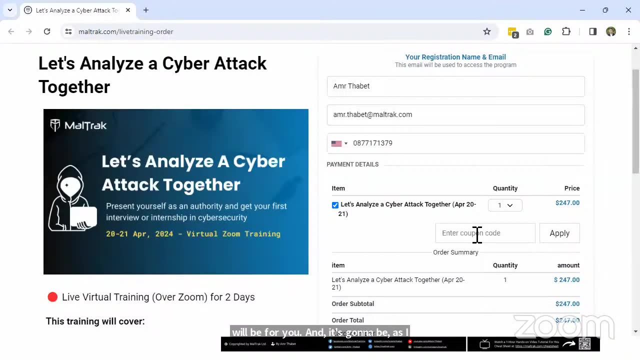 of this. you will be writing your first blog. you're going to share that blog and you're going to have the best training you're looking for. this training will be for you and it's going to be as i said, it's going to be 247. but if you join today, if you join in this, if you join today, we have a coupon called. 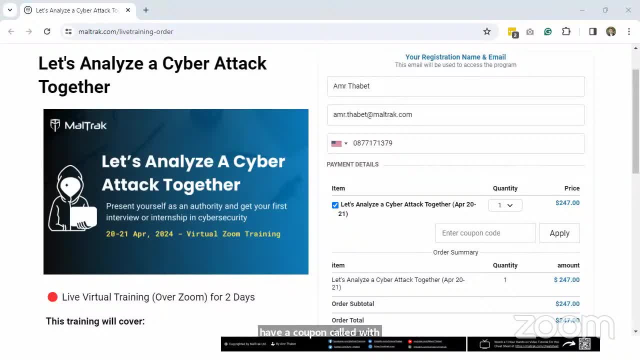 um, let me find the name of the coupon. um, it's called live today. if you use live today and click apply, you're going to have 100 of the price. so if you join now, i'm going to put the link and in the description and the zoom, meeting and as: 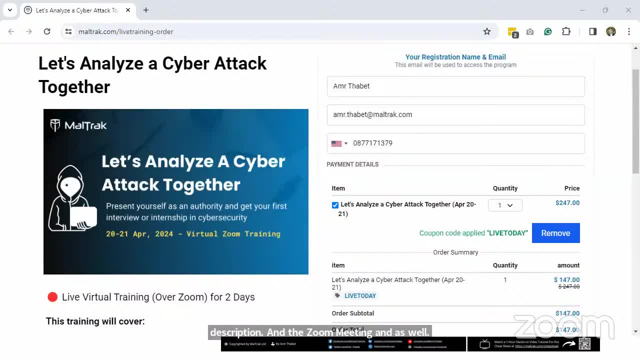 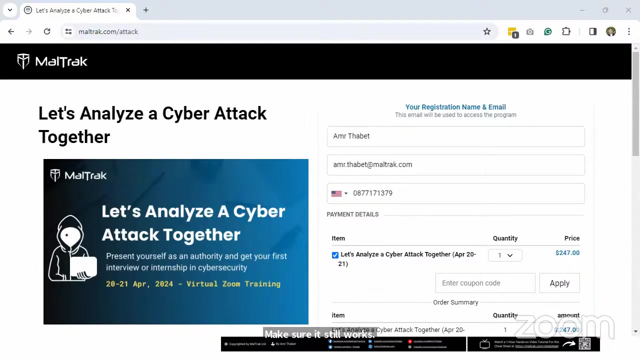 well in different other pages. let me get that link. if you go to make sure it still works, i'm gonna paste it up here and as well in the other, in some of you guys on as well. i will be on youtube, so i'm going to paste it up here and as well in the other, in some of you guys. 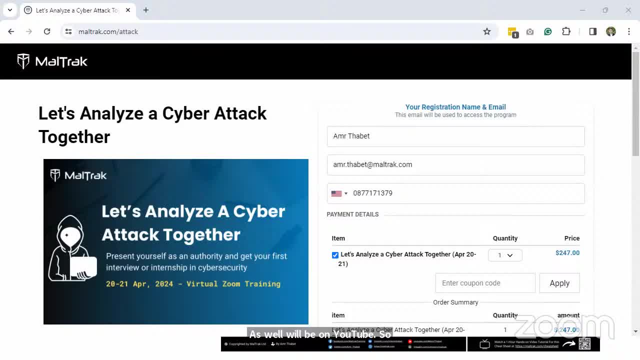 So if you go to maltrakcom slash attack and apply the coupon live today, you're going to get access to this training. It's going to be live next, not this weekend, the next weekend, So you have time, you'll be in the weekend. 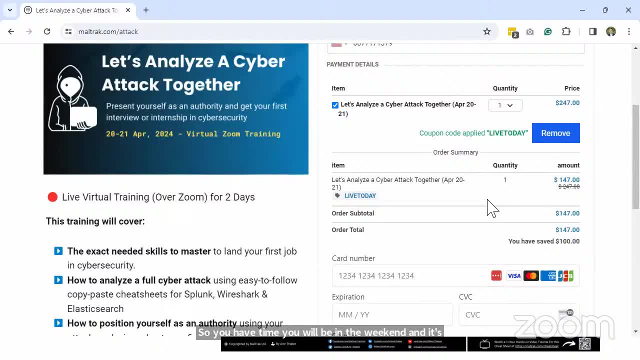 and it's going to be how to analyze a real attack together. It's going to be nine hours training. It's going to be for 147. only Apply the coupon live today. I'm going to paste the coupon. This discount only works for this training. 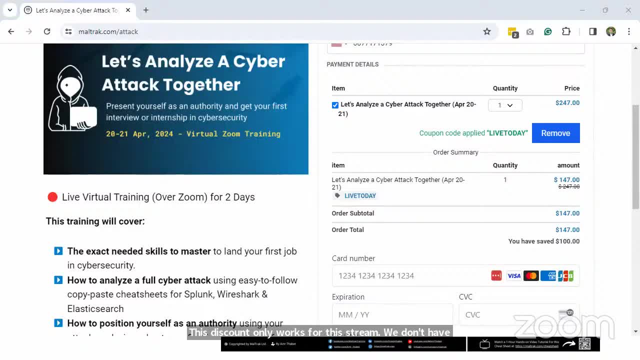 We don't have other discounts of other trainings. We mostly don't do discounts, But for this specific training, for this one training only, we are making it the most affordable ever and we're putting it in the lowest price possible. Guys, any questions you have about the program, about this training? 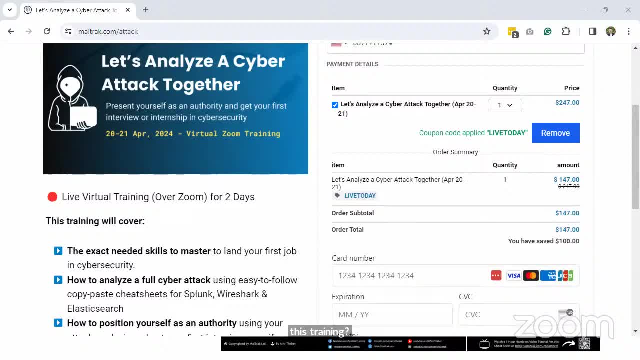 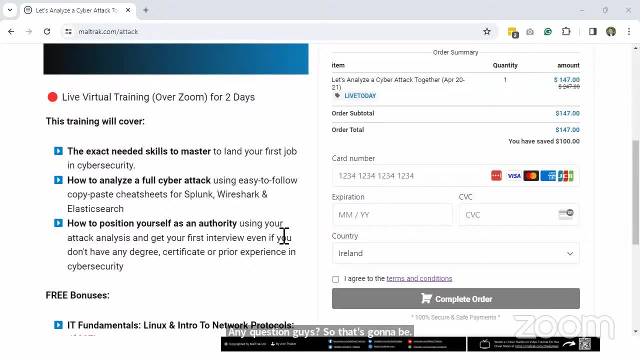 Any questions, guys? So that's going to be like. this is again, we need another discount on other course provided by you. We won't do that. We won't do that now, unfortunately, But this training is really the most like the best bargain you can ever get. 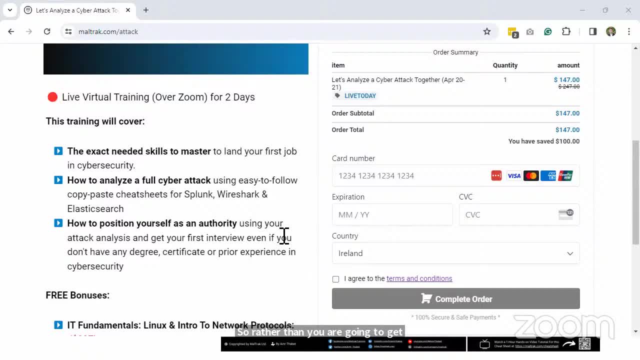 So, rather than you're going to get the $1,000 and the other $2,000, this is the only one that is now the most affordable And the training is really impressive. You will walk away with these cheat sheets that you can use in your own work. 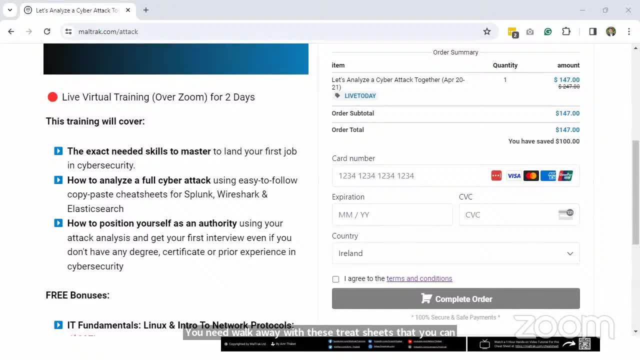 if you are a SOC analyst or for your own blogs where you show yourself as a professional in this field. So, for people who are already registered, we're going to start officially in the 20th of April. You're going to receive an email from me on this Monday. 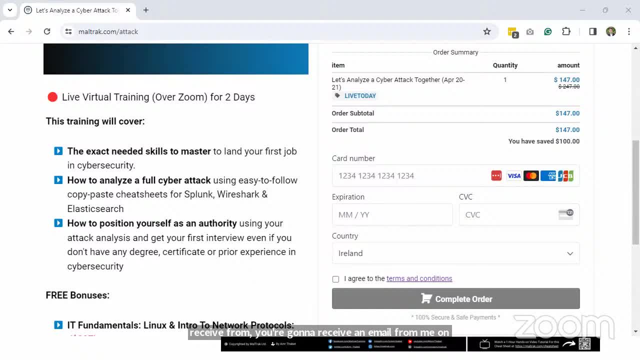 with all the exact prerequisites As well. you're going to access a community where you can work with the other people. So you're already registered. That's perfect. You're going to be able to access that community. We're going to send an email on Monday for everyone who have registered. 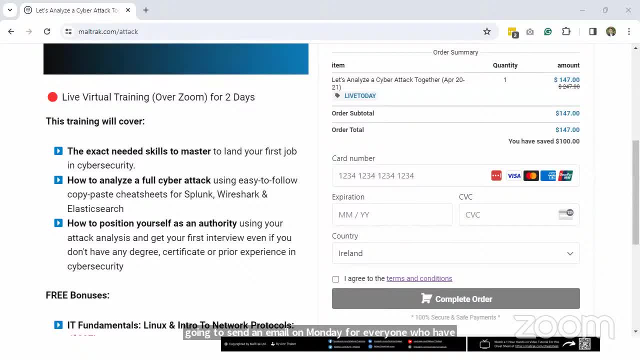 with the exact prerequisites, with everything, If you have already registered. also, you should be accessing the library of trainings you have access to. Do you access the trainings in our training portal? It's going to be added to the master's program. 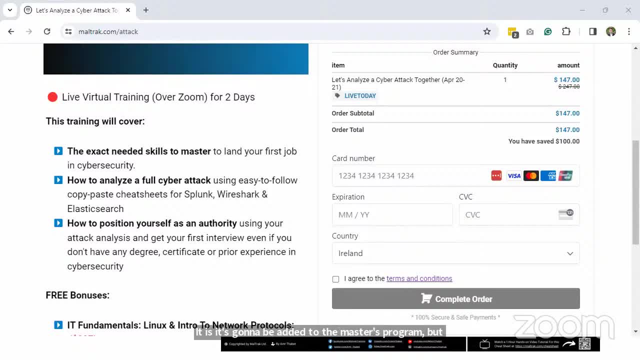 but the master's program is going to be added to the master's program. The master's program has way more in-depth trainings. This is just an intro to what we provide in our training. We really have in-depth coaching and we have live trainings every single month. 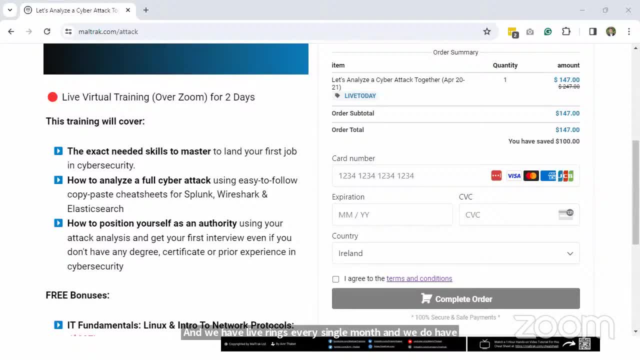 And we do have as well weekly coaching and stuff like that. But hopefully, throughout this training you're going to see the value we provide and you're able to go into the next step. I would say that this is literally the best training you can ever get for that price. 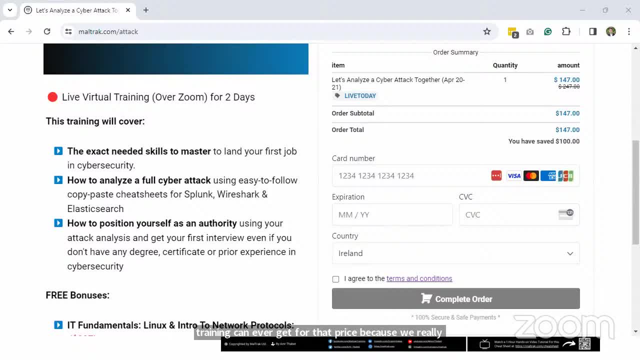 because we really do Really in-depth into analyzing a real attack. You really have someone who is already professional in the market, who's a professional in the industry, and get these trainings and get all his insights, all of his expertise, even his commands. 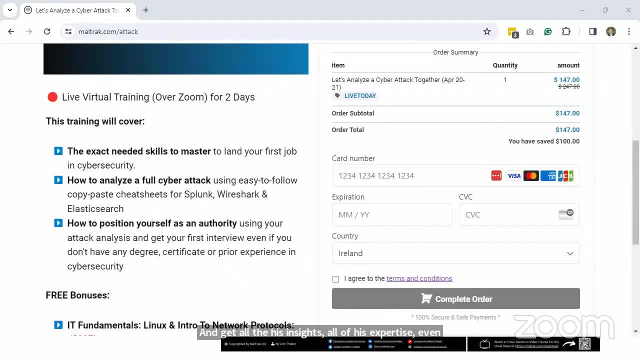 copy paste that you can copy paste in your analysis and get to see, to put yourself in a way that you look like you are really professional in this field for like one, two years, Even if you're still starting up following these cheat sheets, following this, following the, the, the samples on the. 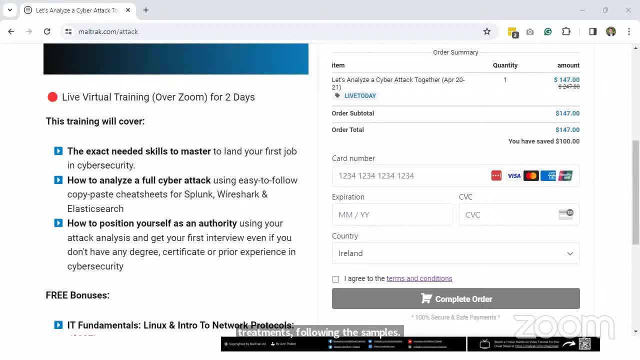 the, uh, the and following my steps. while I'm doing throughout this live training, you can have a blog that shows that you have been two years in that field already And that can already get you into an internship, can get you into an offer. 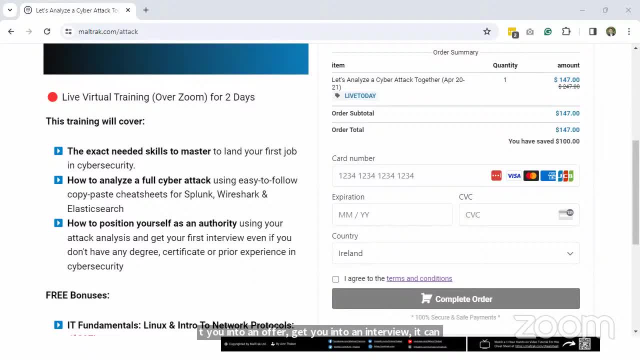 get you into an interview. It can get you somewhere. So if you are starting, this is like a real fast shortcut, because you are really going into that training, You're getting the information really fast. You are also applying this information. You're getting basically all the tools, all the different scripts. 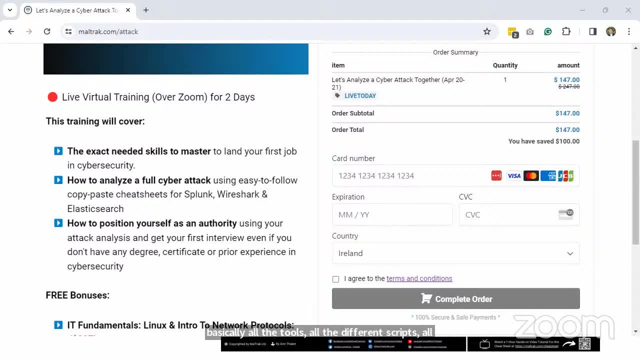 all the different commands, all the process from someone who was already in that field for a long, long time. you are imitating him. You're writing a blog, You are having something that shows your skills and you are presenting that in your own, in your own blog. 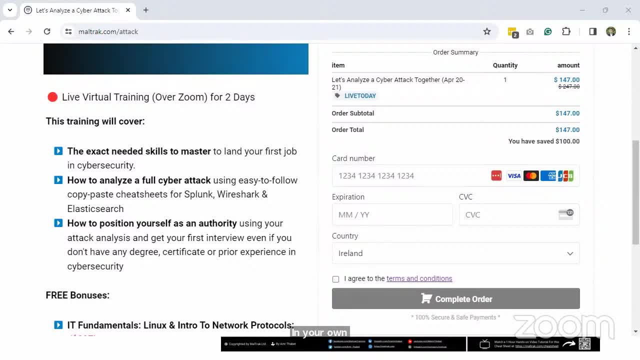 And you already now look like you are. you have been in the field for like one and a half years. You don't need to. you still going to need to learn the actual skills, but you already have passed a big mile by just attending today's training. 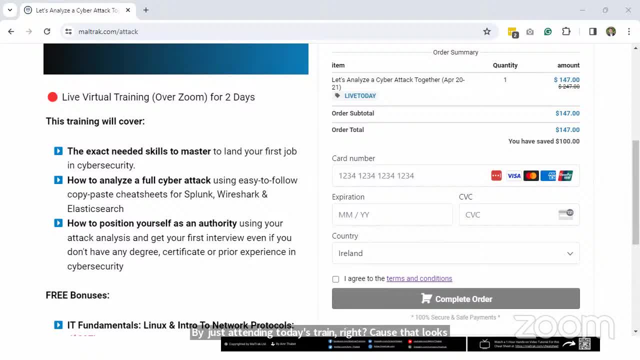 Like. does that mean it's like, it's really for me, if you are starting in SOC, you'd be crazy not to join that Like. it is really the best option for you to be able to to showcase that you have. 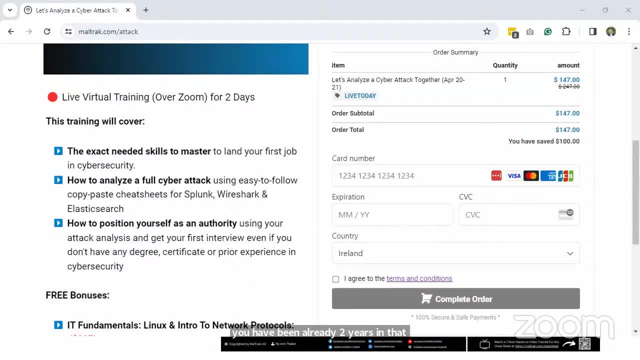 been already two years in that field. Um so so yeah, Um so uh, can we, uh, so we can have to. we have to register today because you have a problem in Egypt to pay in USD, So I need to find a friend to pay for me. 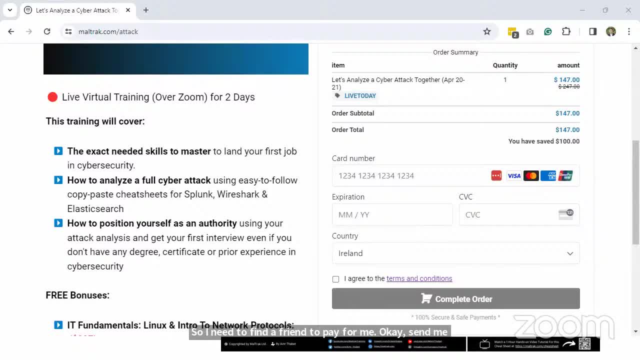 Okay, Send me an email. I'm going to share my email up here as well. Uh, it's support at Montrackcom. Just send me an email If, if you are, if you want to join but you don't know how, okay. 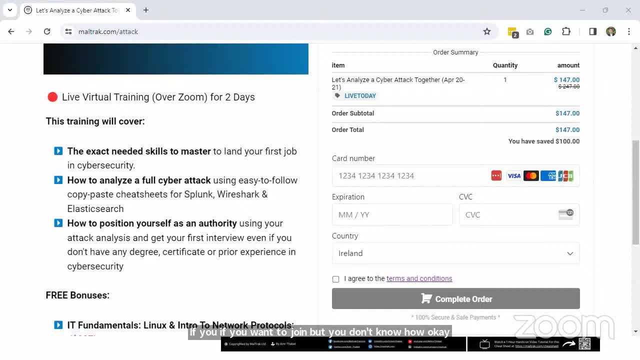 how I can do that now. Can I have it? Can I just join tomorrow, or something like that? Just send me an email If you still want to Have that coupon, If you still want to have that discount. Um, and it's open for today. 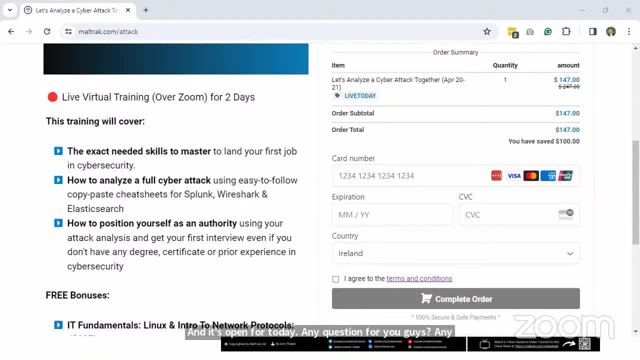 Any question for you guys? any questions? Uh, Mohamed Atif or Mohamed Asif Khan, what the tools we'll be covering in the training? So we will be covering um the first thing we're going to be covering: Splunk. 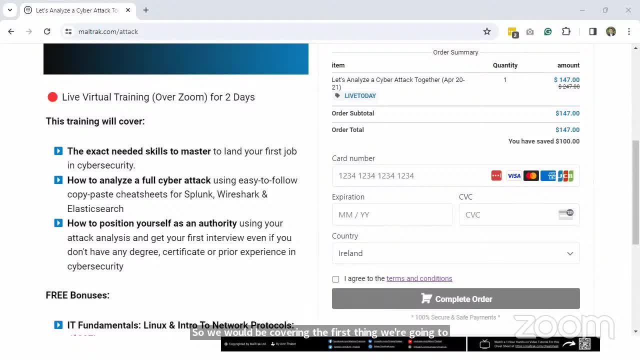 We'll be covering Splunk in depth. SSM- Uh, we'll be covering Wireshark, Zuey. these three tools we'll be covering in depth. but it's not about the tools, It's more about the Logs and about the process. 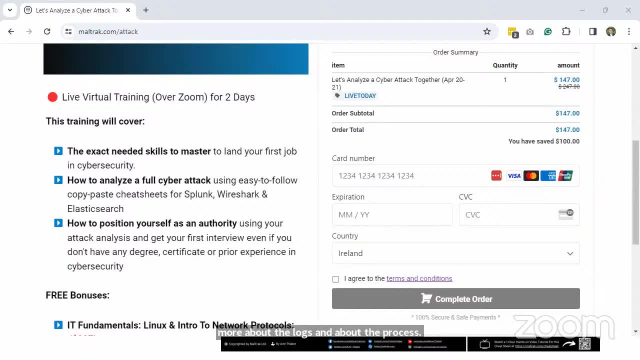 So we're going to cover the incident response process from A to Z. How you can, how you can detect attacks, I can investigate these attacks. I can investigate further and further, How you can write a report that shows you know everything about this attack. 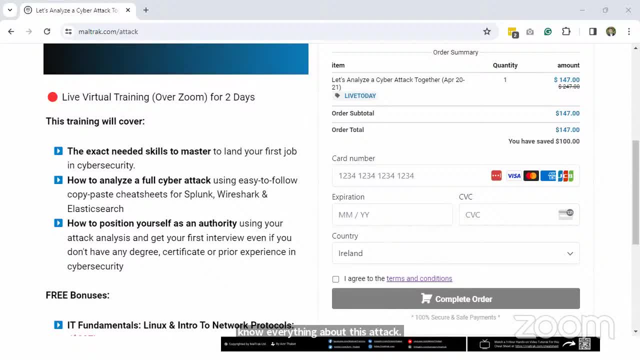 And we're also going to talk about what, if you were in this company? how are you going to isolate this attack? How are you going to contain this attack? All of this different information? Are you going to perform a practical work? uh, ourselves as well. 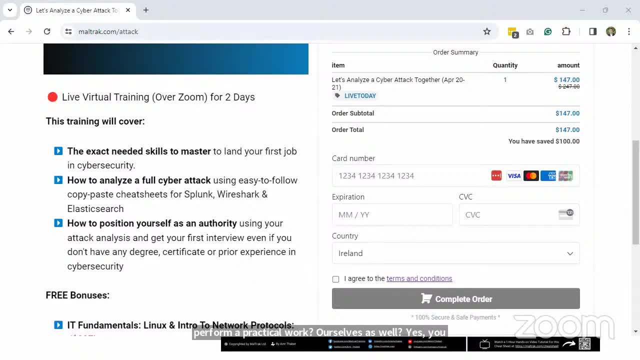 Yes, you will, Or just attend the session. You will be performing The attack. you're going to have the samples, the cheat sheets. You're going to perform the attack. You're going to go into breakout rooms. breakout rooms- hopefully no breakups, uh, breakout. 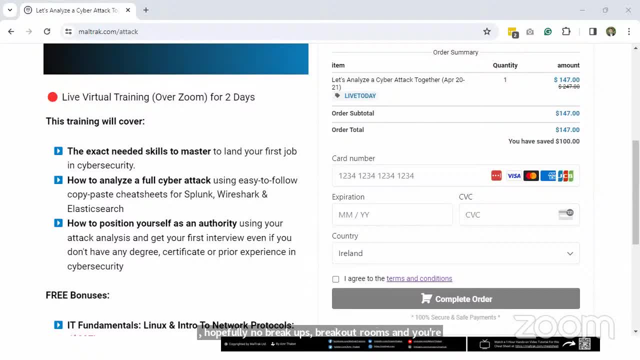 rooms and you're going to perform the attack You're going to share to among other people and as well, me and and uh and another coach as well. We're going to be going through all of you guys and making sure that you are really following. 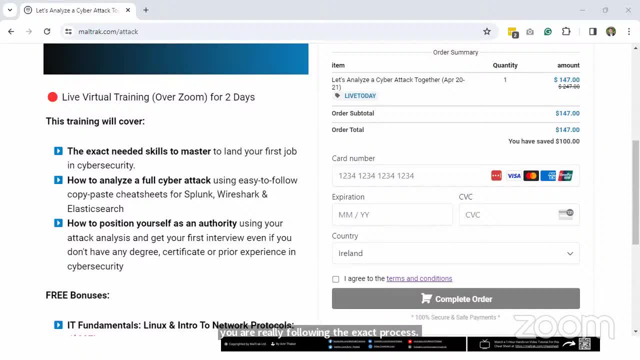 the exact process. Um, uh, so um, or just attend the session and learn from what you're doing or did during today's session. Okay, If we do The hands-on, what are the prerequisites? need to be installed in the system beforehand. 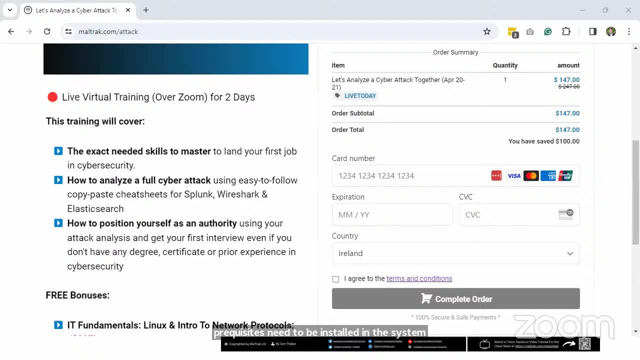 We're going to share with you guys, uh, all of that. Once you you're registered in Monday. we're going to share with you all the exact prerequisites, tools that you need to have installed. Mainly it will be Splunk, Wireshark and Zui. 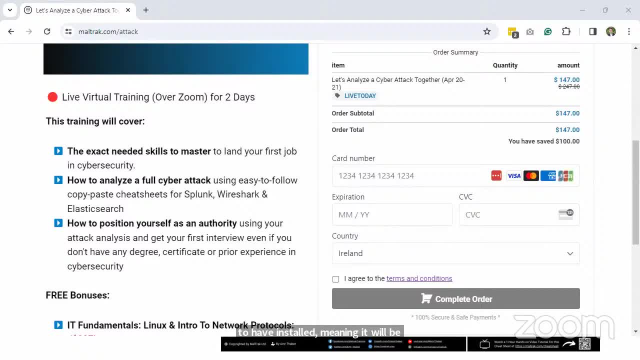 You don't need uh uh virtual machines. uh, just, you know Splunk and uh and Wireshark and Zui. but I will send an email with all these details. Um uh, thank you very much. 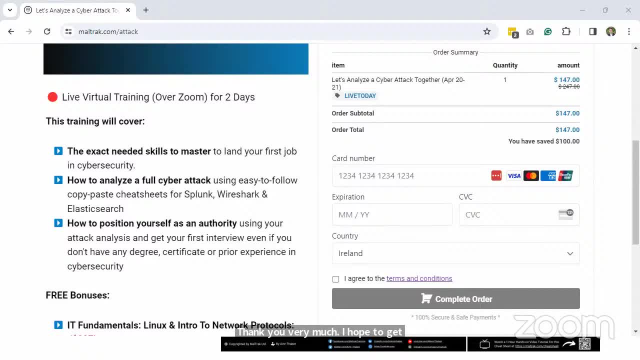 I hope to get better soon too. Um, okay, guys, any other questions? Um, I don't think employers can just look at the lab you have done and then evaluate you. from that can freely land the job offer, since competition is hypercompetitive. 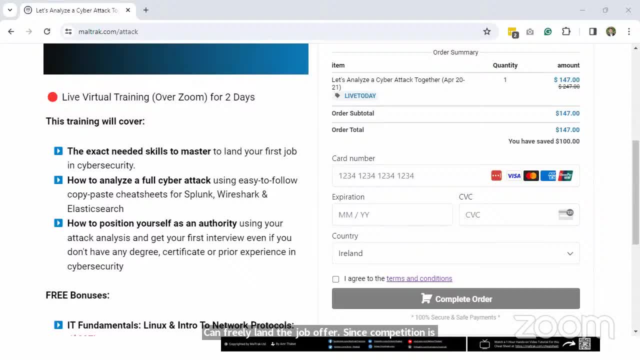 Um, so there's a good question, uh, Nathan, uh, that is on on LinkedIn. So employers will look at your labs and they will look at that as a person worth- uh worth- an interview, And then they're going to interview you and see if you are good enough. 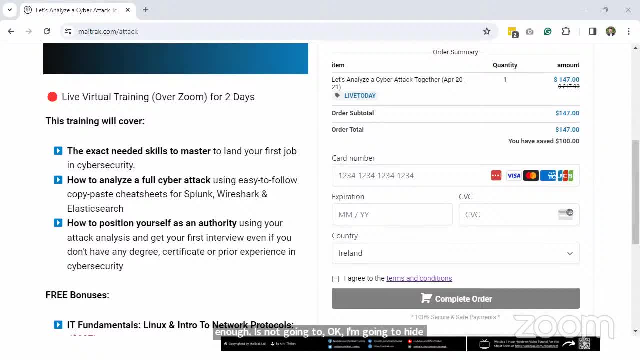 It's not going to. okay, I'm going to hire- I like the lab, I'm going to hire that person. It doesn't work like that. but they will get you into an interview and you say, okay, this person looks like he knows what he's doing. 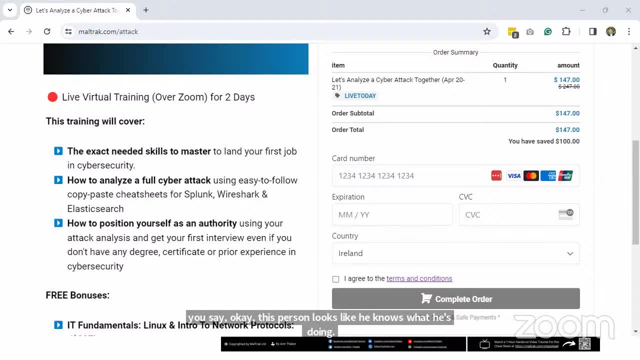 We have, um, a student called Vivek. He was a part of one of our trainings- uh, read, team training- And uh, this read team training. we were developing a backdoor, um, uh, a C++ backdoor. 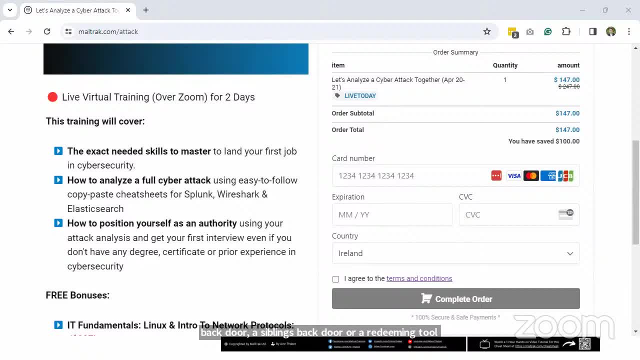 or a read teaming tool. Uh, throughout the whole training he followed the training He did the read team tool. He wrote it in his resume and in his interview on Amazon. they were like that's really amazing. And the the only, the whole interview was questions about these exact projects he has. 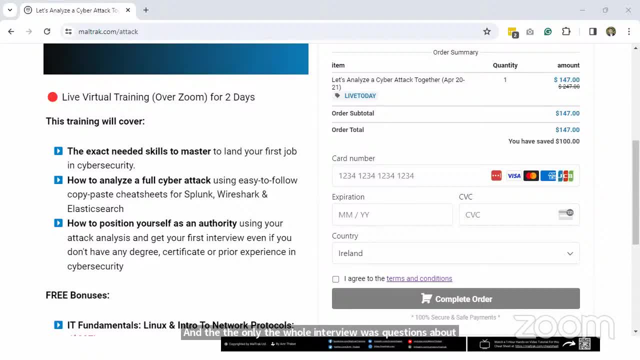 done And he got hired after that in Amazon and AWS as a security engineer, mainly because of just one project in his in his resume that was really attracting the art. I also had interviews with Amazon where I had one One project I have done that. I spent one day in it. really it was like kind of uh in a way. 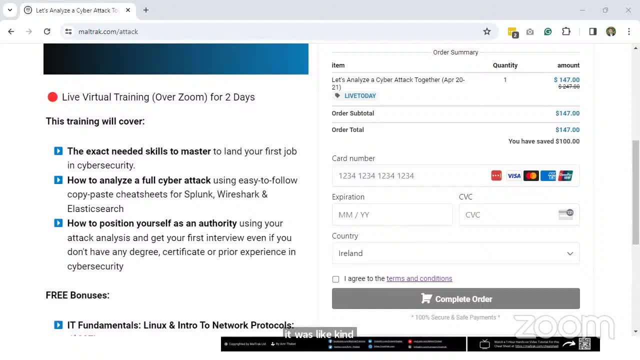 innovation day in my work I did a small project and then I wrote it in my resume and my whole interview was about how, how amazing the idea of this project is And, uh, and he asked me all day, all the interviews, asking me questions about that. 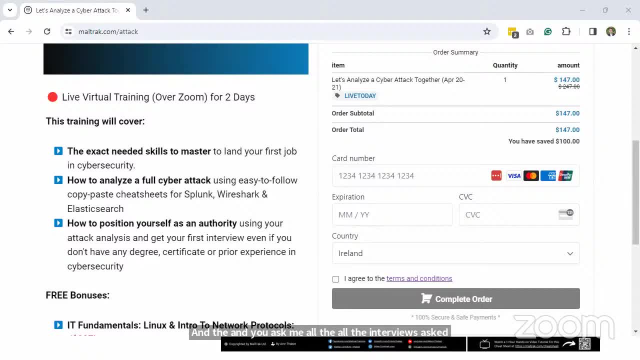 And because of that I was able to go to the next step in the interview and that went from there. So does it really allow get you a job? No, Not exactly, but it gets you way ahead in the interview. probably not only gets you. 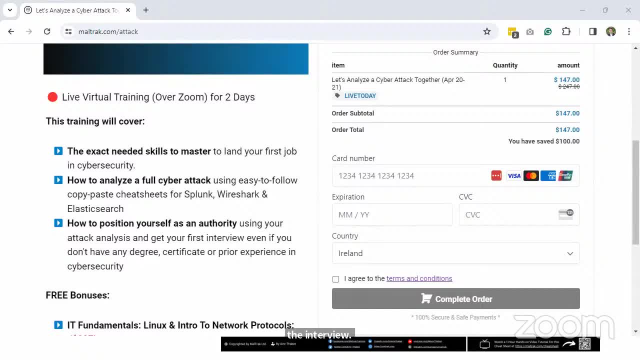 to the first interview, but probably the second or the third one, just because you have something that you are. you proved your skills through it. He's going to ask you a lot about that project, but he's going to be really impressed and 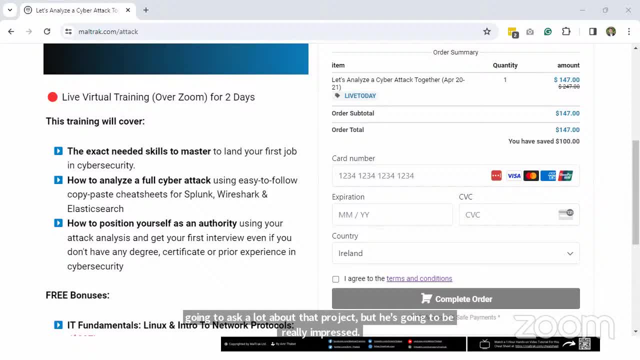 you're going to really look into. okay, maybe we can test that person further. The main, main, important goal for any hiring manager is that you have um, um, that you have the skillset To do your day-to-day job. 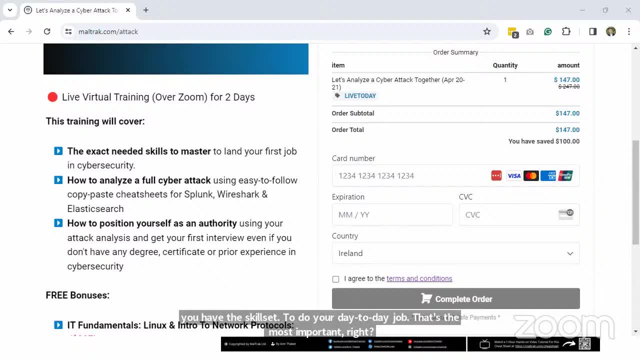 That's the most important right. If you do have the skillset, it doesn't really matter if you are uh, if you have degree, if you have certifications, whatever the story is, it doesn't matter. Do you want you to be plugged into a team and do your job? 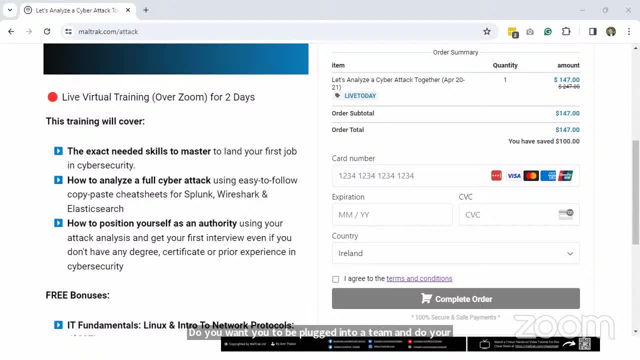 That's it. So if you're not doing though, then there's going to be another. uh, if you're not really in the level to do your job, then they don't want to hire you. So how you can prove that you are? 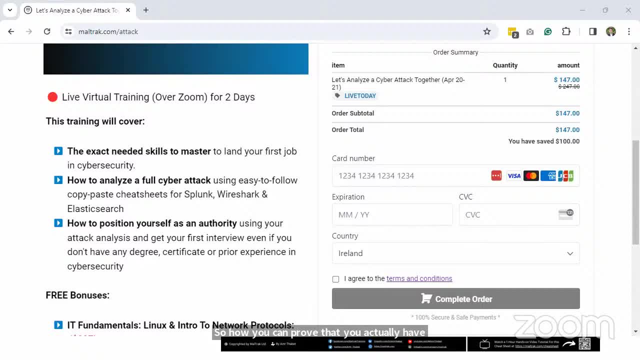 Actually have the skills to do your day-to-day job is to do what you're going to do in your day-to-day job and post it in a blog and say: I have done that, I know how to do that. Can I get a job now? 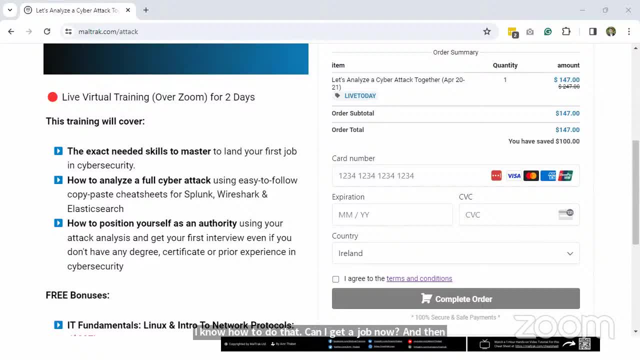 And then they will give you more chances and they're going to give you into, they're going to be more, more than happy to hire you. Does that make sense to you guys? And that's what we try to do in that training. 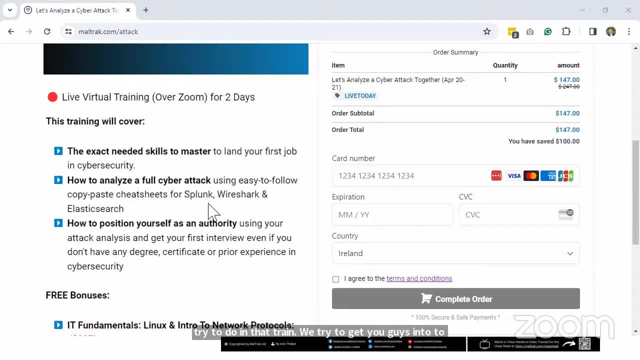 We try to get you guys into to do something that you're going to do in your day-to-day job and write a blog about it. Showcase it. Just you know how to do what you're doing And from there hopefully you can get your first interview, maybe an internship. 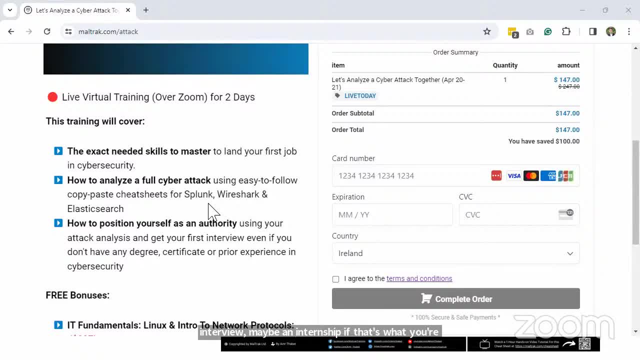 If you, if that's what you're looking for, and maybe even a real job offer, Does that make sense for you guys? Thanks guys, Absolutely Welcome. Any last questions before I go? Any last questions YouTube guys. I know YouTube guys are. you're a bit slower. 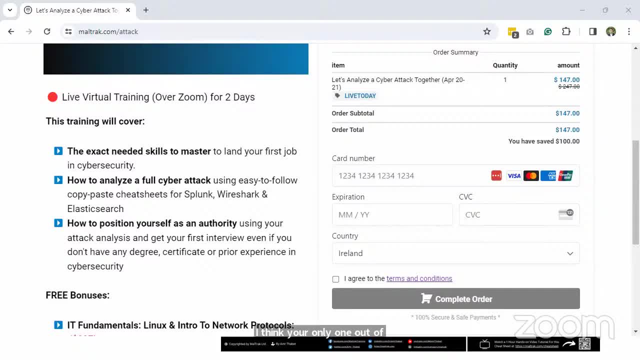 I think you're only one out of 1000 applicants in the backdoor way. Is this a backdoor way to get the job? I think there's only one job out of 1000 applicants. Yeah, I I, if I understand your question correctly. this is really the best way to be in a kind. 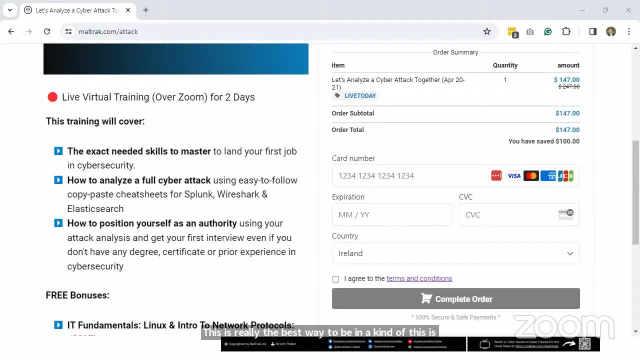 of this is really the backdoor, Really, Yeah. So I think the best way to help the hiring managers is to have a project that proves your skills and you- maybe you can reach directly to the hiring managers- showcase that you look, I have done these projects. 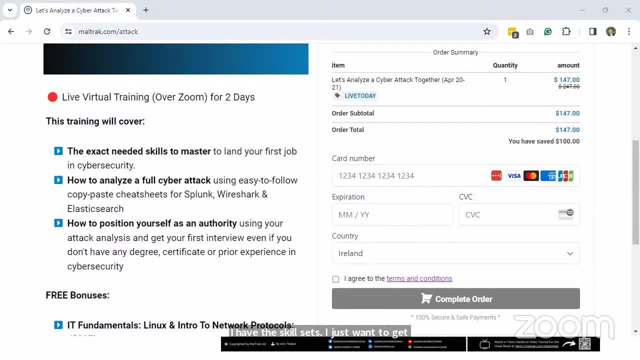 I know what I am, what I'm doing, I have the skillsets. I just want to get a chance in an interview And from there, once you are in an interview, this is where you prove your skillsets And and you'll be surprised. 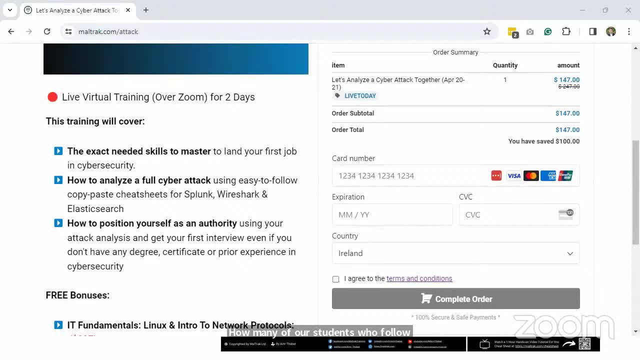 How many of our students who follow this exact same process- and we helped them through it- it they don't even apply for jobs. they the recruiters and the hiring managers they are reaching them out to to hire them in the different jobs. you would be surprised how many cases it. 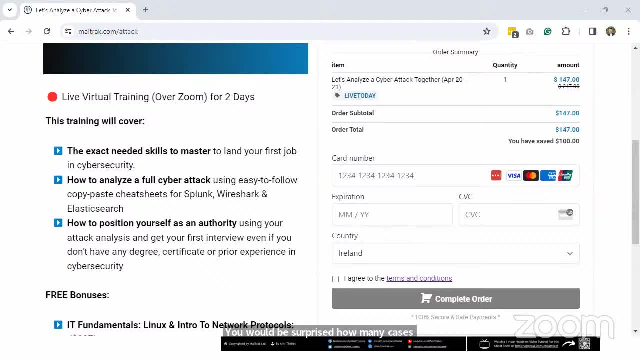 happens like that. you think that, oh, we apply so many different jobs and they don't even look at our, our resume. they are actually searching on linkedin and they are sending- uh, sending- requests to people to apply for the jobs because they think that their profile is really good. you would be. 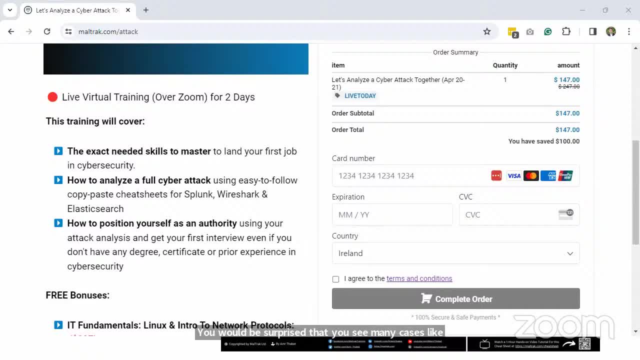 surprised that you see many cases like that is happening in the cyber security realm- from the manager himself that he applied for the job. that's what happened with me with microsoft. the manager who's applying, or who i'm applying for, a job for, or supposed to work under, uh in his team he was. 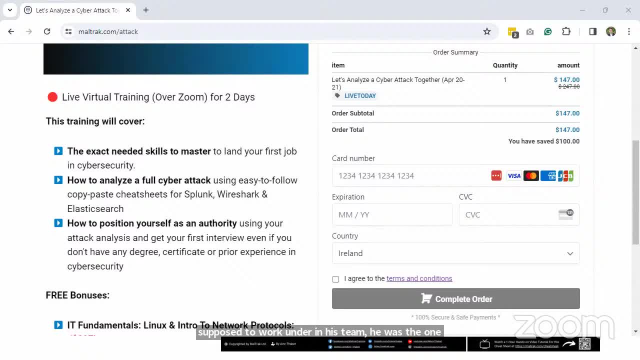 the one reached me out for linkedin, and that happened with kaspersky as well. there was actually someone who reached out to me to apply for this kaspersky job and so on. so it is basically you, the hiring managers, the recruiters, who are reaching out to people trying to find people. 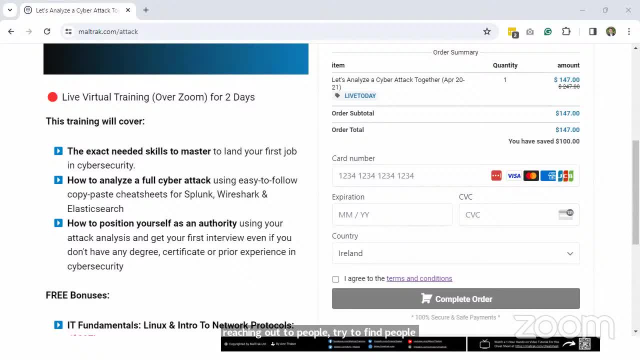 and this is the best way you can showcase your skills. does that make sense for you guys? thumbs up still make sense. i know 20 of you are still alive with me. thank you guys for being here. any other question, guys? okay, if there's no questions, guys, this is your chance. go to maltrakcom slash attack today this. 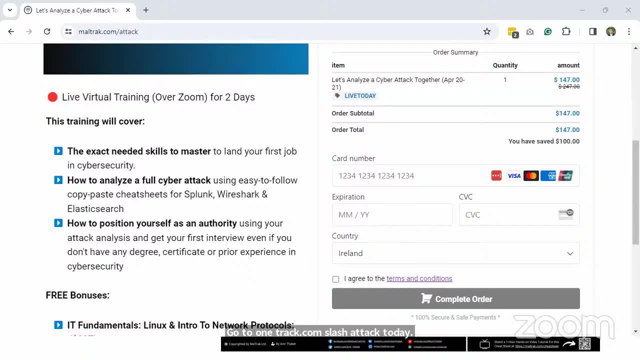 is literally the most affordable and the most the the like. this training will really make a massive difference in your career. this is really the shortcut. this is the backdoor, as this guy is saying. this is the backdoor to get ahead like, as you are already two years at the field, not only. 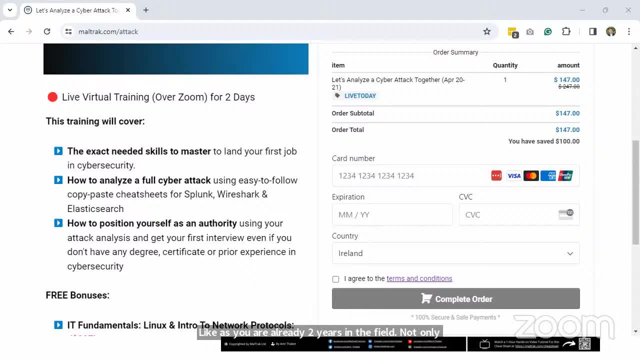 you're going to learn the skill, the exact skills, for the job, but you're also going to learn the skills that you're going to use in your sock job, the exact tools you're going to use. but also you'll be able to show that i i know how to use this stuff and using the cheat sheets, using also our bonuses. 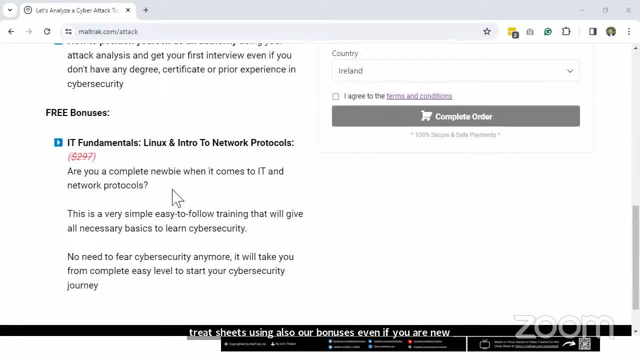 even if you are new to the field, using that bonus training. this is going to be a free training that you're going to get access to in once you join. that's going to be an immediate access. once you join, you're going to get all of this. uh, you're going to get all of this. different cheat sheets.